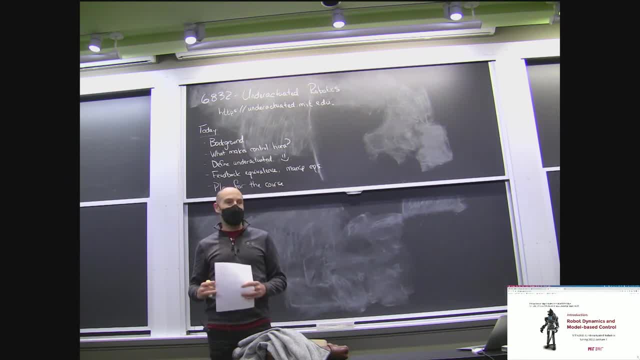 some of the very best sort of control we know how to do in robotics. Now reinforcement learning is coming into play and producing similar. I'll show some highlights, Maybe some of my favorite examples. and the world is in. I think the world of controls is in like a beautiful place. 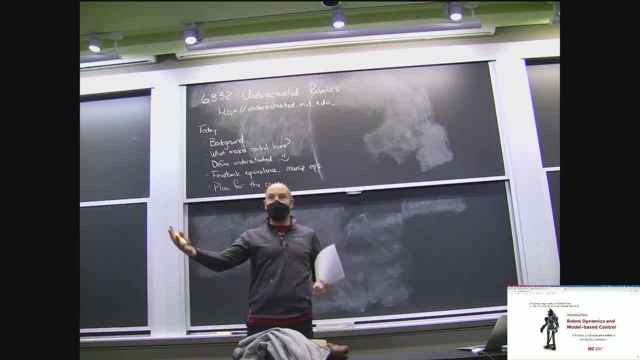 where some of the exciting work that's happened in empirical reinforcement learning is blending with some of the work from theoretical reinforcement learning and machine learning and rigorous controls. okay, Now there's a couple different classes that are all sort of relevant to that at MIT. 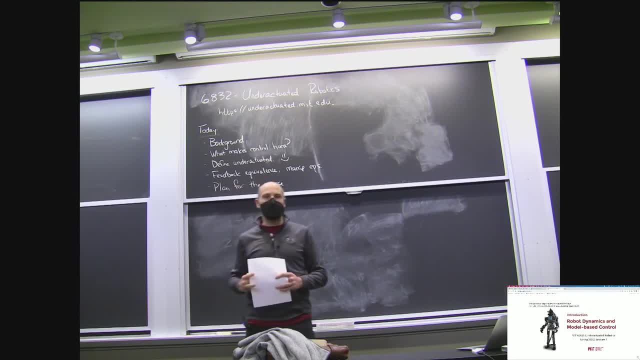 Nowadays we have reinforcement learning class and dynamic programming class. that will stand alone And cover the reinforcement learning side of it a little bit more. But even the theory of reinforcement learning is increasingly leaning back on the theory of controls. right, These things really do go well together. 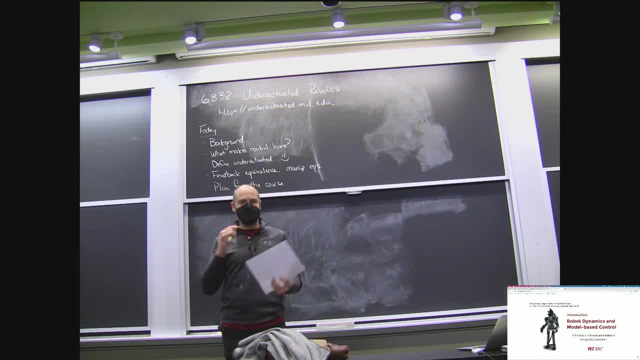 So what I want to do, what I think I can contribute most to your quest to understand these things, is to tell you how you know how those different technologies interplay, And I'm going to try to take you through the steps of sort of understanding dynamics. 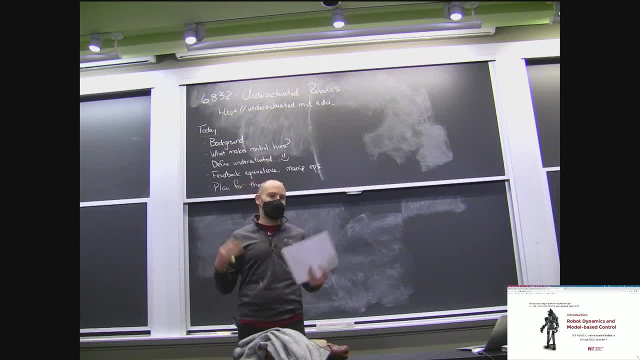 Nonlinear dynamics. There's beautiful ways that people talk about mechanics and understand nonlinear dynamics. when you care about nonlinear dynamics, If you know what a dimensionless coordinate is, you're on your way. If you know what a Poincaré map is, you're on your way. 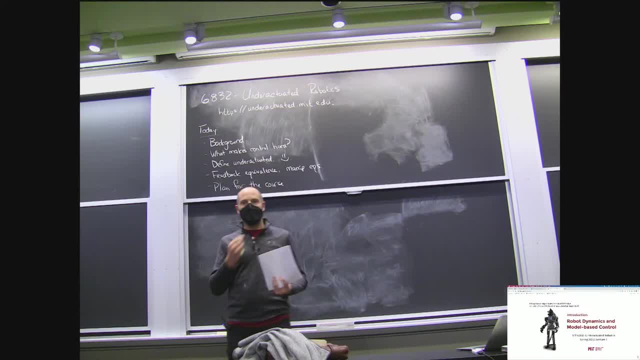 There's some beautiful concepts from nonlinear dynamics. There's some beautiful concepts from controls that will remain relevant even if, you know, even if we have big data. I think understanding the algorithms is going to use the tools of control, And then we're going to bring them all together and see where reinforcement, learning and control meet. 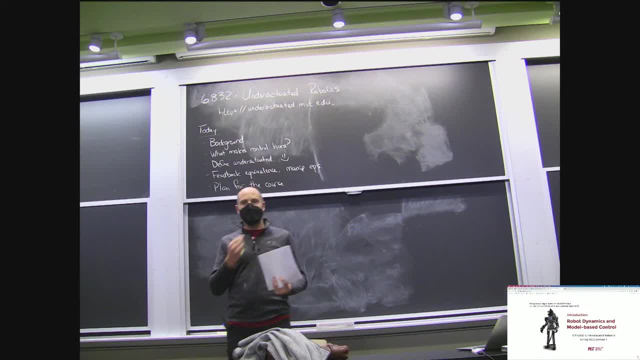 So I'll go a little bit out of order here, But let's talk a little bit about what makes control hard. Okay, So there's a classic picture that you see in sort of the beginning of any reinforcement learning talk and in the on the cover of a lot of controls texts. 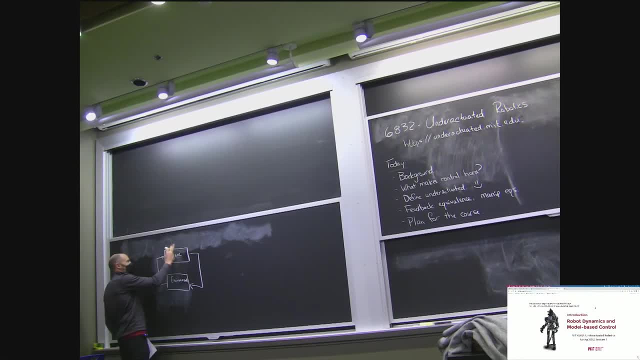 Well then, a feedback loop right. The control Controls people you know, so the agent might also be called a policy right, or your controller. The environment, in our case, is going to be a robot. It's going to be Atlas or some other awesome robot plus the you know. 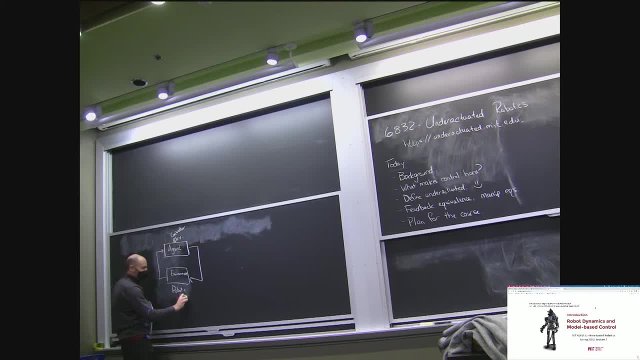 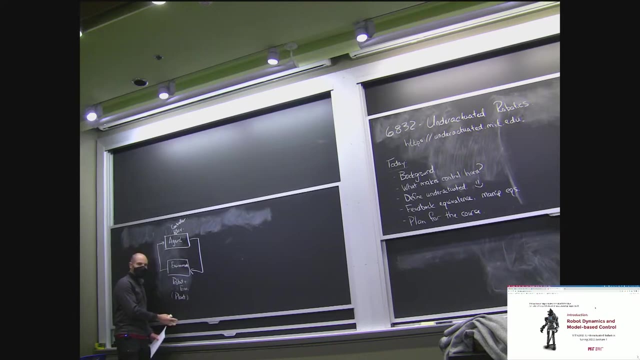 anything in the world plus any physical objects in the world, Okay, And we might also call it the plant pretty regularly. That's a whole thing, A holdover from chemical engineering contributing a lot to to the beginnings of control, And we we still call the thing we're trying to control, the plant often. 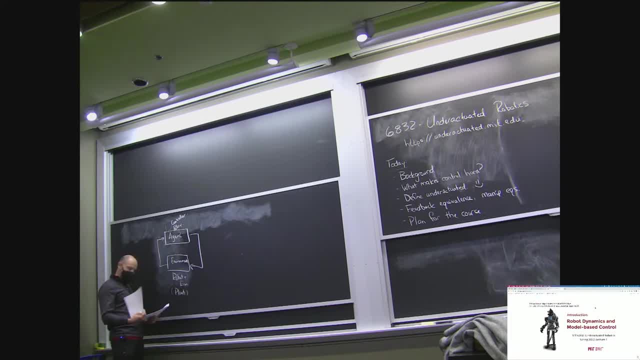 Okay, Okay. So there's lots of different versions of this problem. You can just think about this. you know, as like I want a single algorithm that can work for any environment. But we're going to try to sort of look under the hood here and make specific, have a specific understanding of particular models of environments and robots where we can sort of, you know, understand more deeply what's going on under the hood and how you should be designing your, your agent. 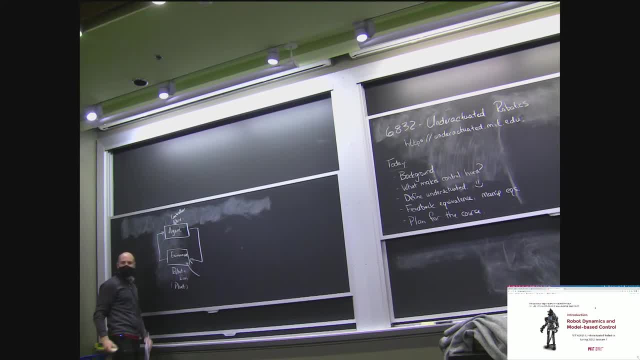 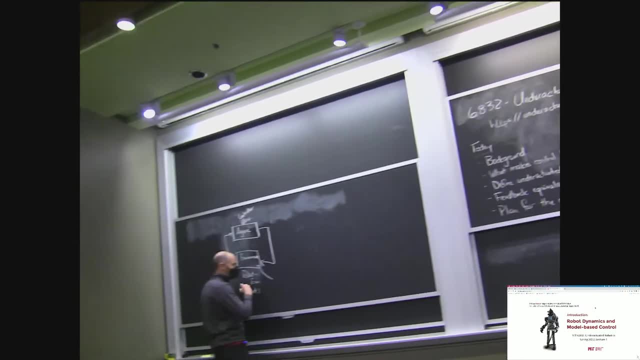 Okay, So in particular, we're going to be doing a lot of work to understand, you know, to to write our environments in the language of differential equations and dynamical systems. So we'll often model this if it's a continuous time. 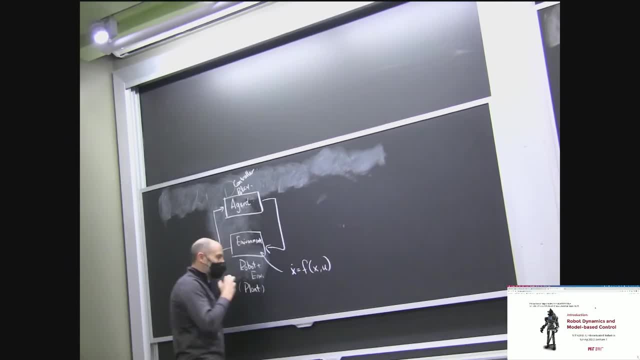 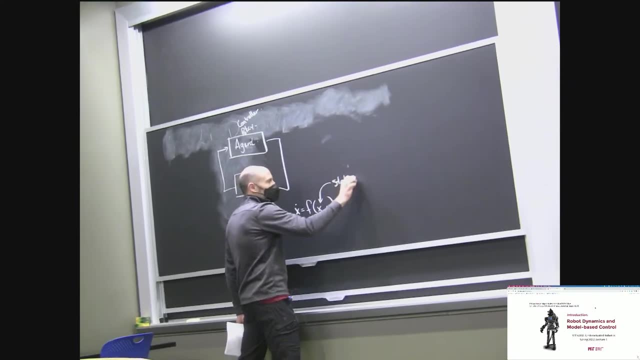 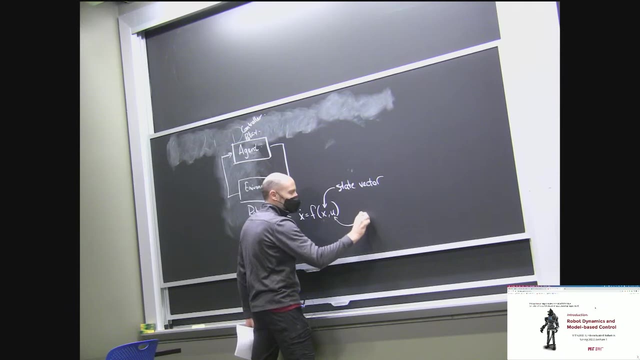 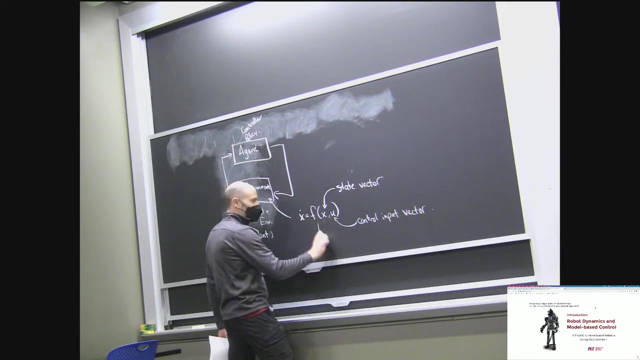 Continuous time system. we'll model it in the language of a of a different differential equation, where this is a state vector, So it's a, you know, a vector notation here. This is my control input vector, which makes this a vector-valued function. 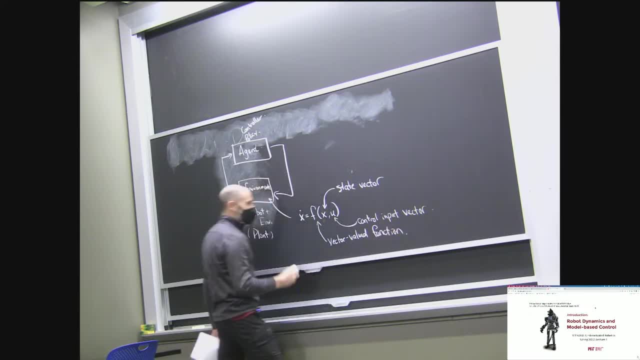 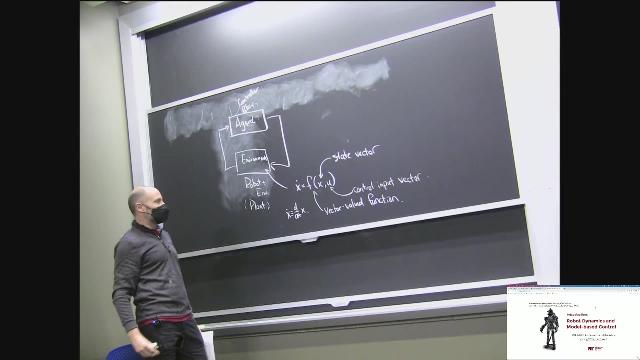 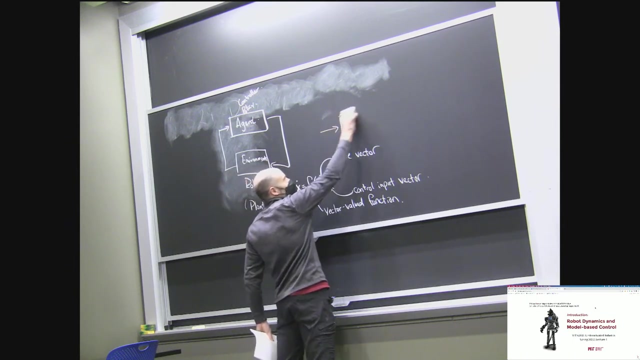 And just to make sure I've defined everything properly, that's always: the dot just means the derivative of, of x, the time derivative of x. Okay, So this is my standard fare for, you know, modeling these environments. And then I also, if I want to model the output. so if I, if I were to just rewrite that over here: right, I've got my. I'll call it a plant this time. 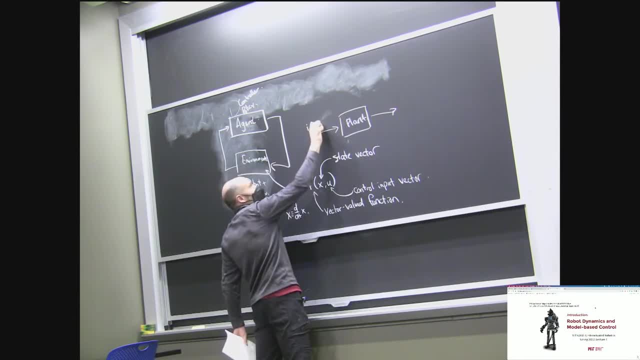 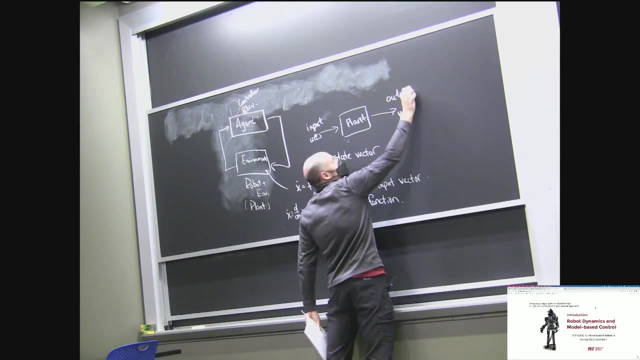 To give equal coverage. I've got my inputs here. we call those u in the language of signals and systems. I'll think of that as a continuous time u coming in, I often use the notation y for my outputs And then the dynamics inside here that govern the, the evolution, are: x dot equals f of x u. 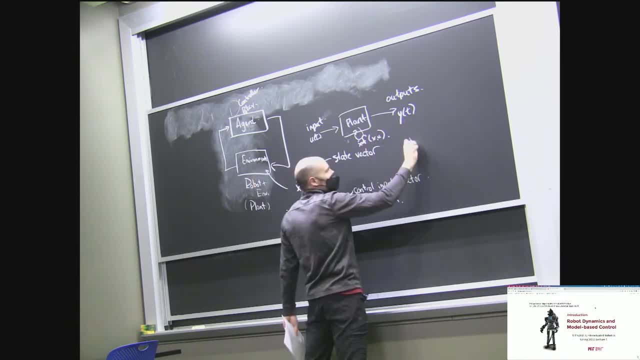 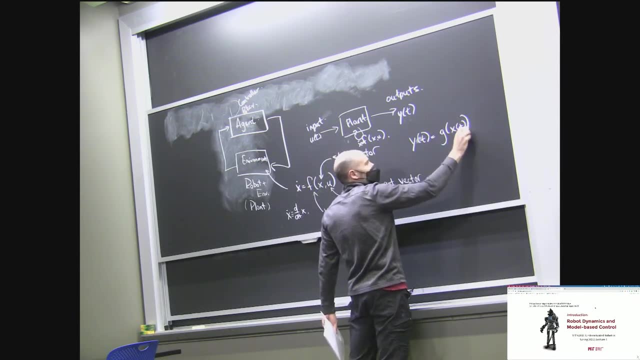 And I need something else to tell me how y is generated. So I also have a Some output function. I'll keep it simple for now. just say it's a simple function of the current x. Okay, So examples of inputs and outputs. 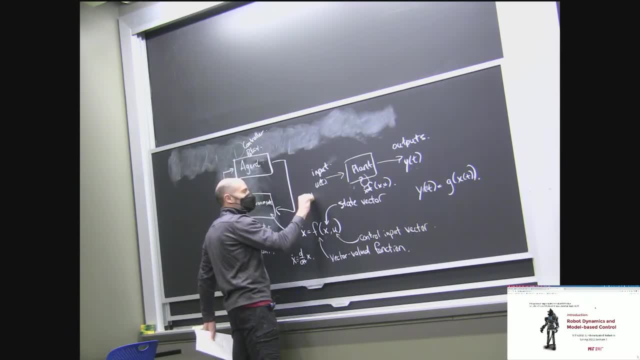 These might be the motor commands. over here I'm controlling a humanoid robot. Maybe it's the. you know, it's actually the, the voltages I send to my, or the, maybe the torque commands that I send to the to each actuator that I've on my robot. 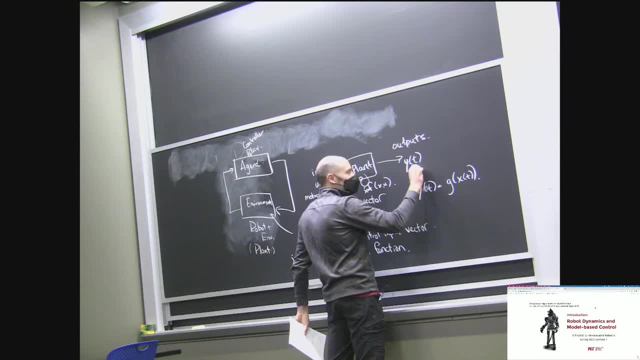 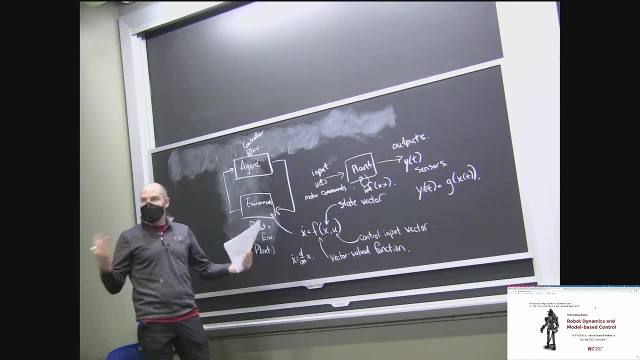 Okay, Y is a is a big vector of my robot sensors. Everything that I can measure from the world is what I've able to give back out of the plant to my control. okay, Okay, and x in the middle is: is a sufficient representation of what's going on in the world so that I can simulate it, for instance, 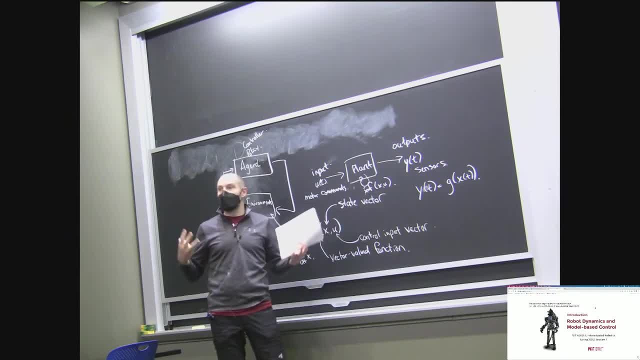 So the case of a robot is, for instance, the positions and the velocities of the robots. So what we're going to do is climb to the four corners. here At the top there's 2 still goes to the second square. 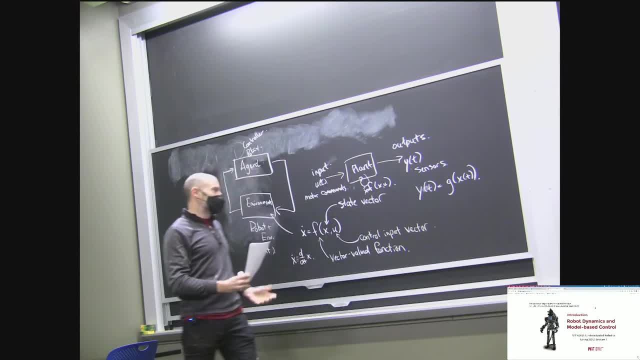 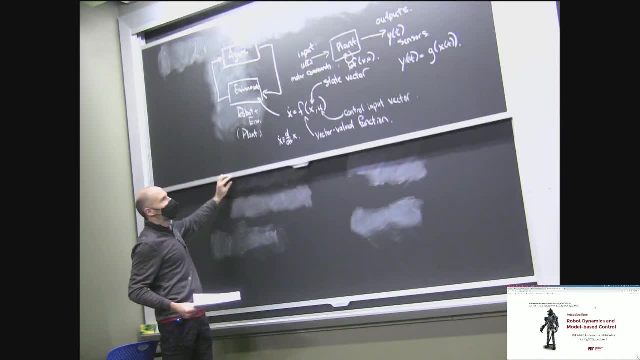 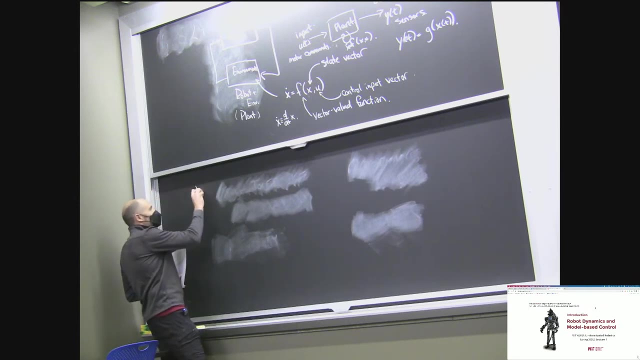 but and all of the objects in the environment would be sufficient. So that's a very general view of the control problem And I want to sort of ask what makes control hard? Or decision making- really, You could put any sort of, you know. 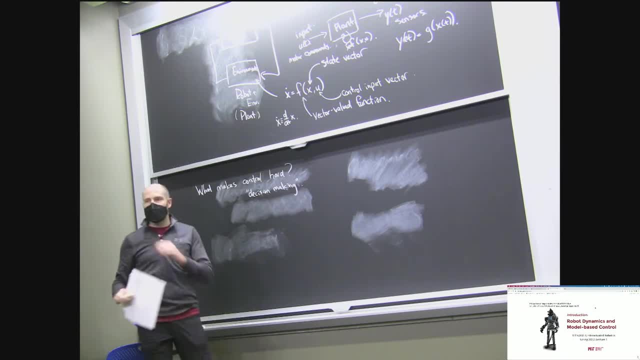 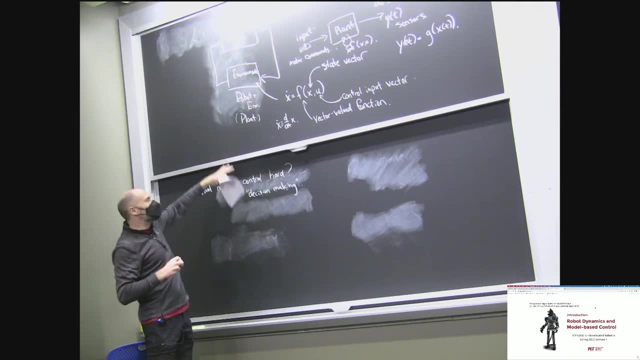 you can say playing Go should fit in this framework also, You can have easier hard control objectives. But let's say I want to make as a working example, I want to make Atlas, a humanoid robot built by Boston Dynamics, do a backflip. 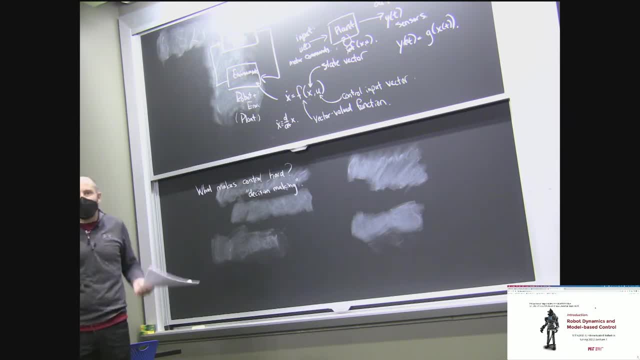 Is that a hard control problem? And why right Is playing Go with a computer a hard- you know- decision making problem, Or why, And you know, there are a couple other canonical examples. So what are some of the things that come to mind for you guys? 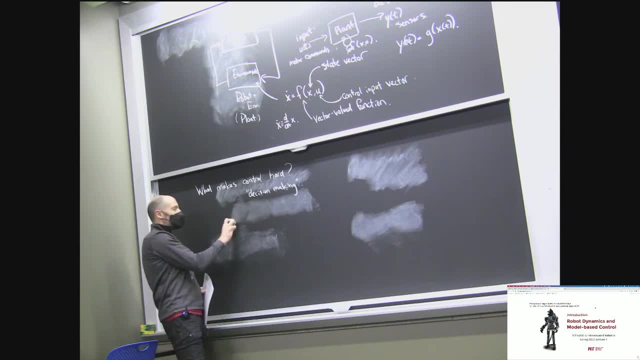 I know that some of you know the language well. What are some of the reasons why control could be hard? Yeah, Stability, Stability. OK, Humanoid robots tend to fall down And we don't want that. Yeah, Large number to the degree of the freedom. 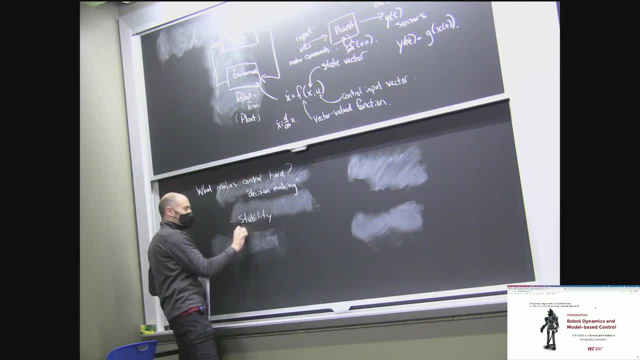 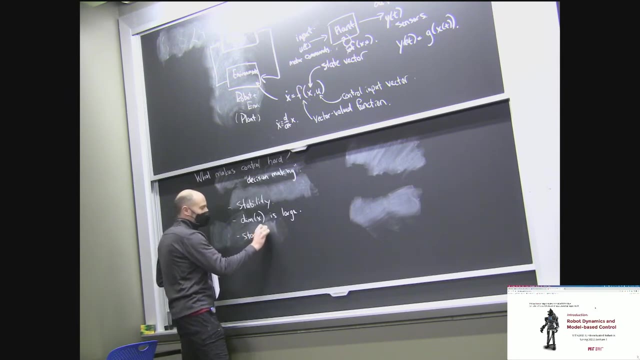 OK. So if x is very large, for instance, What else? Yeah, Stochasticity, OK, Good, Stochasticity. What did I do? Stochasticity, Yeah, Yeah, Yeah, Yes. Partial observability: Yes. 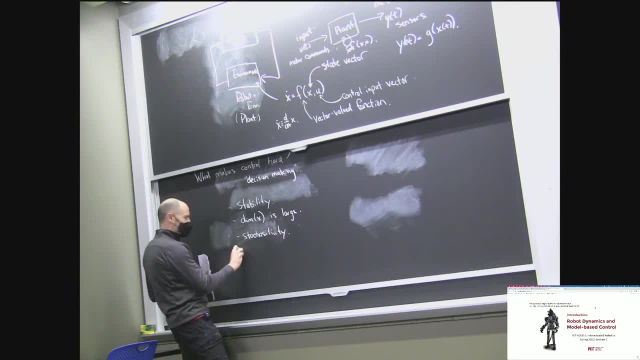 Good. So that's- maybe I almost wrote that along with this one, But it's, I think, deserves its own line. Partial observability. Any other big ones, Yeah. Coupled input. Coupled input- What do you mean by that? 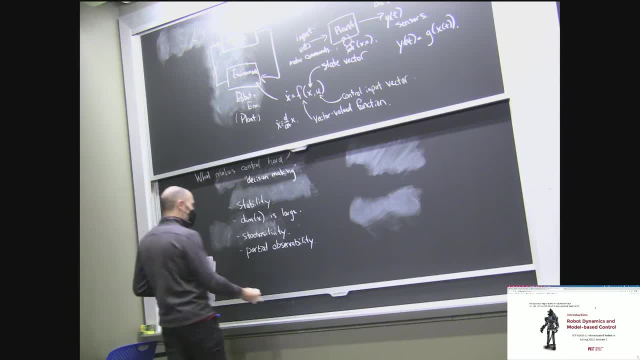 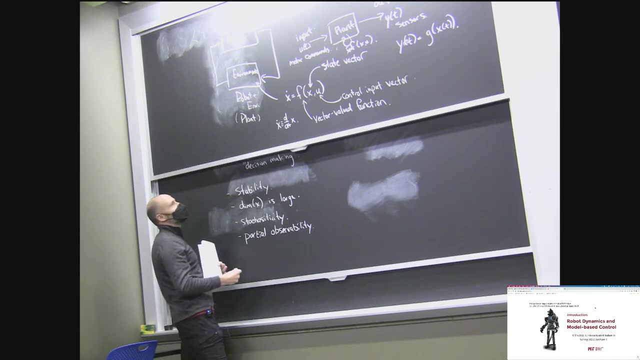 So like one input changes more than one input. OK, So it could be really just, Maybe just more generally, to say that if f is some complex relation, so if the way u enters f is a complicated function, that's a good list. 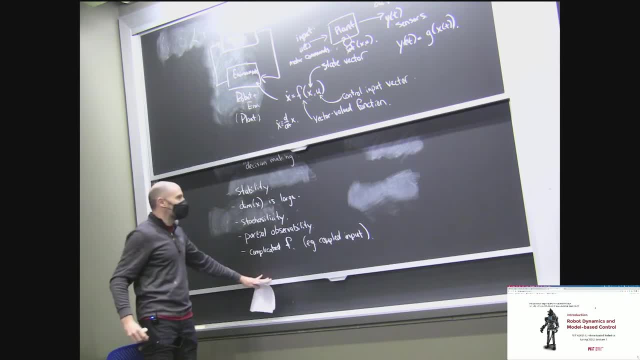 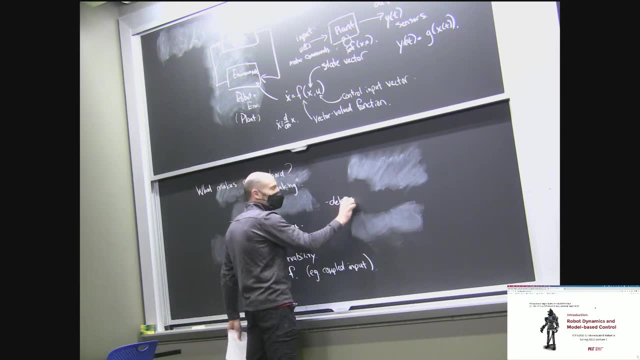 So let me add a couple others that I think people will often say. So let me add a couple others that I think people will often say: Delayed reward in the RL sense, which is, I think, synonymous with having the consequences of your control. 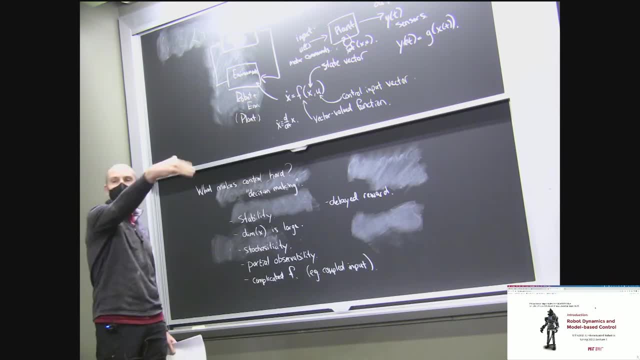 actions at time 0,, for instance, have an effect far into the future. You could have it come through the cost function or you could have it come through your dynamics. But if your decision now takes time to take impact, right Yeah. 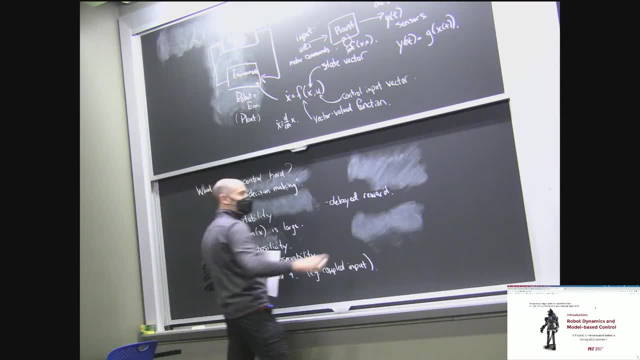 You could have an impact than this. long-term dynamics, That's a big one. So the game of Go, for instance, is not challenging. for partial observability reasons, You can look at the board in Go and immediately see everything there is to know about the board. 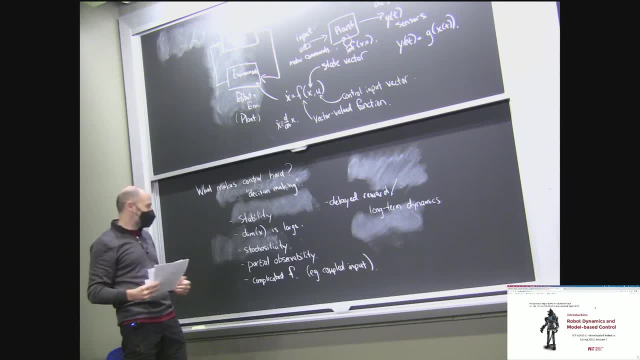 Maybe you can't see in the other play, but you can at least see the state of the board. But you have to think really far ahead potentially, or have a strategy that implicitly thinks far ahead, in order to win. There's no stability issues or other things. 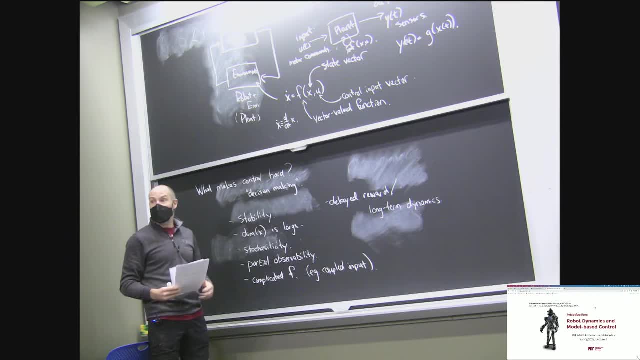 but a lot of different problems have a lot of these different aspects. So you can guess where I'm going with this. How does underactuated fit into this? I mean, I'm going to define underactuated for you. but given this backdrop, 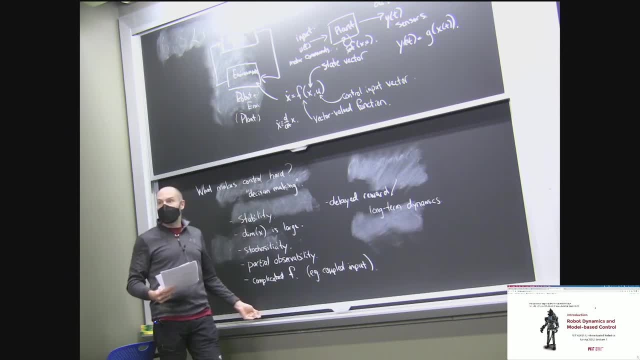 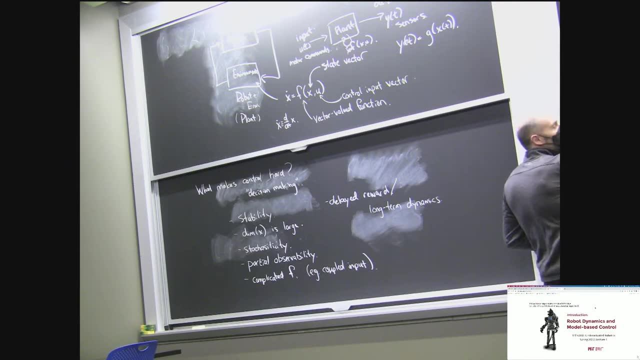 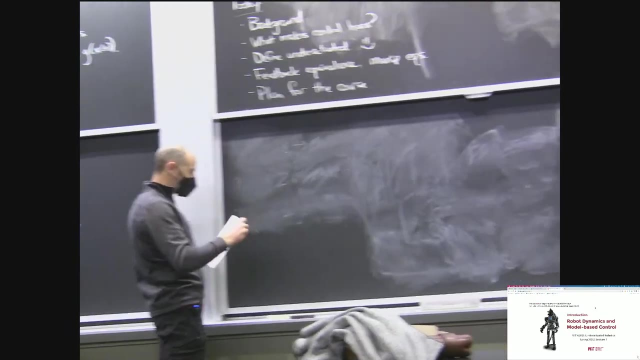 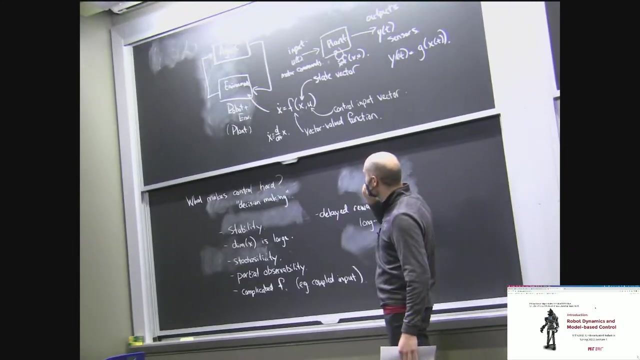 You know what makes control problems in robotics hard? My claim is a big one- is when a robot is underactuated. OK, So let's do it slightly carefully And I'll write the definition and then we'll connect it back to this. 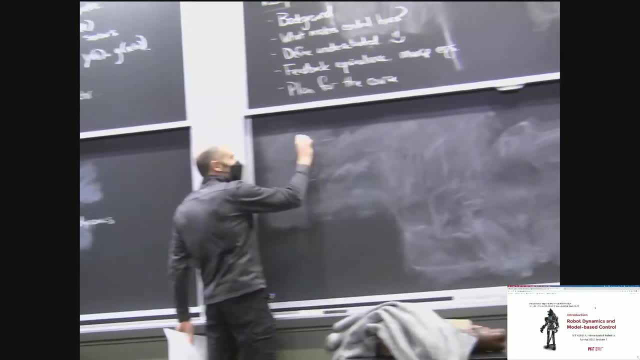 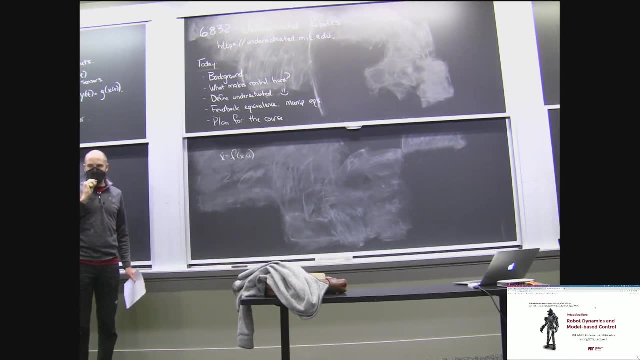 So, starting with our nonlinear differential equation like this: OK, OK, OK, OK, OK. I'm going to specialize this a little bit because we in this class, we're going to think mostly about controlling mechanical systems. Mechanical systems are second order in nature. 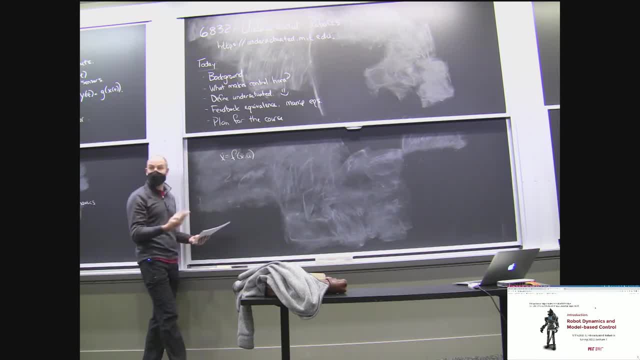 So it's going to pay. even though you can always write it in a first order form, there's more structure if you write the second order equations, OK, So I'm going to go ahead and define q as the vector of generalized positions. 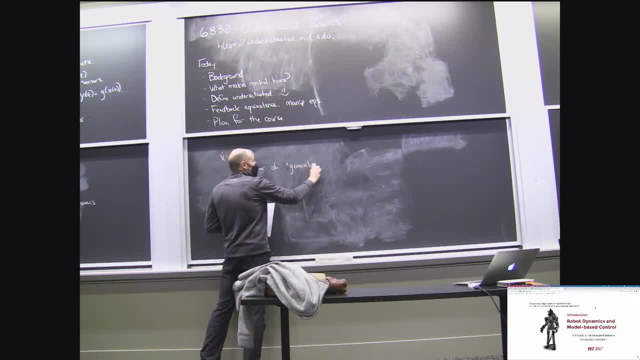 So for a robot, if I had a cart moving on a track, it would actually be the position variables of those, the location on the slider. But for a robot with joints it's actually going to be the joint angle. That is the generalized position. 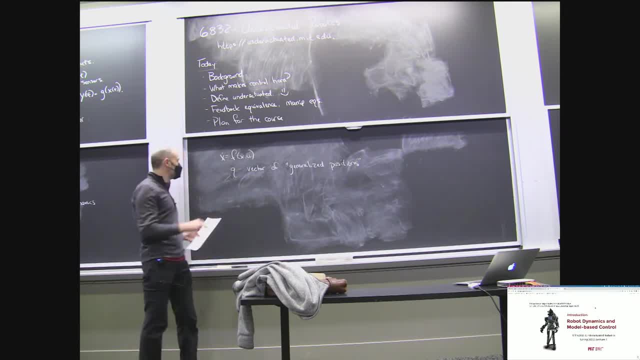 The angle coordinate tells me about the positions of my robots, And then I'll use q dot for the velocities, q double dot for accelerations and the like, And since mechanical systems are second order, I basically have f equals ma flying around. 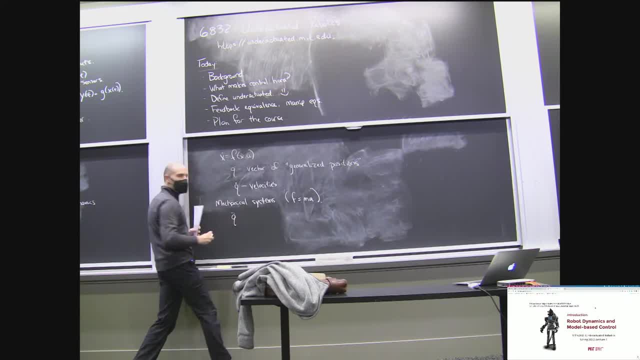 It's going to pay to write this in increasingly more specific forms, which gives us more structure to understand what's going on. So, instead of just writing the first order update, I'm going to write it as f1 q q dot plus f2 q q dot. 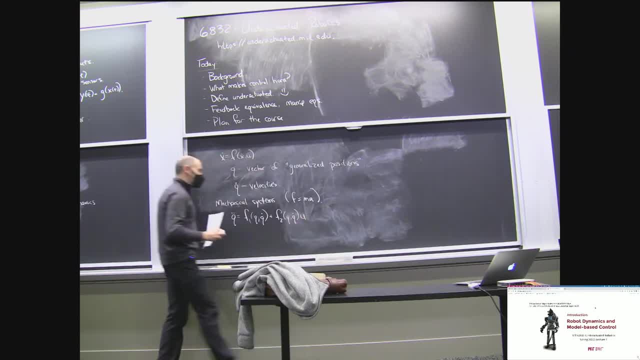 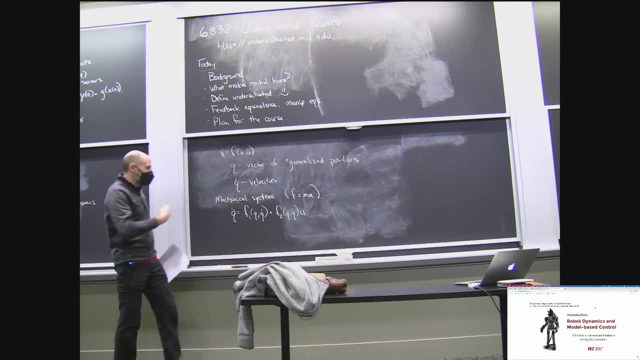 I'm also going to make one more assumption. as I write this here, I'm going to choose this particular form. I could have written it as just q, q, dot and u, but I'm going to go ahead and say: I happen to know that for robots, most of the mechanical systems, we care about the forces, the control. 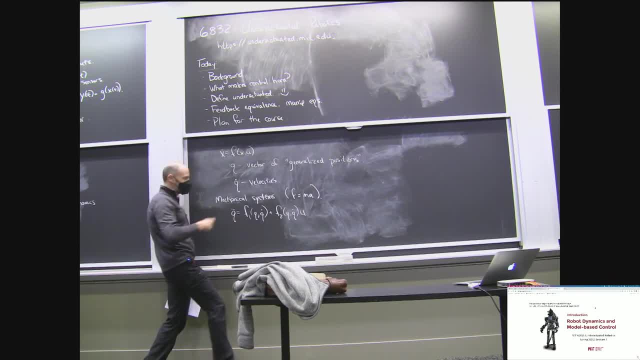 inputs enter in a special way. This is called control. affine: All right, The dependence. when you write a bunch of equations of motion for your robots and you get out of a differential equation like this, you look, you'll see that if your commands 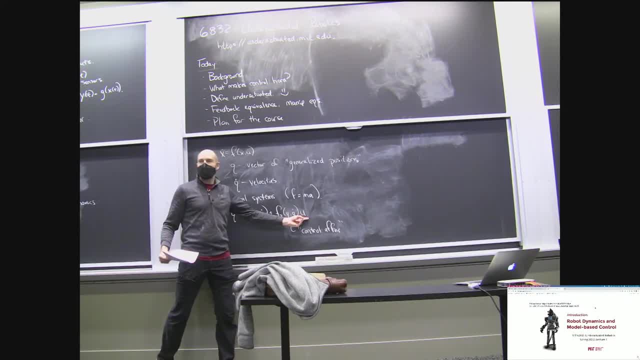 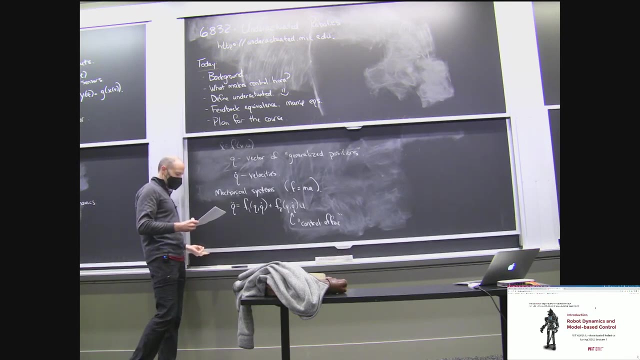 are torques, then they always come in a nice. you know it's linear in this term but it's affine in the whole thing, right? So control, affine, Complicated nonlinear terms. but the? u is simple, All right. 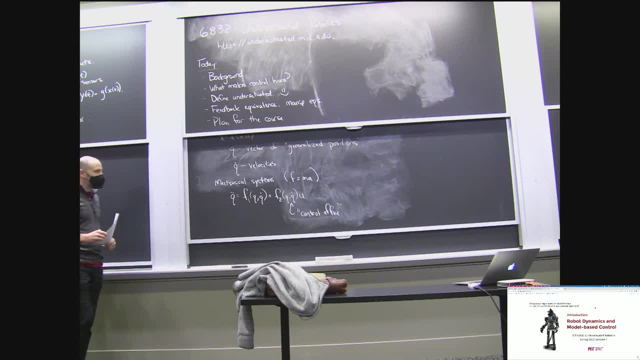 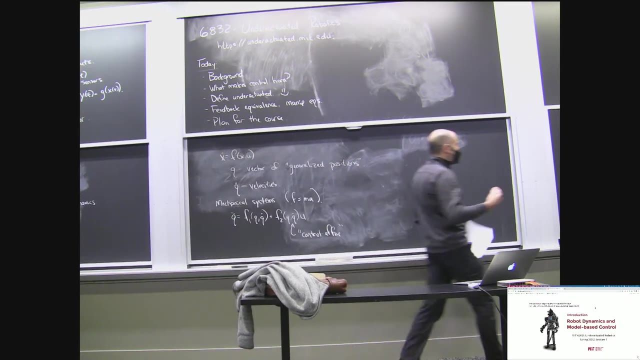 All right, Okay, We're going to even make, we're going to, we're going to get inside f1 and f2 pretty even in this lecture. we'll do it a little bit, Okay. So now we get to define the name of the class. 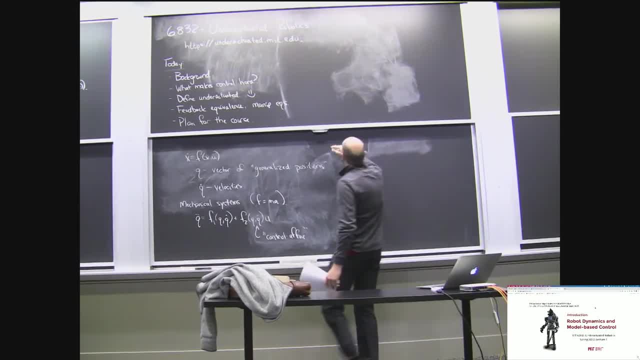 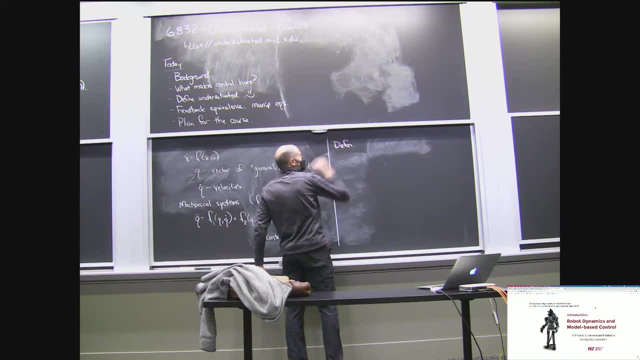 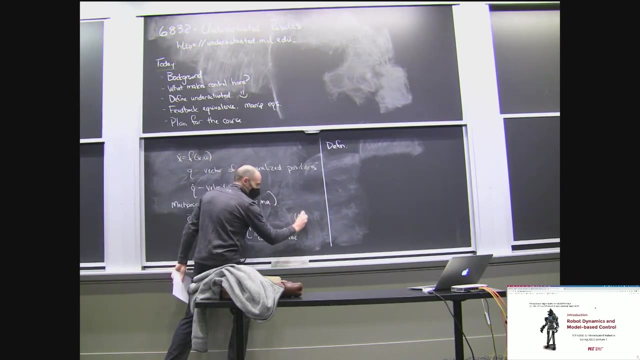 Okay, I'll see if I can do it right here. Okay, All right, I'm going to say a system described by these equations. Let me just use my sort of. let's pretend I had a LaTeX equation in a paper and it was: 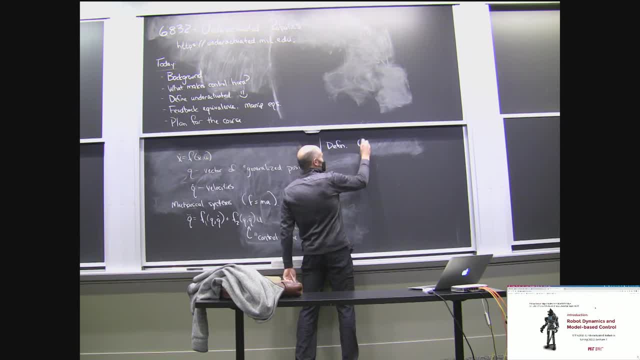 one right there. So I'll say: system defined in equation one is fully actuated. I'm going to be careful and say I'm going to in some state q. Okay, So I'm going to say I'm going to be careful and say I'm going to in some state q. 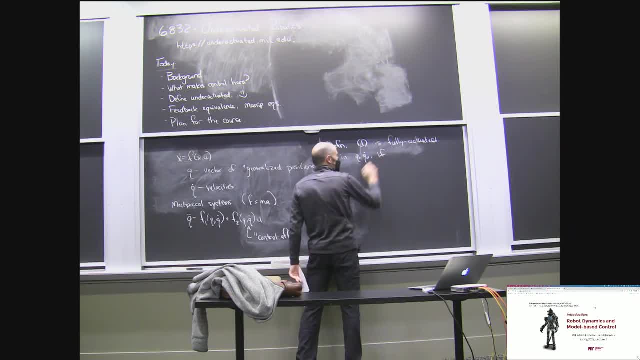 If the rank of this matrix, if that matrix is full row rank, if f2, q0, q0, dot is full row rank, We're going to understand why that's important, I think very hopefully very clearly in a minute, okay. 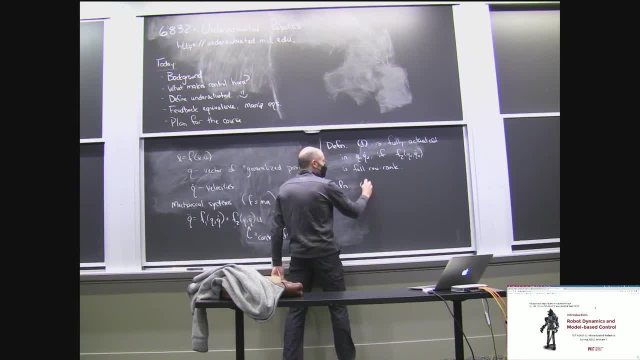 And that system is under actuated in that particular state. Okay, Okay, Okay, Okay, Okay, Okay, Okay. So you can see that the dimension of f2 is less than the dimension of q. Okay, So now let's unpack that. 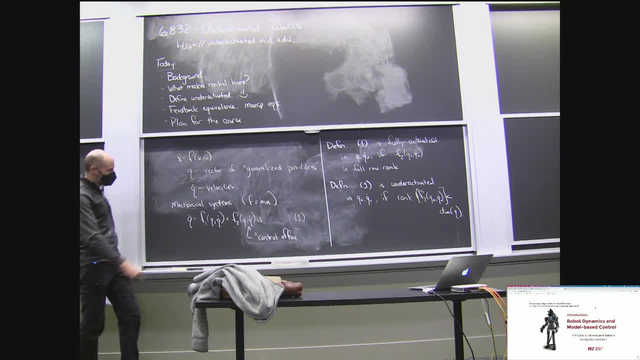 It's a pretty fundamental if the course is named after it, right. So in general, u is a vector right, q is a vector Right vector. I've assumed that Q and Q dot and Q double dot are all the same size vectors. 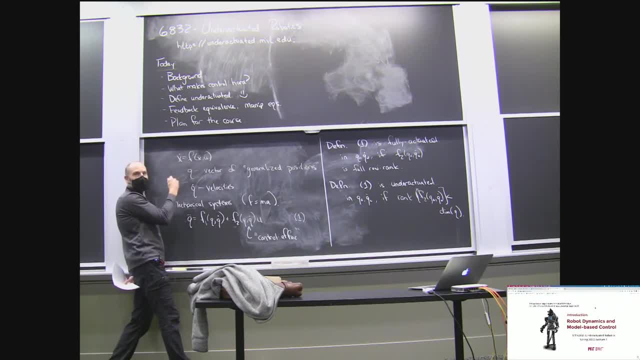 There are cases where that breaks, when you have quaternions flying around and stuff like this. but for now we're just going to keep it simple and say Q and Q dot are all the same size. So this is a matrix differential equation. F2 is a function, of course, of 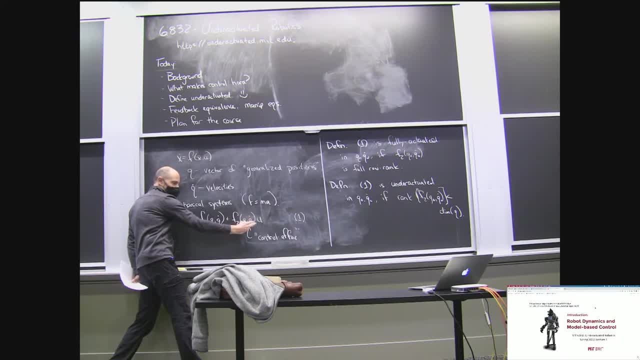 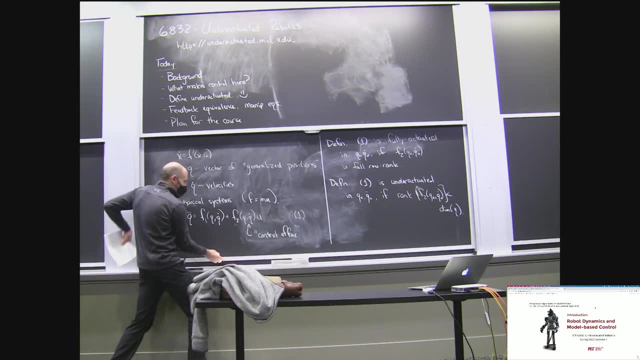 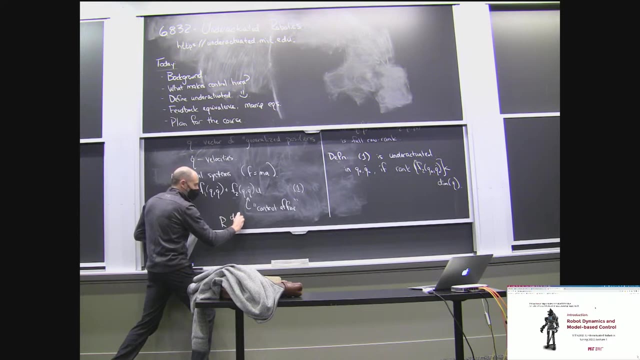 these variables, but for any values of those variables you put in. that's a matrix. F2 represents a matrix function. The size of that matrix is what It lives in: R of dimension Q by dimension U. It has to spit out a vector of Q. 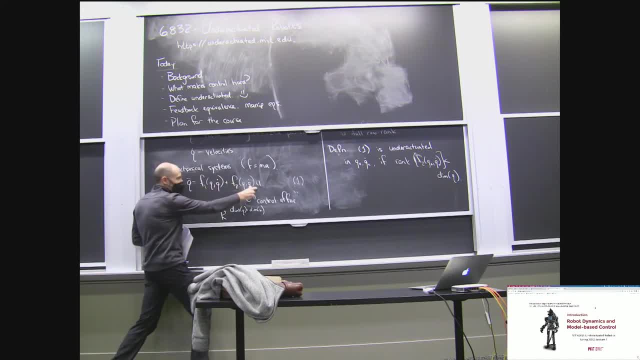 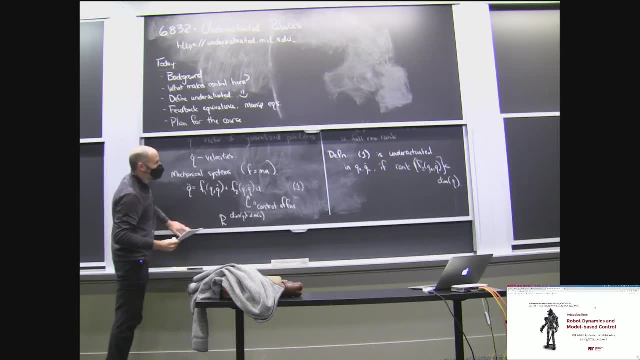 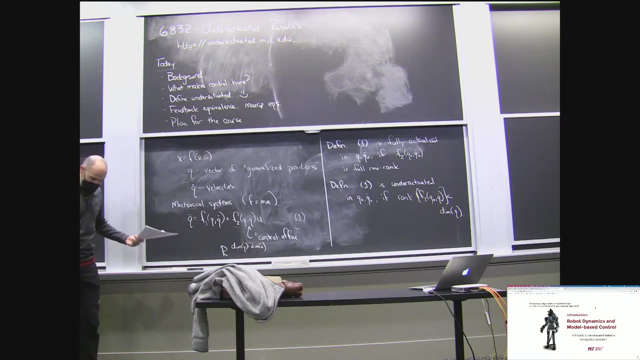 It has to spit out a vector of size Q to make this work, and it has to consume a vector of dimension U, whatever the dimension of that U vector is. So if I were to have a humanoid robot, for instance, it might take me many, many Qs to. 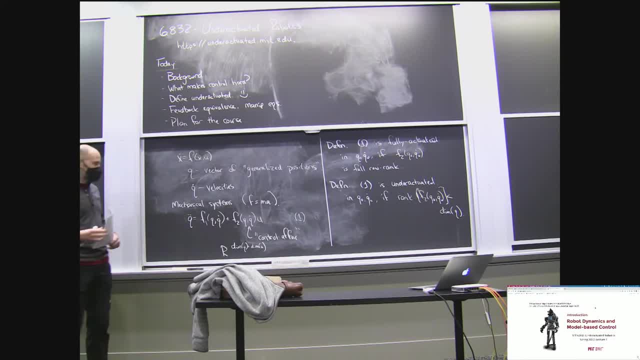 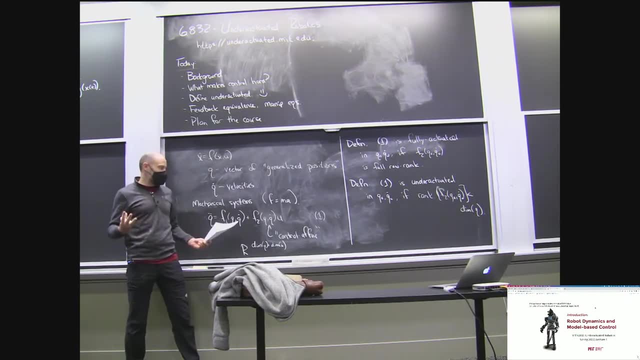 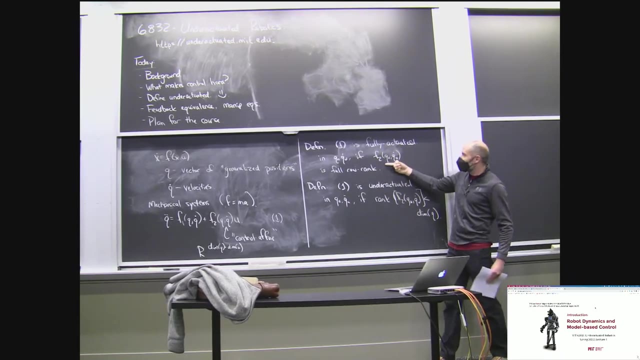 fully define what's going on in my humanoid and I've got some number of actuators. So if in a, there's a good case here. So first of all, let's see what does it mean to be? why do I say full row rank instead of just in column rank or something else? 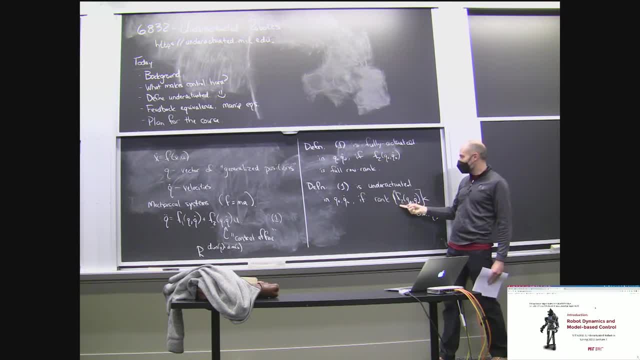 right, At most, the dimension, the row rank of this matrix can't be greater than dimension of Q, right? So being full row rank means that this is The rank of this matrix, is dimension Q And we, What does mastering of this dimension maybe actually mean? Yeah, That means that this is dimension X minus X minusagram. It's a function of the value de Dakle, And I have to build off it pretty well, Better, Well, So three days, you'll be like: okay, now who chin is. 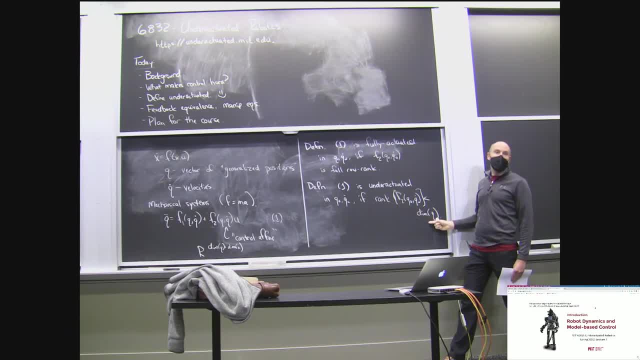 why we have one Yeah, And the rank of that matrix is less than dimension q, then I'm underactuated. Do we understand just the algebra of that sort of Yeah, OK, So when you're fully actuated, things are pretty good. 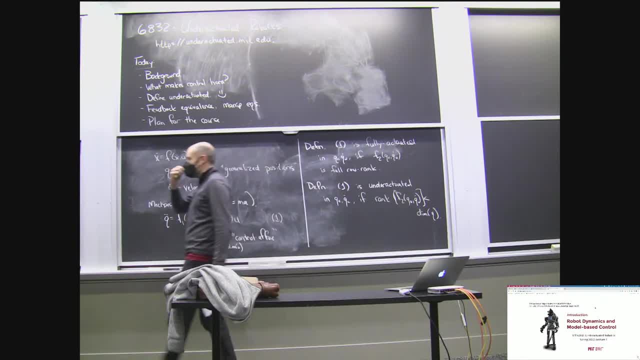 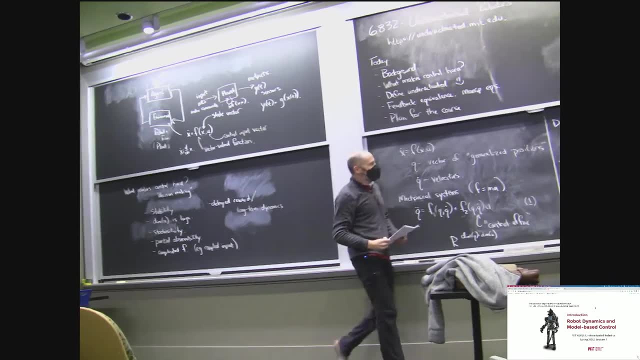 Life is pretty good, Control is. I mean there's different ways that control could if you're partially observable, But a lot of the control problems we want to write are not that hard When control is underactuated. that's a particular way that control gets pretty hard, pretty fast. 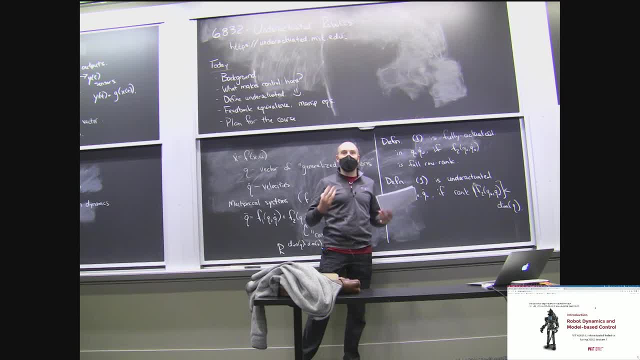 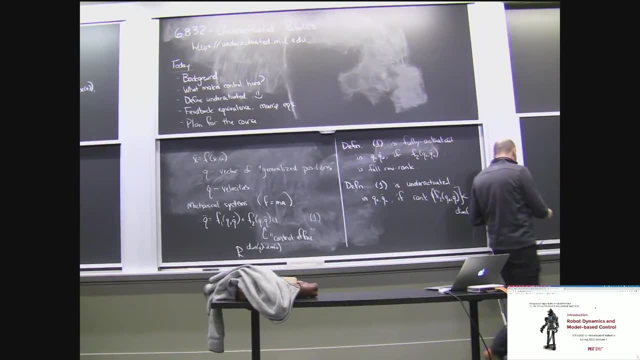 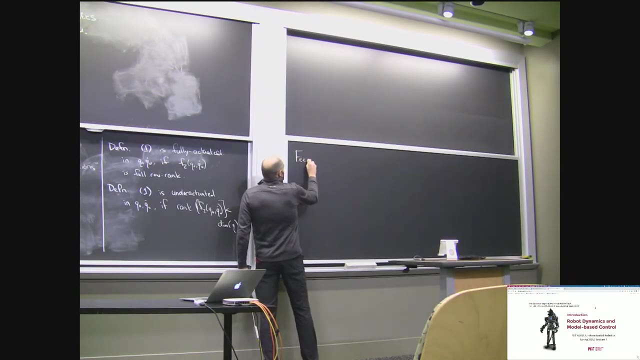 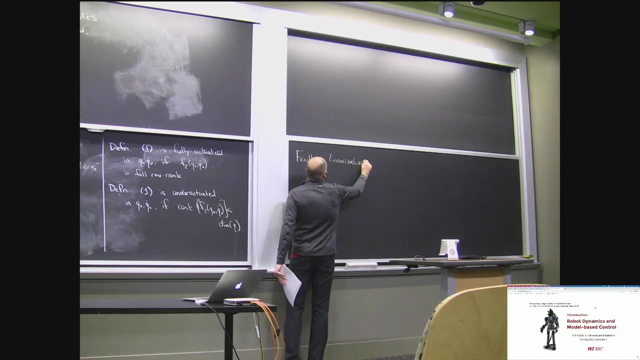 And it happens to be the one that dominates the way we think about walking robots, fast flying UAVs and other cool systems. Let me try to convince you of that by telling you what feedback linearization is, ideally with a demo, If the projector starts working. 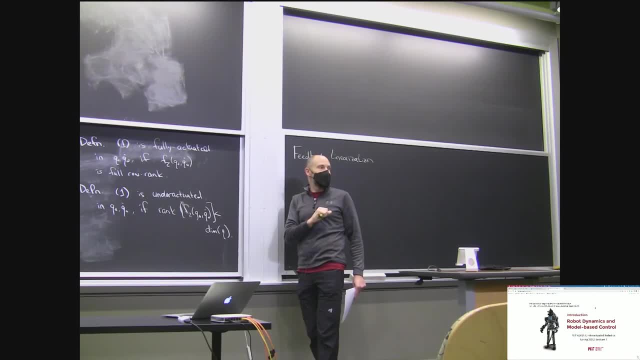 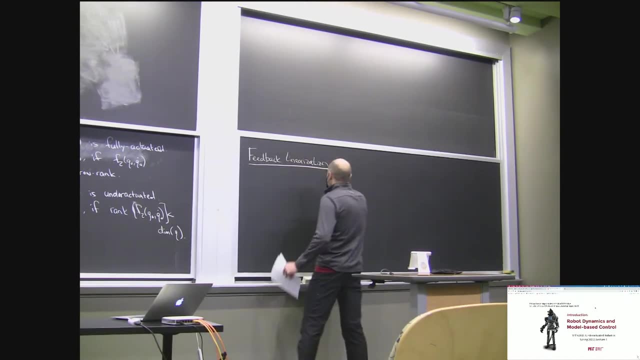 Any sign? Good, Yes, OK, right now. Yes, Go for it, Thank you, OK. So let's say I'm working with my matrix equations here, Control affine form. I'm going to assume that I know F1 and F2.. 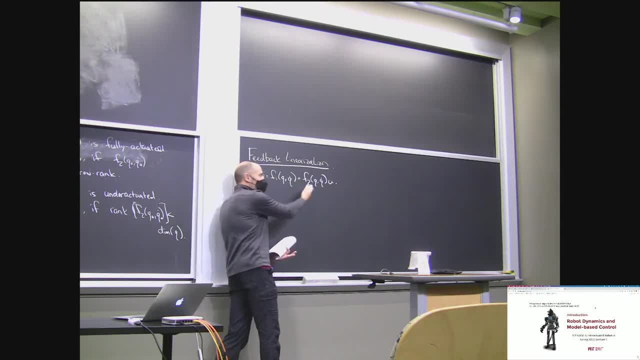 There's a very interesting generalization of this when F1 and F2 have to be estimated or learned right. But let's just assume we know F1 and F2.. So if I'm given this And I'm given a design, 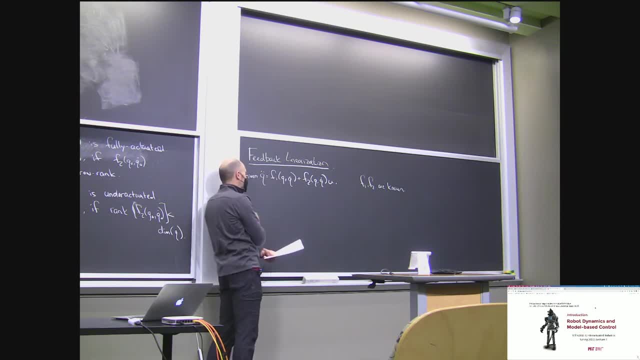 And I'm given the desired acceleration that I want to produce. have my robot produce. My claim is that a simple control law exists for fully actuated systems that can make the robot do exactly what I want it to do, And that's what I want any time right. 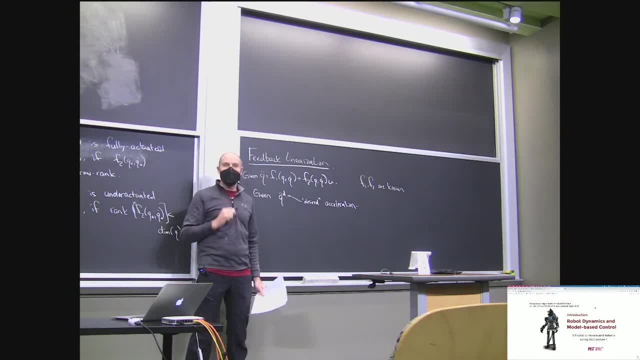 The property that matters about whether I can achieve an arbitrary desired acceleration is exactly this full row rank matrix. OK, And you can just see that with a. that might be enough, But we can just see it by saying: let me write a controller. 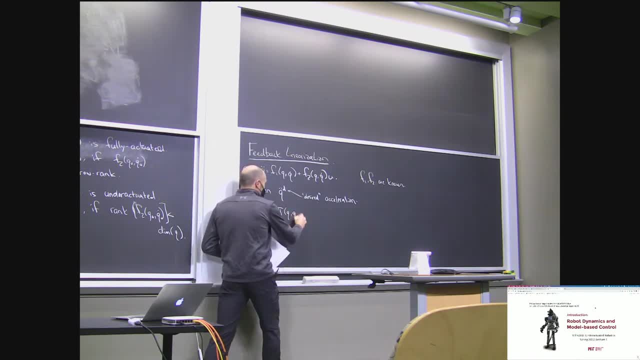 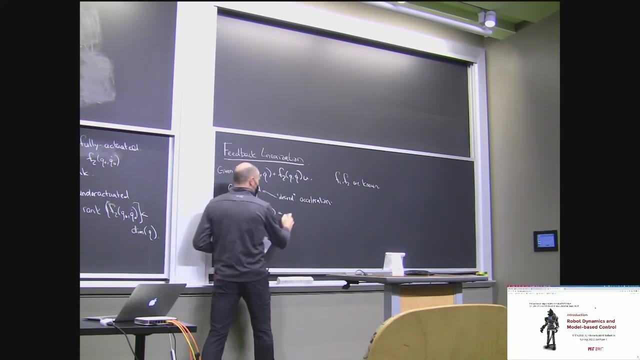 I'll say my controller, of course, has got to be some function. This is my control policy. I get to choose it right And I'm going to choose. since I know F1 and F2, I'm going to choose to use F2, inverse right. 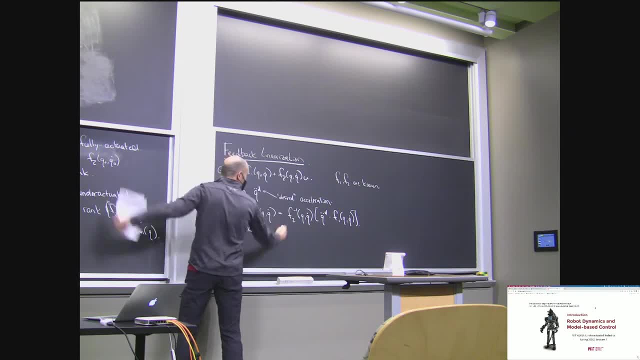 That's a valid controller if F2. Right, OK, F2 is invertible, And it's invertible when it's full rank, right? Why is that a good controller? As you can see now, if I were to take this controller, 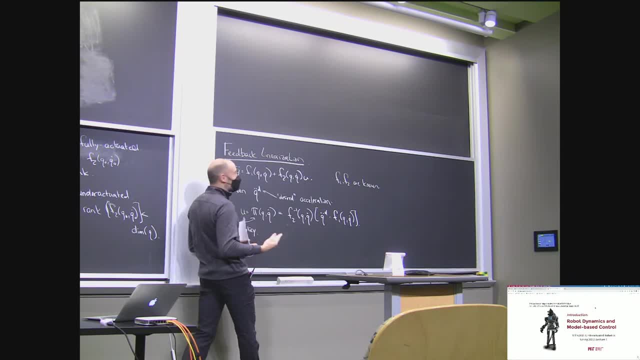 stick it into the equations here: solve for the closed loop dynamics, And I'm just going to substitute this into u here to see what the controller plus the plant do together. Then this term cancels. This term cancels, and I just implies the closed loop dynamics. 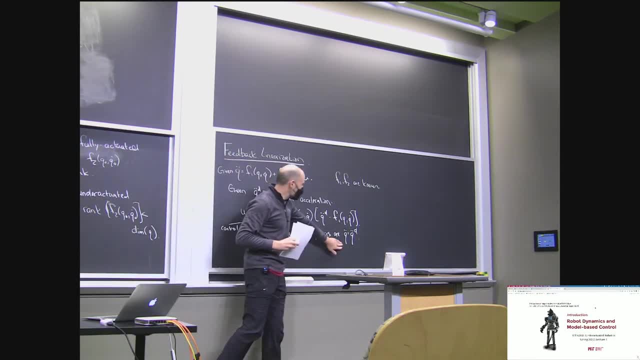 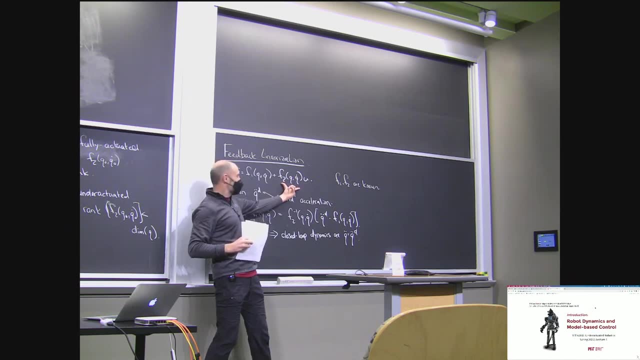 OK. So in the case where I have a big enough controller, a big enough F2 matrix, I can basically instantaneously command the robot to follow any acceleration I want it to follow. Why is that a big deal? How does it make control easy? 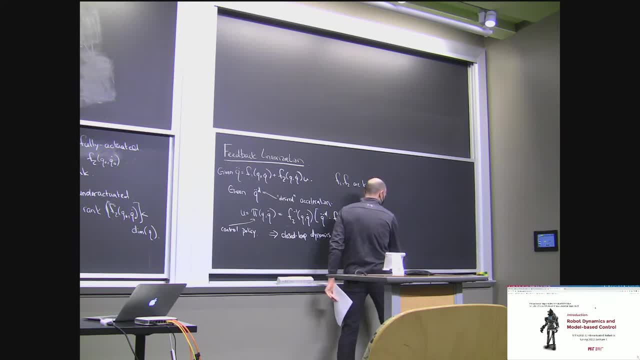 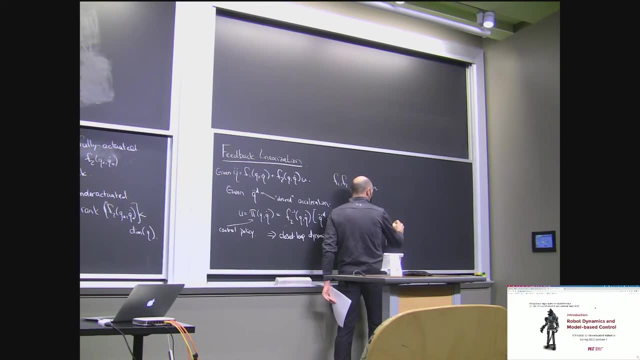 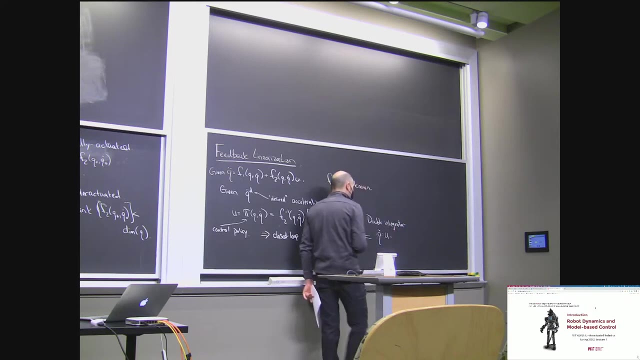 This system. now I can think about it as a different system that I might want to control. This is a very famous simple system. Q is a vector, It's a stack of double integrators, It's a linear system and it's a trivial linear system. 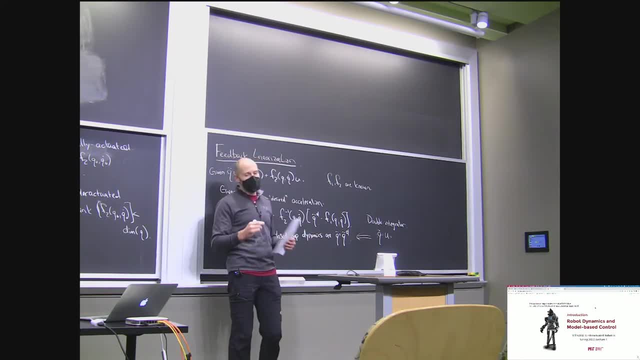 So if I have long-term objectives, try to get to a certain place at a certain time. I am actually very good and we'll derive some of the So controllers. I'm very good at controlling this system, Even if there's long-term delayed reward. 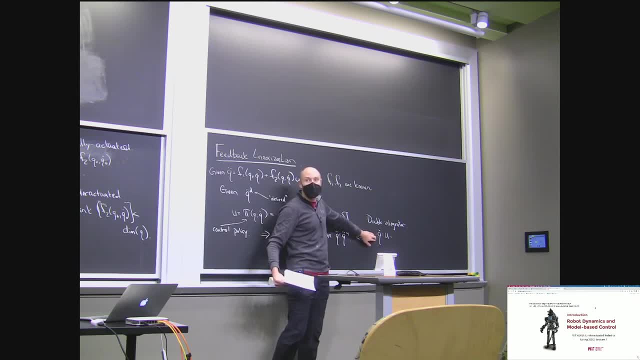 other kind of things. this system is simple enough that I can write very strong controls for it. In the case where this matrix is full row rank, I can apply this controller first to show that the system is feedback equivalent, And I can also set the speed of the robot. 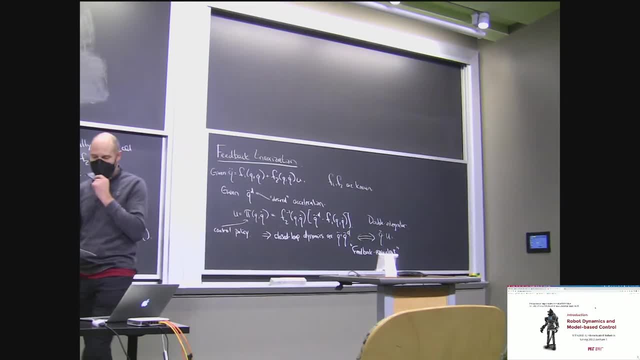 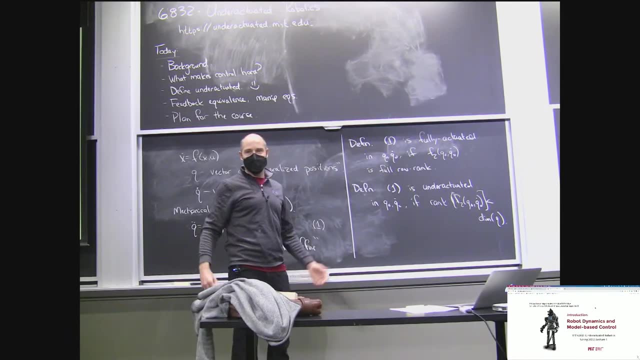 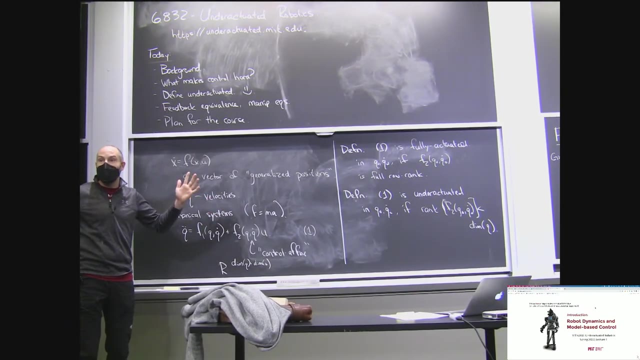 to the double integrator. Now here's a place where movies would help, but I guess I'll just use the humanoid robot as an example And I'll use myself as a prop, I guess, Right, So OK, Humanoid robots used to walk like this. 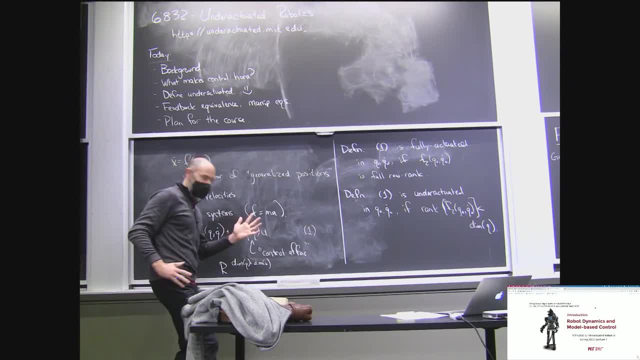 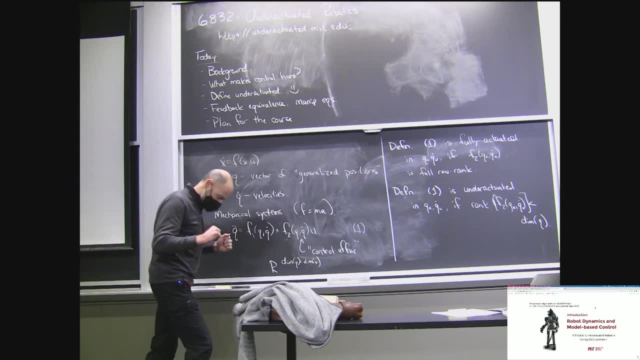 OK, Right, They used to. you know it's sort of ridiculous, but that's really what they do. Actually, When they started at the dawn of robots, they actually moved. worse, They would first put their weight exactly over the center of support of one foot. 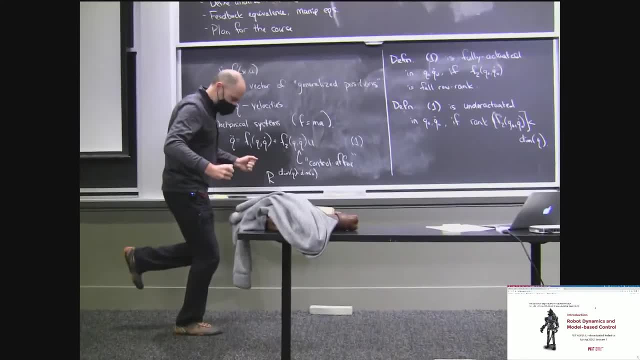 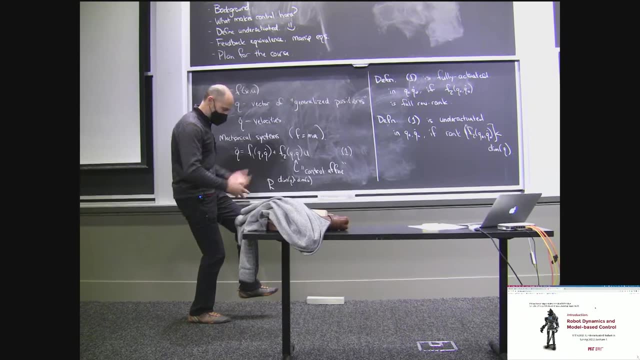 They'd keep their center of mass directly over there. They'd very slowly lift this leg And then very slowly, you know, while keeping this velocity low, so it didn't affect- add any complicated terms, you know, and then put things forward. 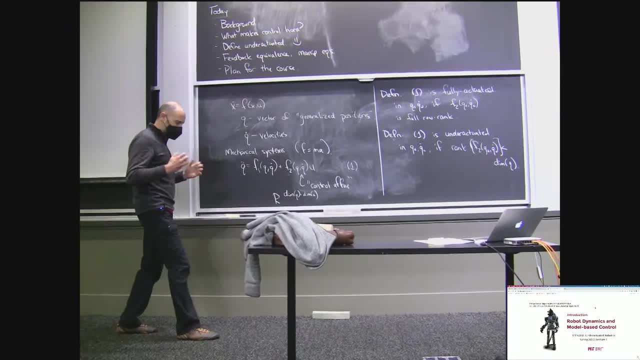 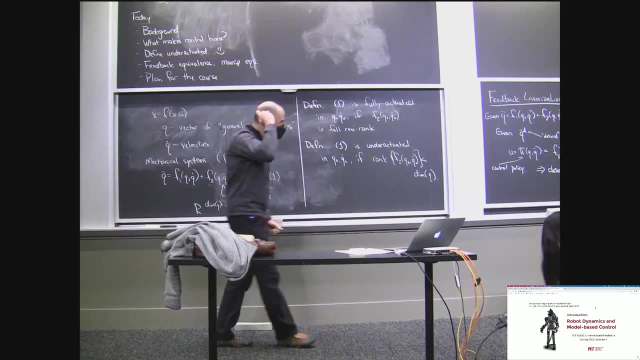 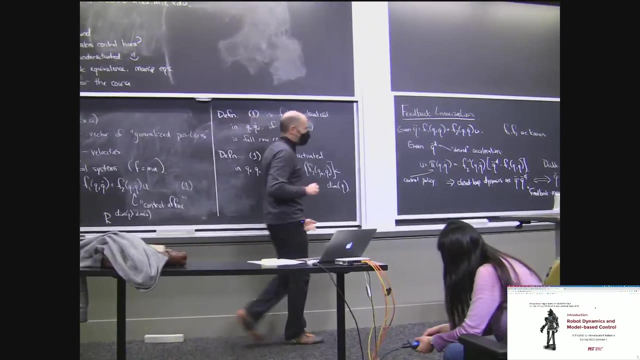 But even recently, you'll see robots that are moving. you know, like this, right, Right, What are they doing? OK, They're doing something sort of similar to this sort of this exploit. OK, which is that what we're doing here? 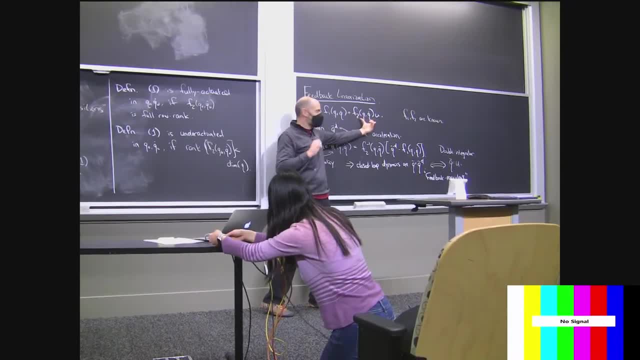 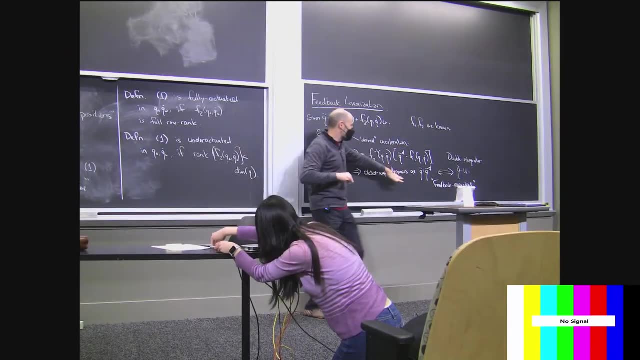 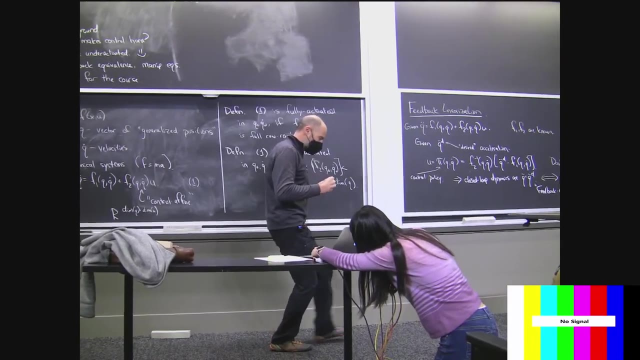 is effectively taking some beautiful dynamical system using a feedback controller to cancel out all of the dynamics of that system and then replacing it with a different dynamic. So the fact that we're, you know, we're seeing robots that move in ways that look inhuman. 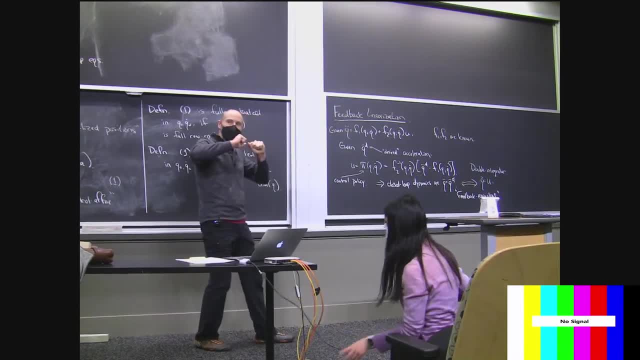 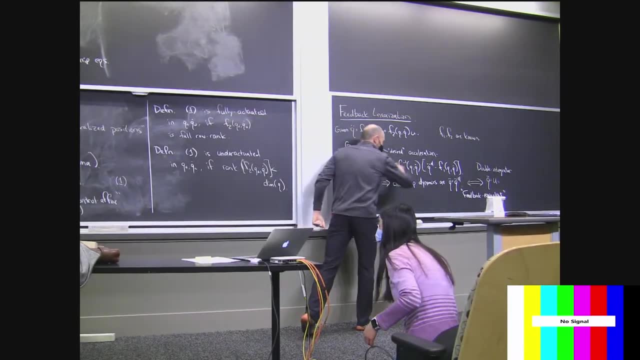 They don't look very physical, right? It's because we're using potentially excessive amounts of energy and control effort in order to try to erase, invert, you know, the matrix and subtract out all the other terms in the equations. Yay. 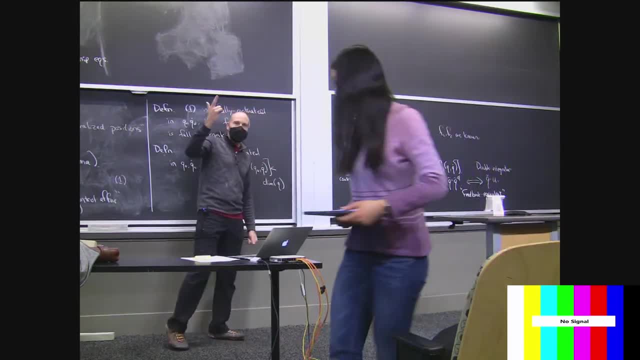 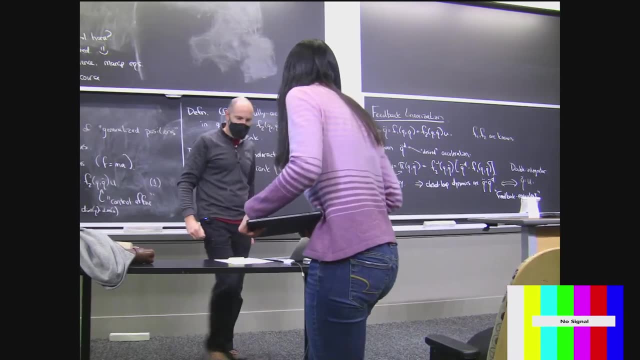 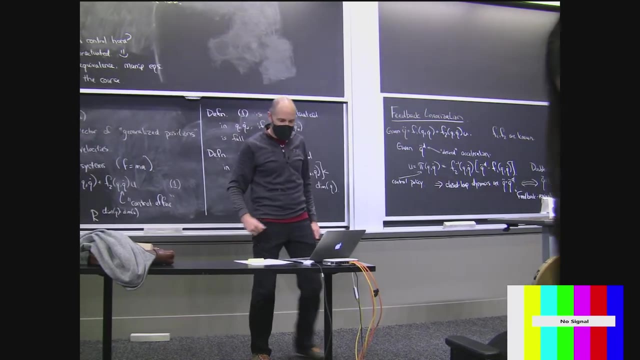 OK, Thank you, Lou. Was there something non-trivial back there or did we just like? Really, I don't know. I just unplugged it, OK, And I think it worked OK. OK, This is not plugged in. 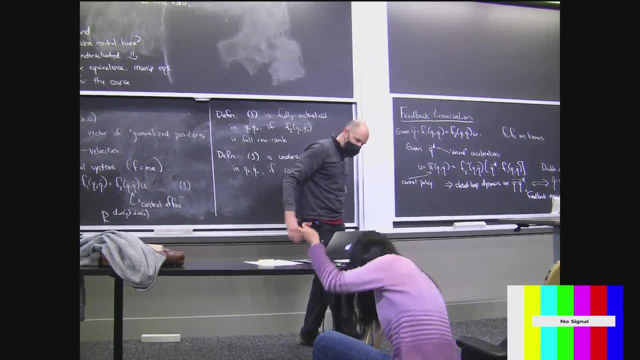 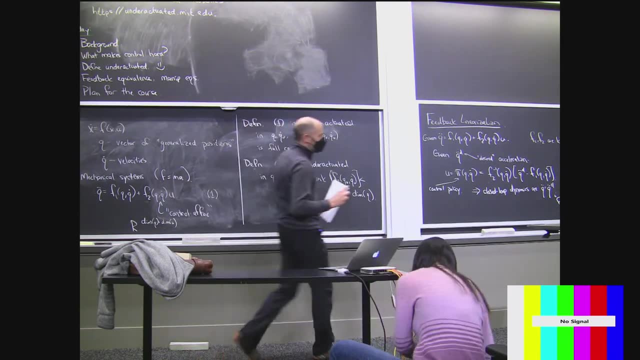 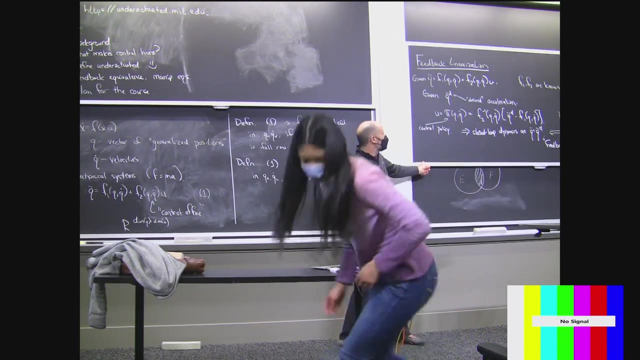 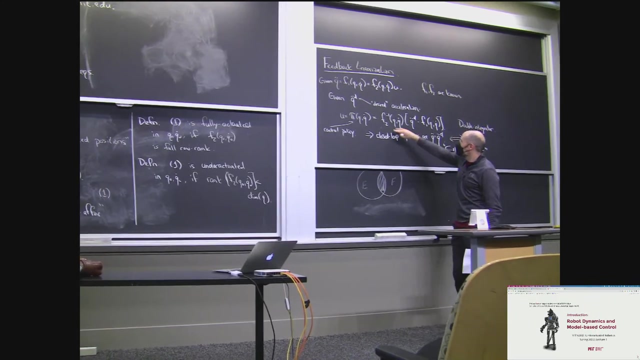 Oh no, Oh OK. So we have many ways that control could be hard. But if you cannot do that, If you can do this control, then there's a particular way that control gets hard for robots. You don't get to cancel out the dynamics. 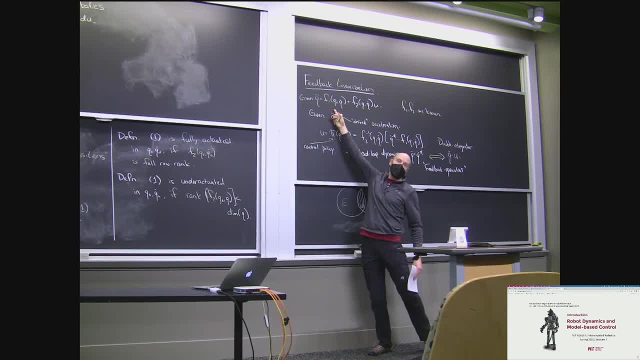 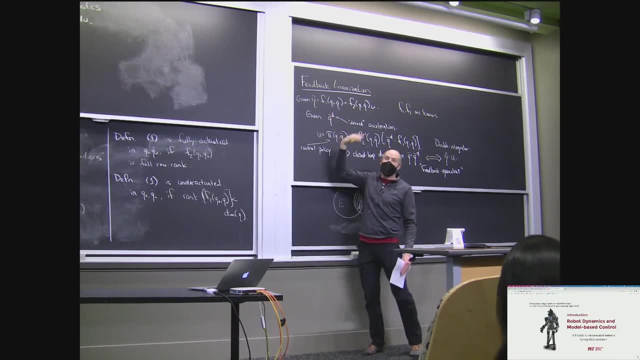 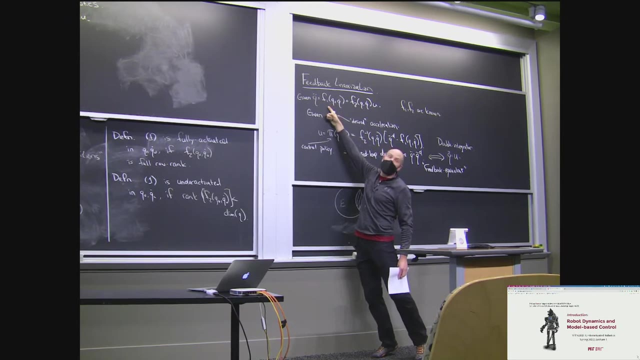 You have to think about the dynamics over a longer range of time. You have to deal with complicated F and long-term dynamics. OK, That's. the emphasis of this class is digging inside, understanding how to do good control when F is complicated and you can't. 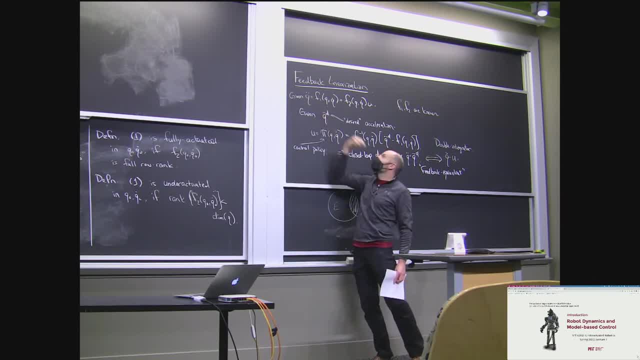 You can't erase it. OK, That happens when you're doing backflips. That happens if you're a UAV flying fast. Any time the dynamics start to overcome your ability to do control, then this comes at an important effect. Let me get a little bit back on the original plan here. 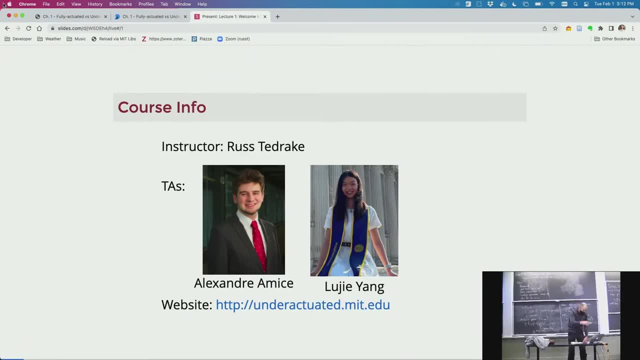 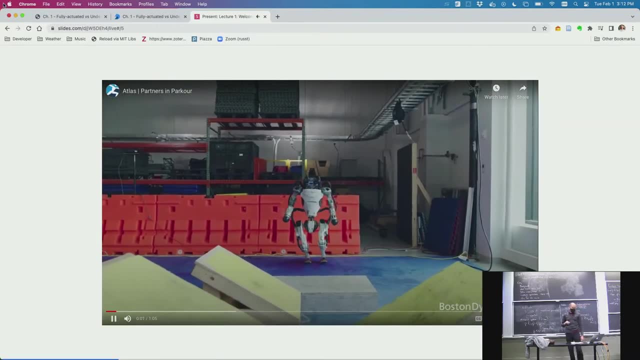 and introduce Alex and Lou. OK, I'll go back. I'll go through that later. OK, You've seen backflips. You've seen dancing robots. Right, Let me just. I have to play this because these are all my friends doing this and it's just so good. 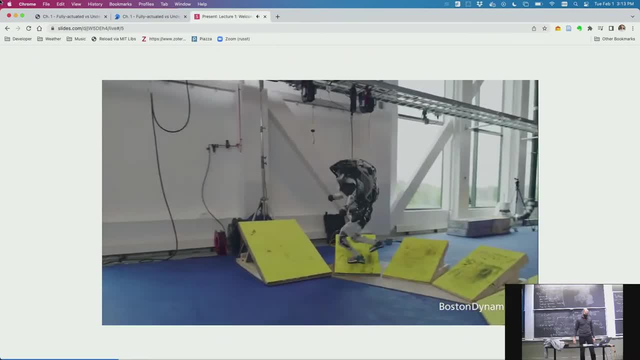 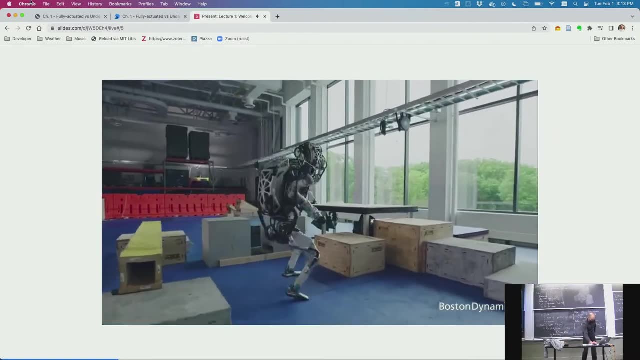 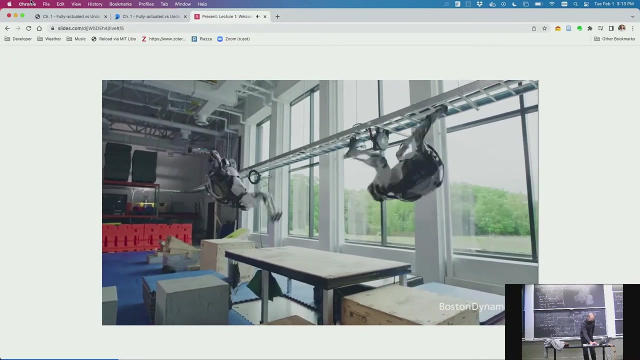 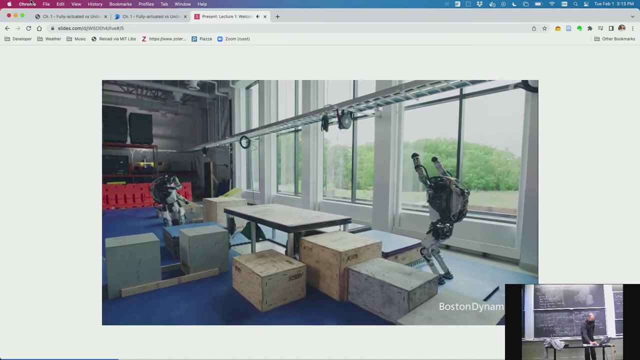 But I'm going to do the test soon. Stop, It has to be earlier than mass of four's count. How long? Three minutes, Two minutes, Three minutes, OK, OK, How about this? Let me go to this. How about that? 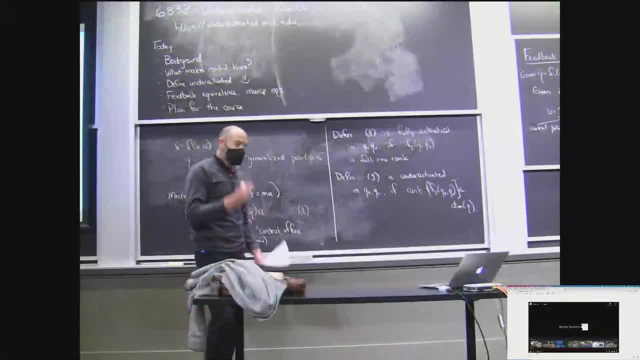 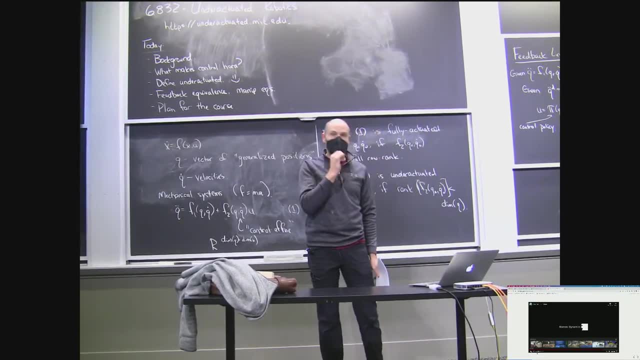 OK, OK. So it's actually interesting. Those robots are somewhere in between the two. you know the extremes of being fully actuated and underactuated. They have a ridiculous amount of power in their joints. We'll talk about exactly the subtleties. 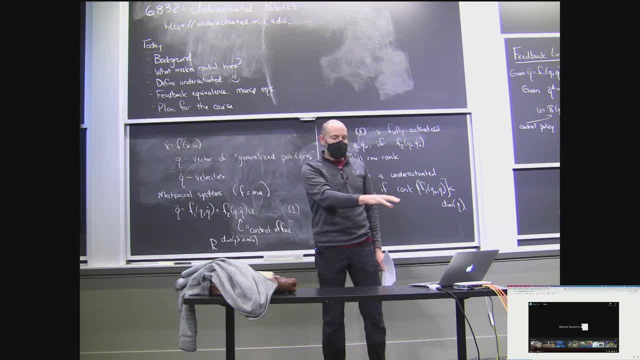 But that is so. I mean, first of all, many of the TAs from this class are on that team working on that robot, right. This is. there's a strong lineage, I guess, from the class to those results. 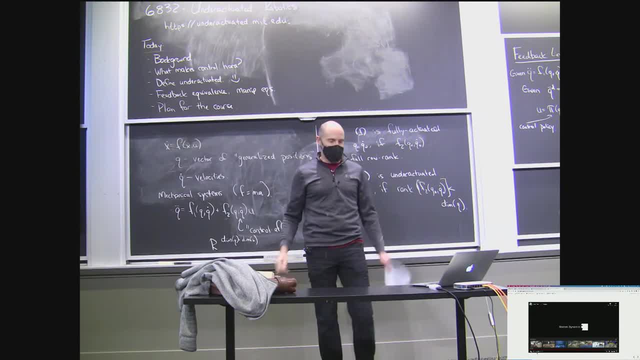 So, and I think they're the best results ever, But- and roughly- we're going to try to teach you about how to do that in this class. That would be. you know, that's the kind of thing we can we're going to dig into and give you tools for throughout the semester. 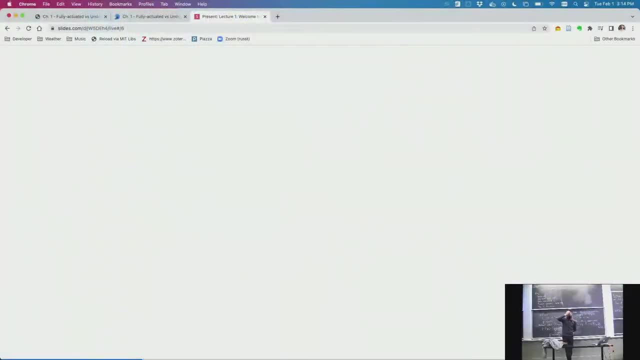 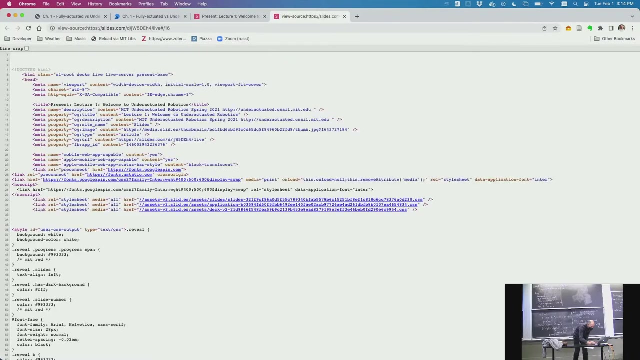 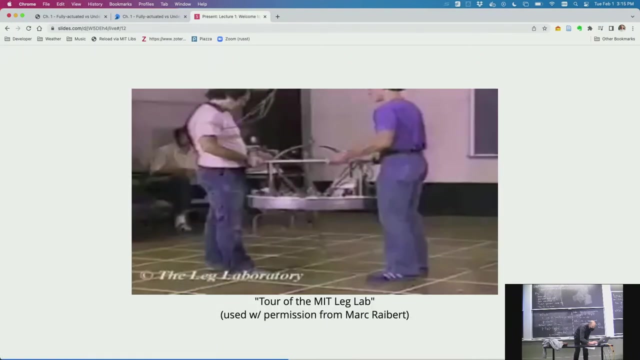 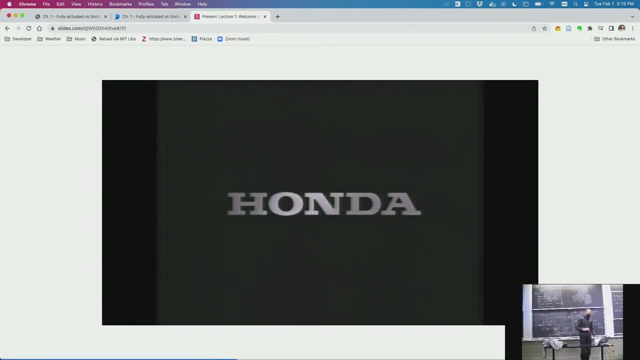 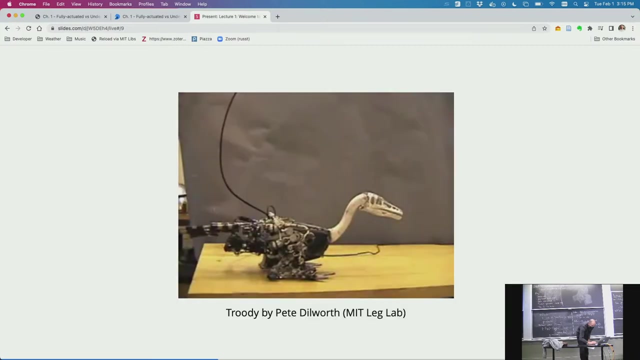 Okay, So let me make. okay. Got to sync two threads here. Let me jump ahead. Okay, All right, I'm going to just, I'm going to just go back through it, because I think otherwise my slides are going to be. 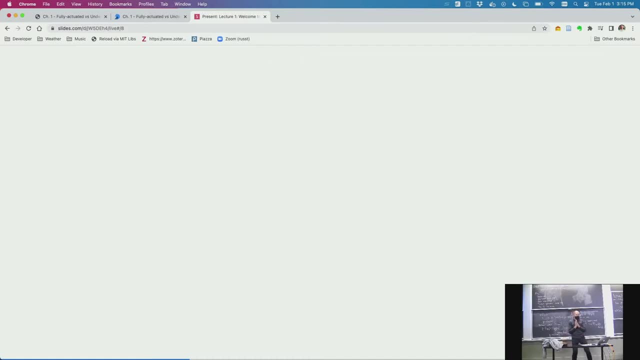 I'm going to be fighting my slides the whole time, So the lead in I was going to give you, which I will. I'll give you still, which is a little bit about. since you've seen the Boston Dynamics videos, I don't really have to motivate you on that. 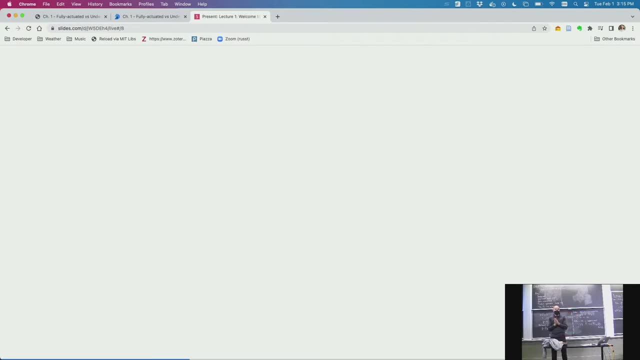 but what I can give you is, um, you know a bit of my history and how that and how those robots came to be and, uh, why the sort of technology built up the way it did. Okay, It's actually. 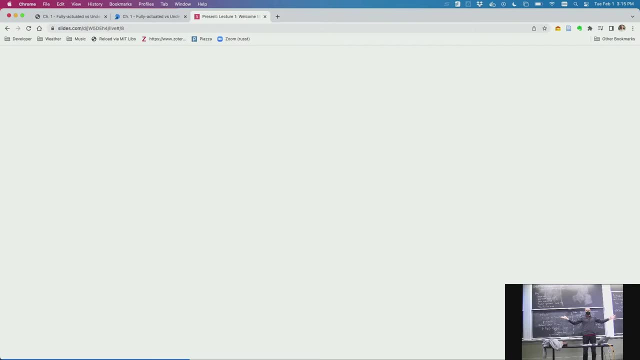 I mentioned, as some of you were coming in, this is E25. I'm not normally in. it's the first time I've taught an E25.. It's been renovated. This building used to be where the neuroscience lived. Okay, Um. 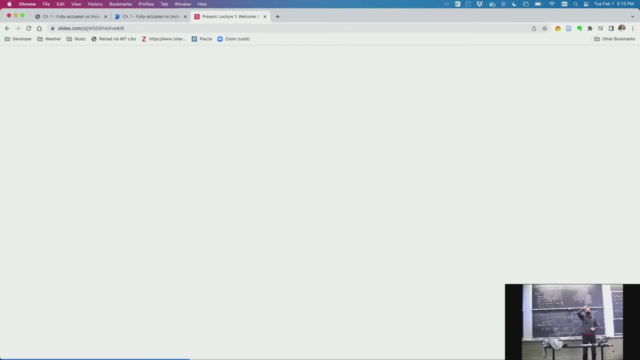 I actually had an office and I worked with a neuroscience professor for my PhD. Um, I shared a monkey, an office with a monkey on the fourth floor, because, uh, I was this- I like needed a little space to build robots, and they didn't really have space except for in the lab where they train the monkeys. 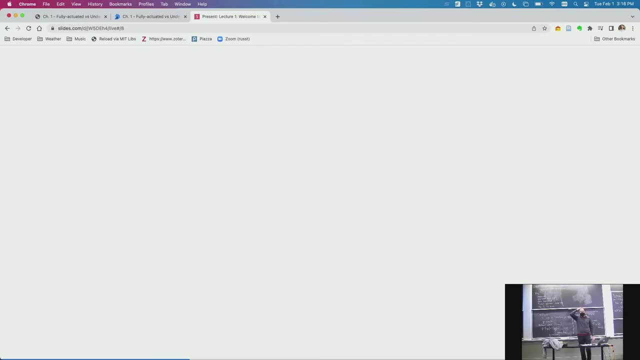 So, um, that was awkward, but it was. you know, it was good I had. I had a little space of my own to build a walking robot in a neuroscience lab, Okay, But I used to hang out at the leg laboratory. 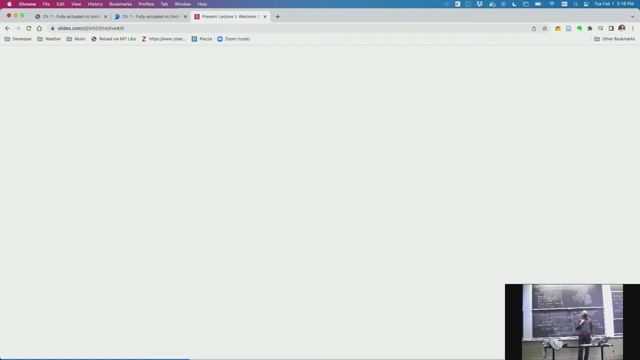 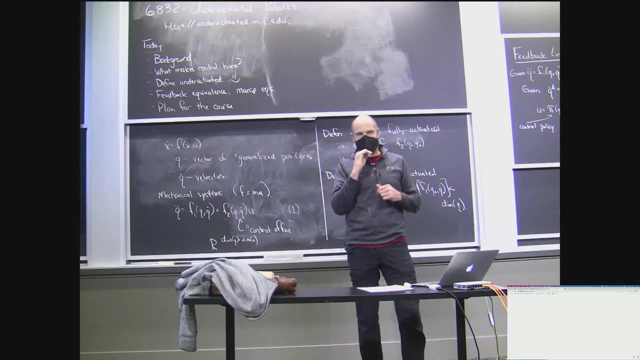 which was in the in the basement of any 43. Okay, Which is over by Akamai and everything. Now, um, the basement of any 43 was this wonderful place. There were old rope walking robots hanging from the ceiling and there was just dripping with with. 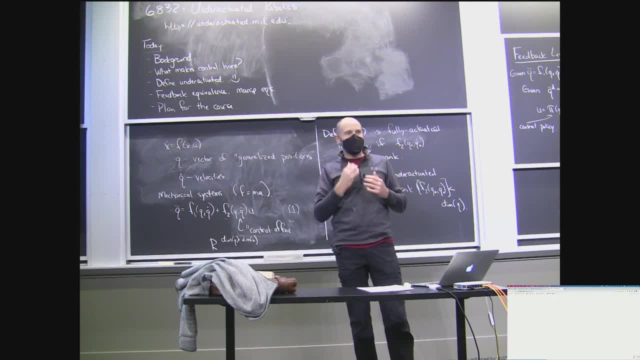 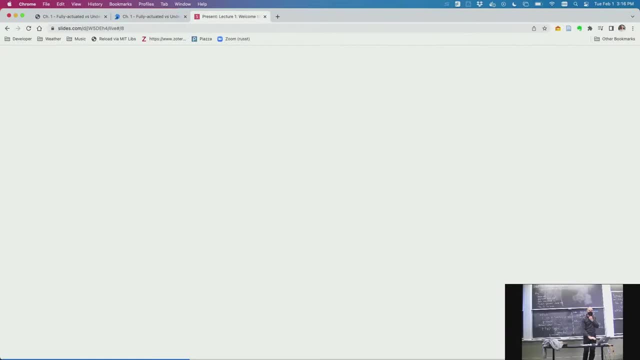 uh, history that where, where the leg lab, you know. and and the Boston dynamics lineage began when I showed up, um, as a grad student in the year 2000,- which was right around time, And I guess some of you were just being born, maybe. 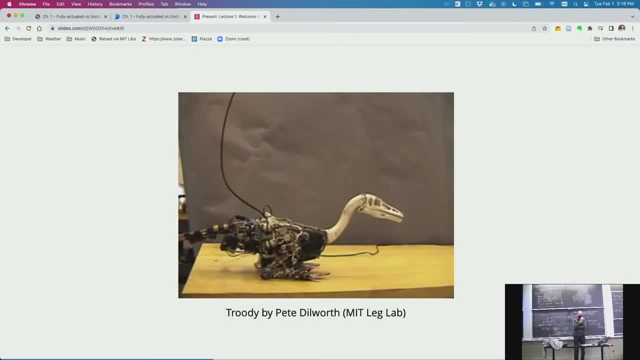 but um, this was the robot that Pete was working on off in the corner. This is, uh, he called it Trudy. It was built out of hobby servos, which were just powerful enough to do it. But um, 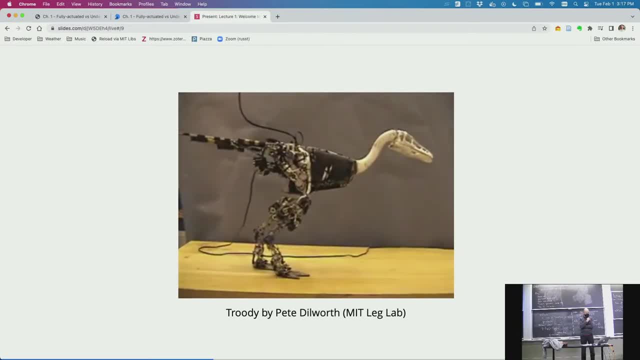 uh, basically, I saw that robot and I and I never looked back. I was completely hooked for the rest of my life. I was- I mean, I was always going to be a roboticist- but uh, but this robot, completely. 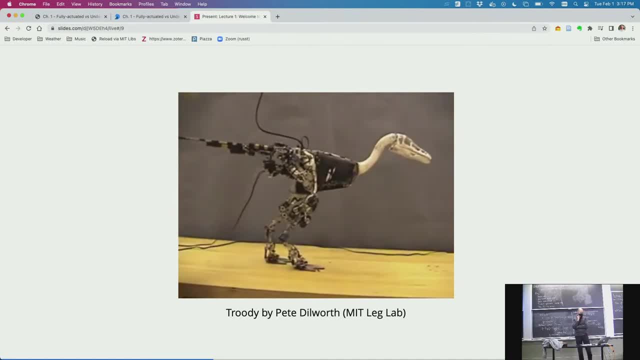 completely sold me. Okay, There were a bunch of robots falling down all over the place too. Okay, There were a bunch of robots falling down all over the place too. This only walked a few times, you know, successfully. but 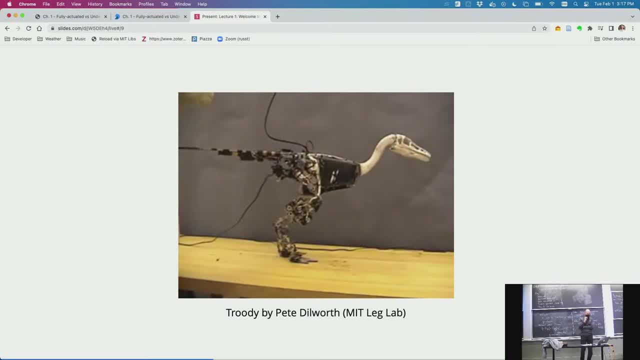 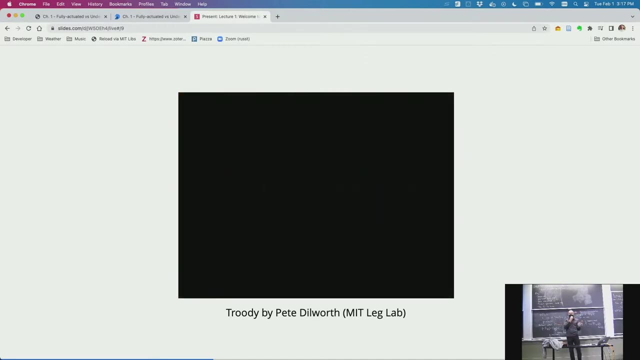 but that was enough for for for me to be completely hooked. Okay, Uh. but the history in the leg lab was so great? um, because it started in the early eighties with Mark Raybert. He actually started at Carnegie Mellon and then moved the lab to MIT. 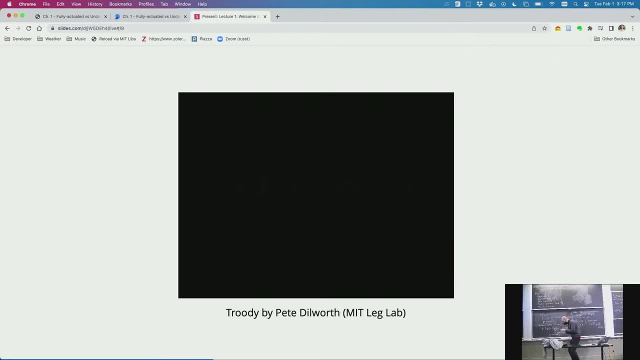 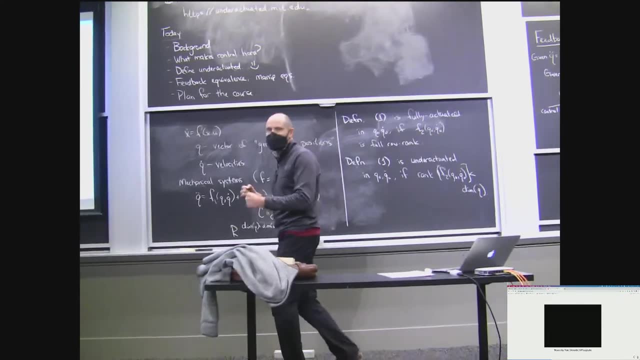 Right, And it started at a time where the robots were really walking around with their trying to put their- um, you know- weight over their, over the center of support, uh, and moving extremely slowly, And Mark Raybert and the leg lab started building these machines that 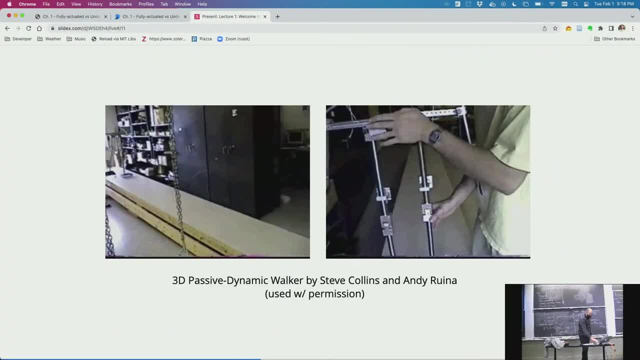 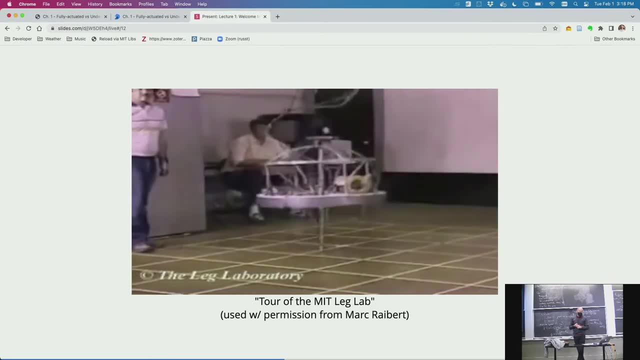 um, that totally changed- I'm going to do a lot of out of order here- totally changed the way people thought about robotics. right, They were pogo stiff stick based robots. This is the three D version of the hopper. 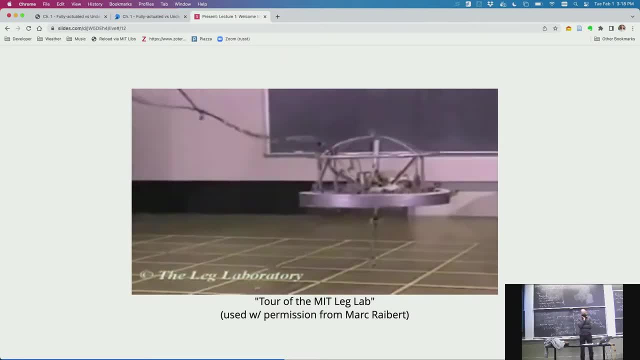 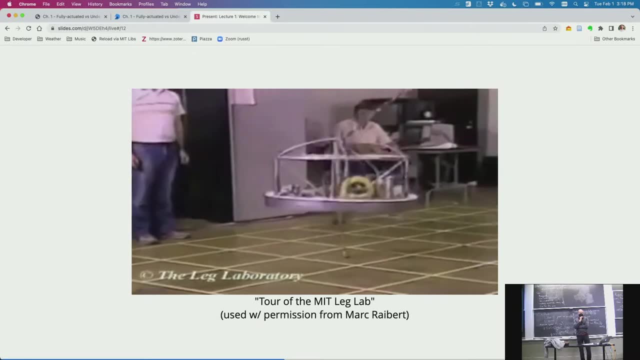 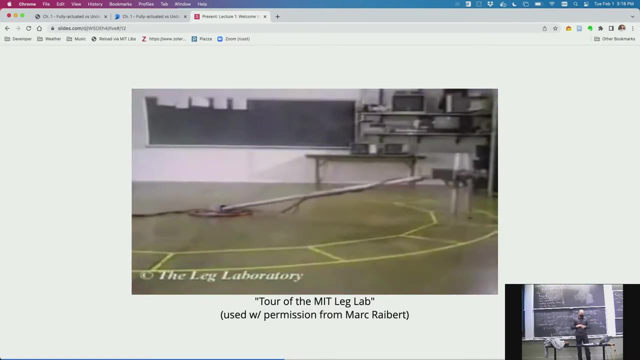 There were two D hoppers before that. Okay And uh, these robots, uh, you know, did use their dynamics in a dramatic fashion where most people were trying to cancel out their dynamics and move extremely slowly. Mark started building robots- that 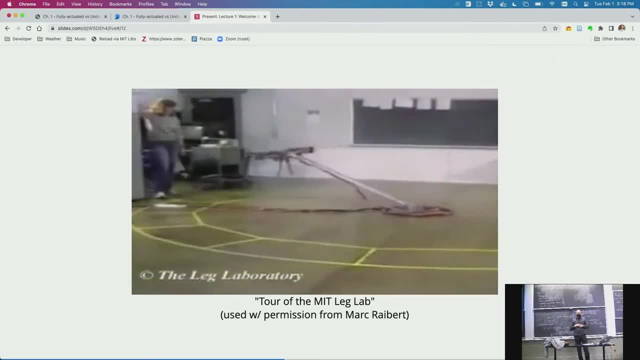 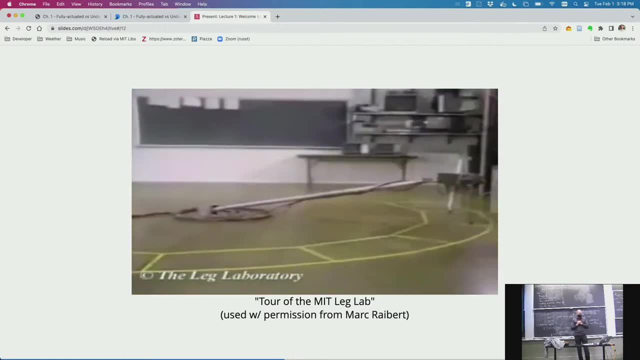 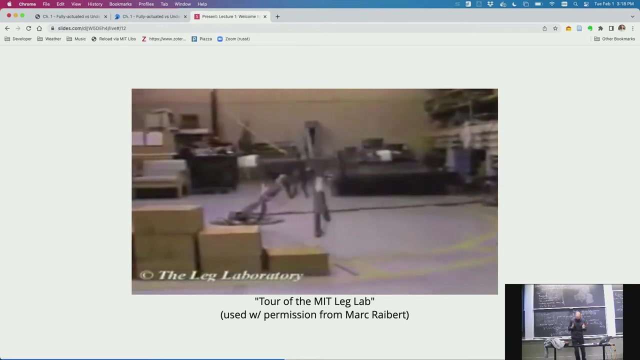 that threw themselves through the air. you know, and in a strange way, um, the control problem for legged robots gets easier when you start moving faster. right, It's actually harder and requires more accuracy to keep your center mass perfectly over your. 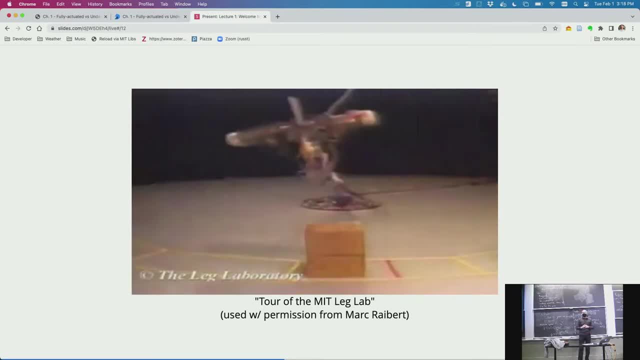 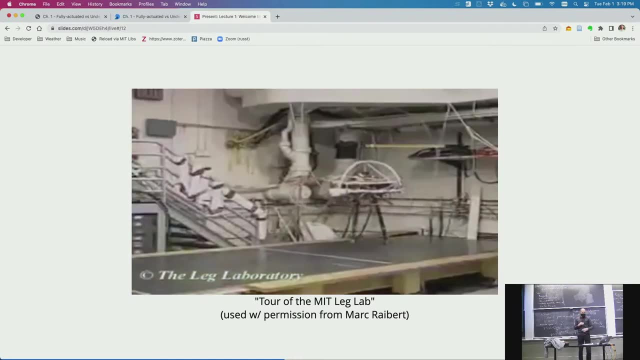 your support polygon That it is to throw yourself forward and get your feet roughly in the right place. Okay, And we'll understand that at great length when we get to the walking stuff. Yeah, So back in the day they started doing backflips. 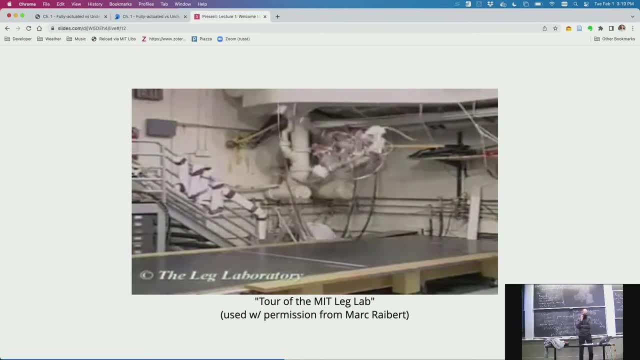 This is the the best, I think 3d backflip, And now you know when. when they did that backflip at Boston dynamics more recently, that was just a direct callback to these old videos. Okay, So good. 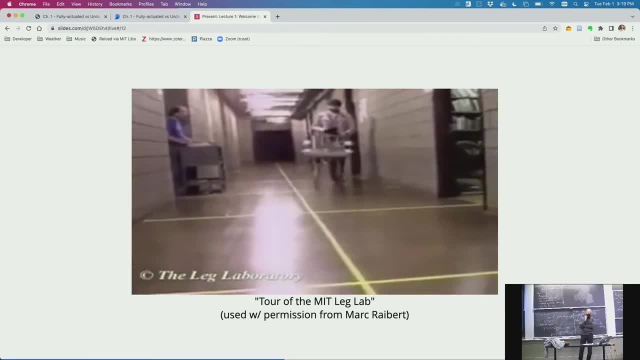 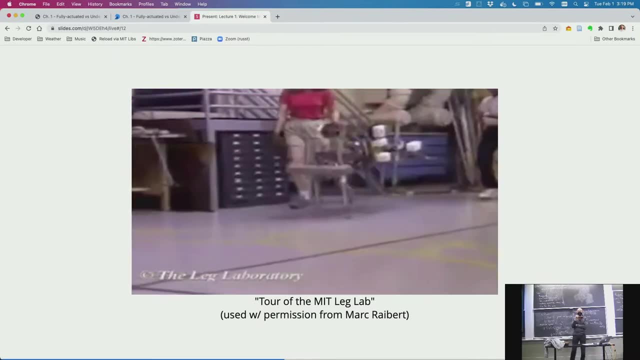 I actually see this is the early versions of the quadrupeds I was even in. I was sitting in the leg lab the day that Mark Rayburn came back and sort of he had- or he had already- stopped to stop being a professor to start Boston dynamics. 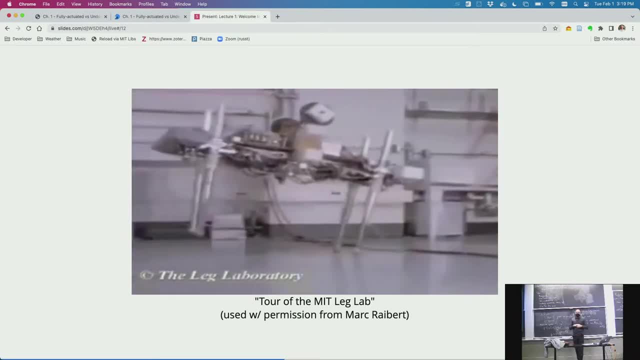 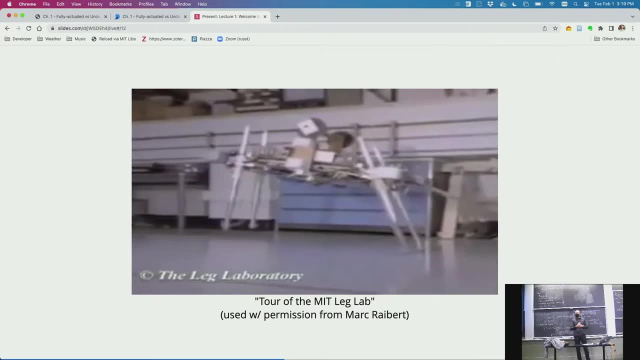 as a simulation company actually down the street, And he came by one day and he said, um, he looked at this old robot or this old treadmill that was lying there And he said: is that being used heavily, Is it, you know? 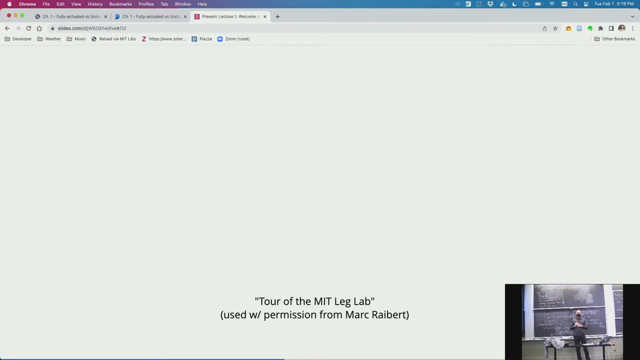 is there a chance we could get that back, Cause we're thinking about building robots again at Boston dynamics. So, um, and the rest, I guess, is history, but you have to understand that how different that was to have robots that are, you know. 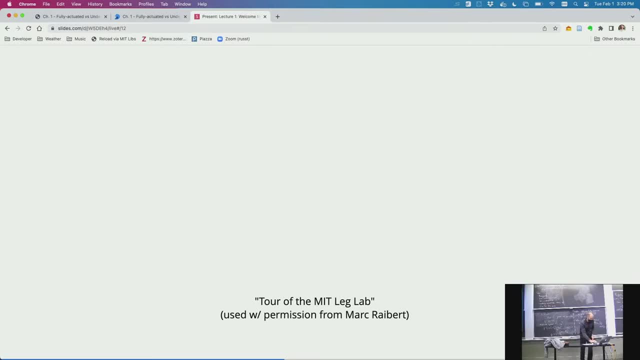 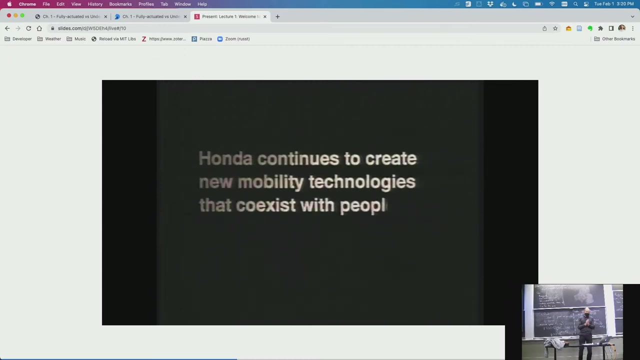 not trying to cancel out their dynamics, but throwing themselves through the air. Okay, And the. the example that made that stick for me, that has such a dramatic influence on my thinking, I think, was the contrast between Honda's Asimo, which was just this, absolutely incredible technology. 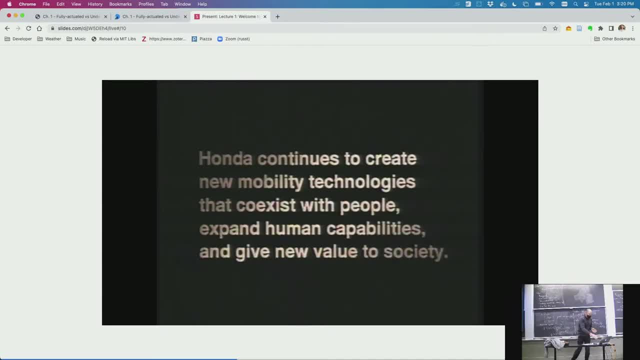 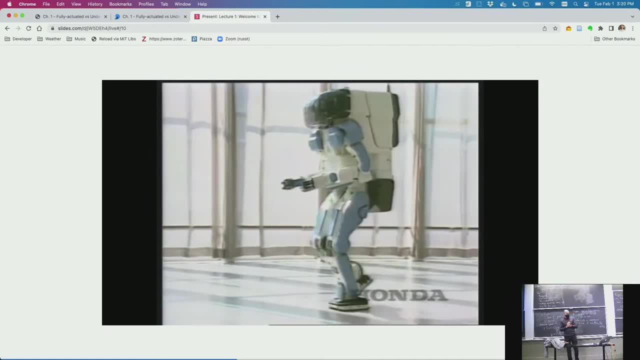 Similarly, this came out in 1997.. The first- this is actually P two- is the first version of this. I was in the Lego lab the day that's that Honda actually stopped by the leg lab to tell us about this, just before they announced it. 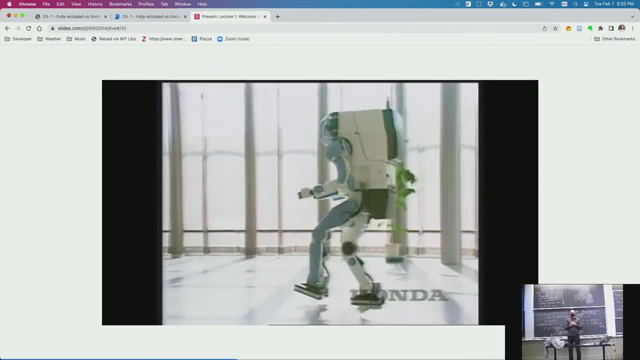 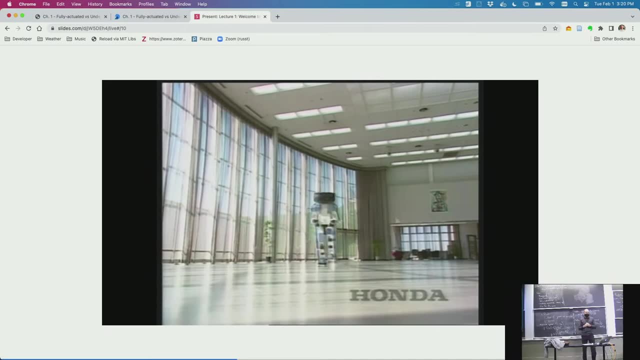 And that was one of those moments where we all looked at each other like, Oh crap, Uh, you know? um, there was a. this one came out just before I arrived at MIT, but there was a. there was a second one, that 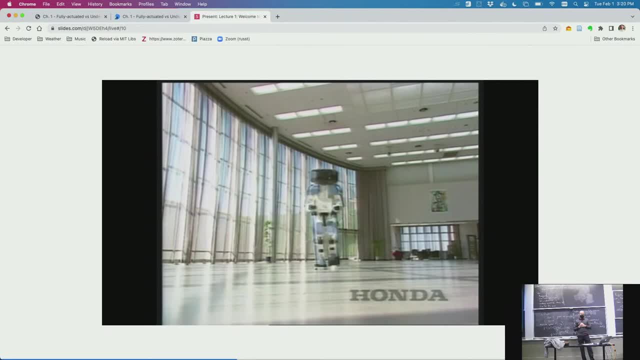 that even just rocked, rocked our world when we, when we saw the preview of it. Okay, But still, this looks very stiff, very rigid, right, We'll understand exactly the assumptions that are there. It's not trying to keep its center of mass directly over its support polygon. 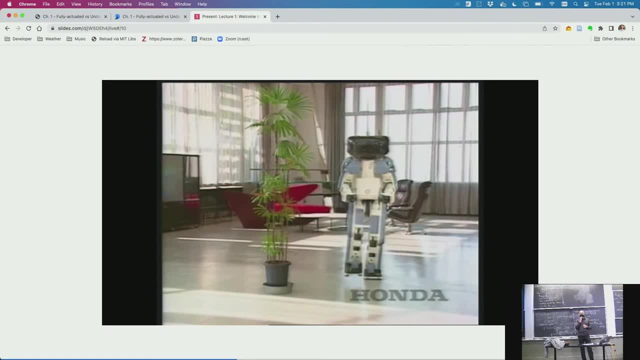 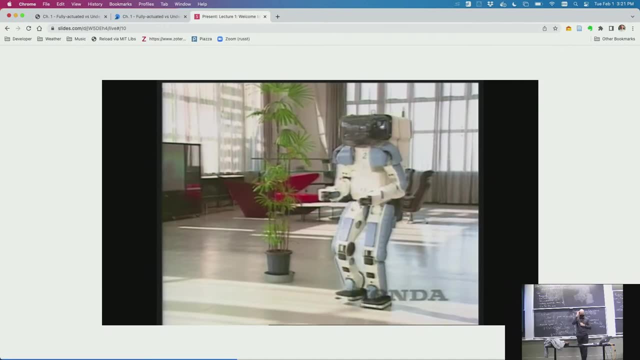 It's doing something smarter than that, but it's still fighting its dynamics in a big way. It's using a lot of power and it pays a huge efficiency penalty for for for doing control in that sort of way where you're trying to fight against your 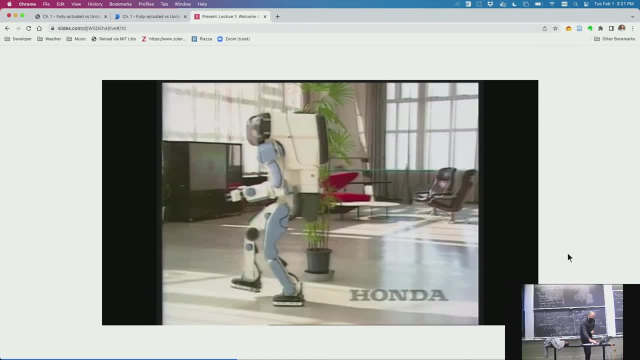 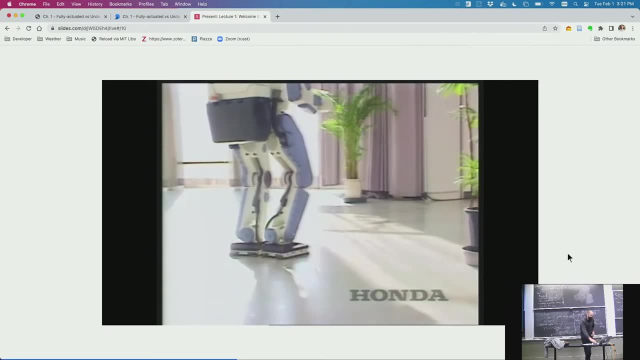 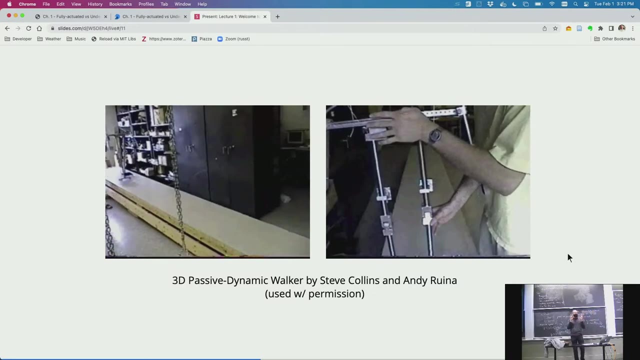 dynamics And then around the same time, like when Mark was doing making hopping robots fly around. there was someone in the late eighties, early nineties, named Tad McGeer that started a different line of work on passive dynamic walking. 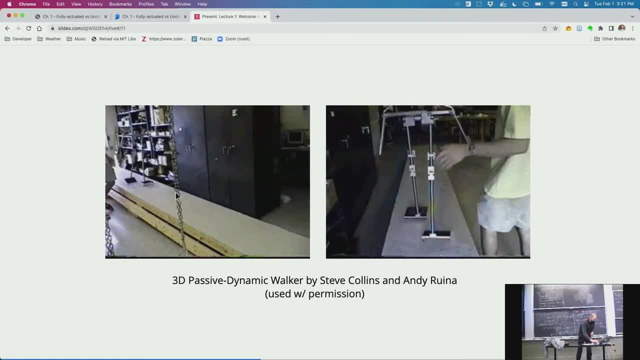 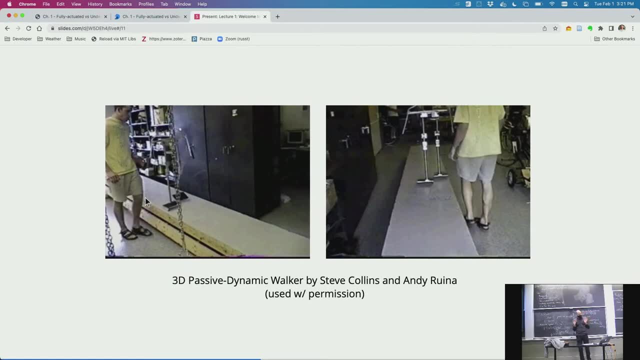 Okay, So passive dynamic walking. these are playing very badly, but these are walking robots that have no motors, no controllers, no things like that. So you put them. they're basically little slinkies, right, You put them on the top of a ramp. 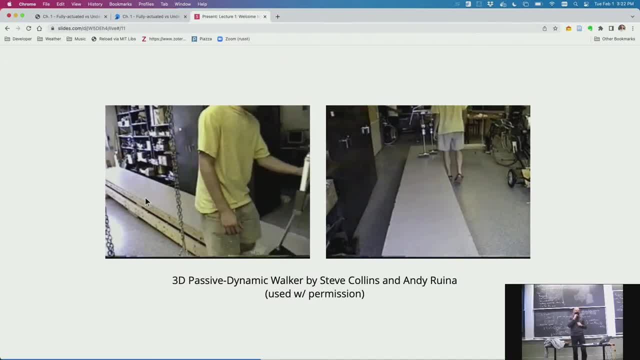 you give them a little push and they just fall down the ramp, powered only by gravity. It's sad that the most visually stunning video played a terrible frame rate. Okay, So, basically everybody who saw this, this was an extension of the of the 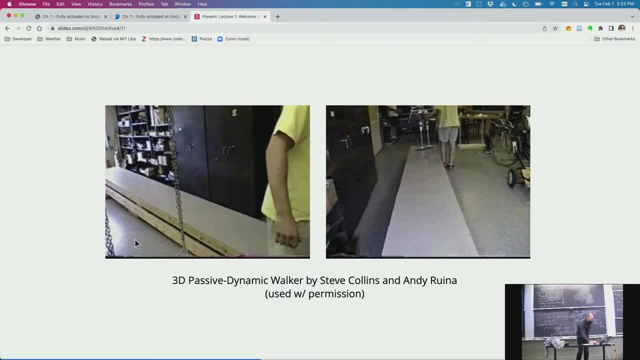 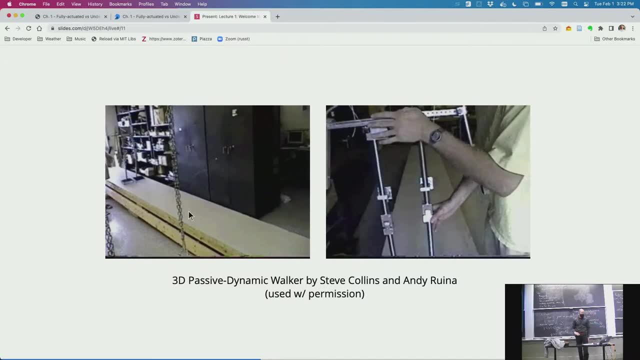 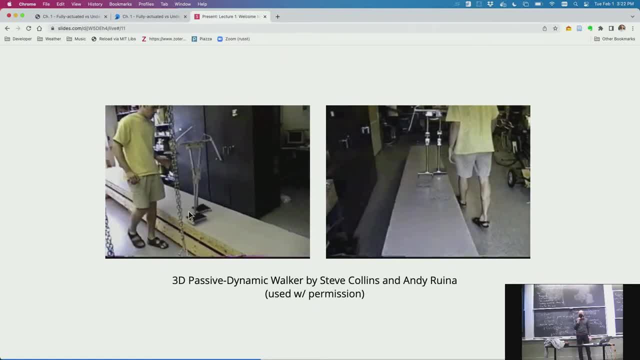 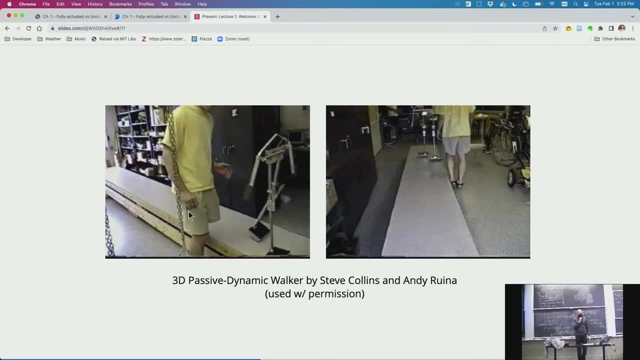 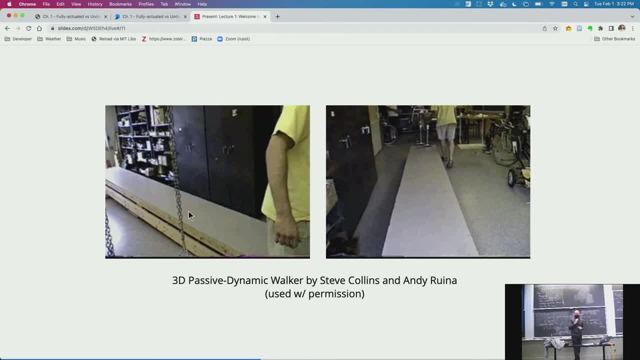 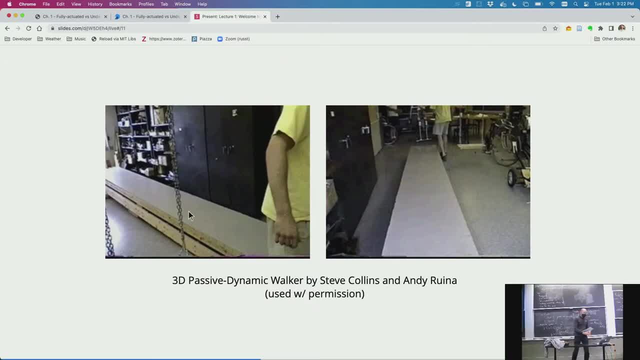 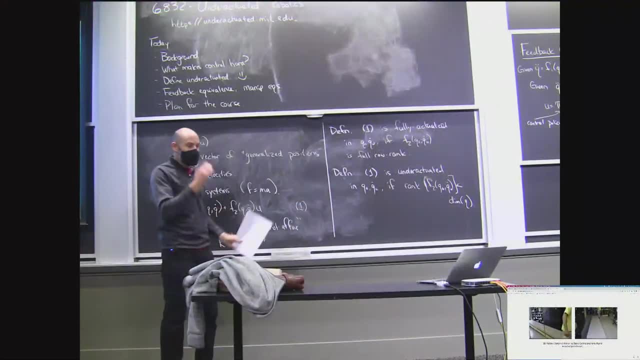 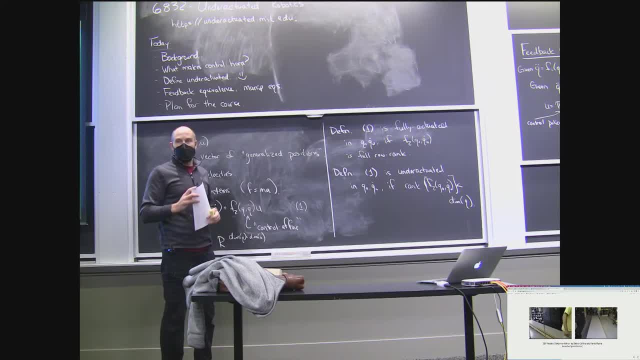 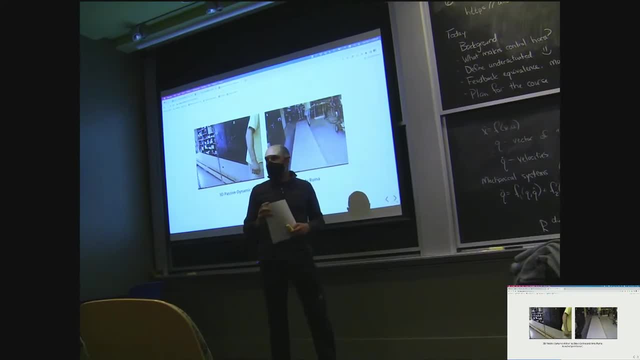 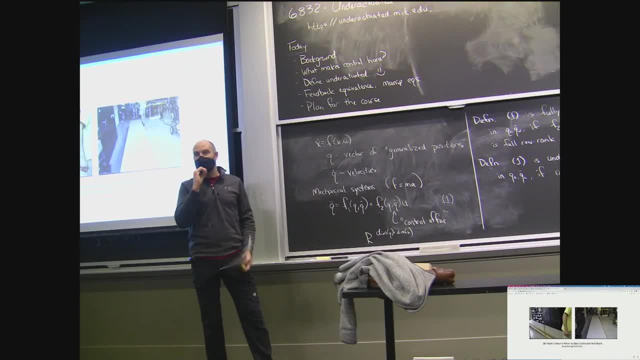 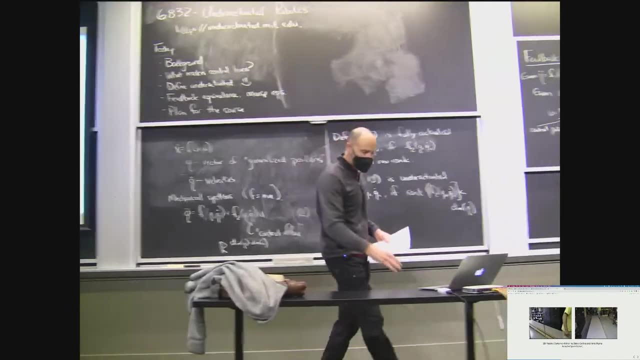 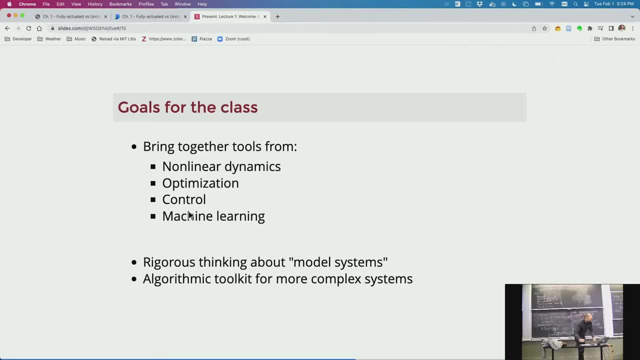 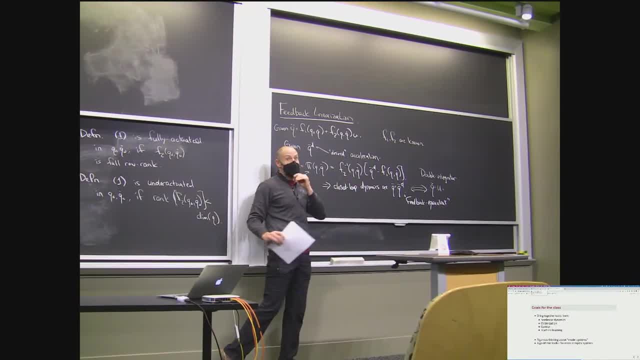 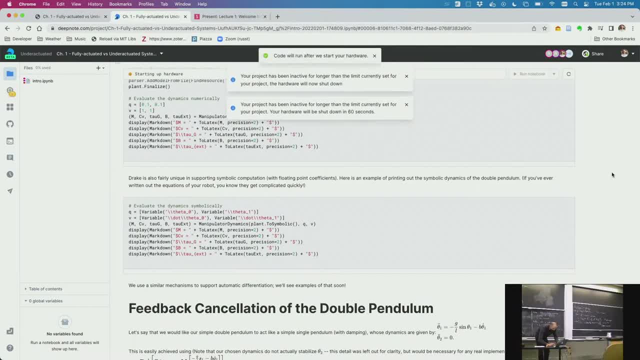 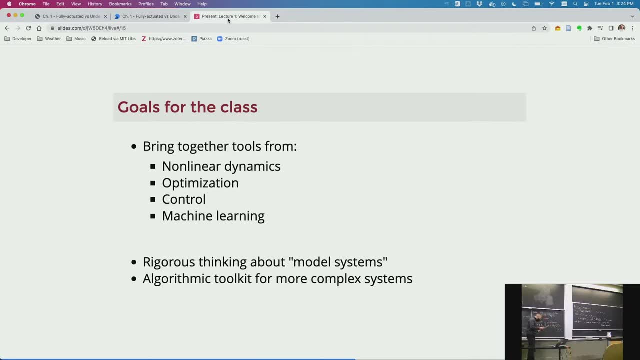 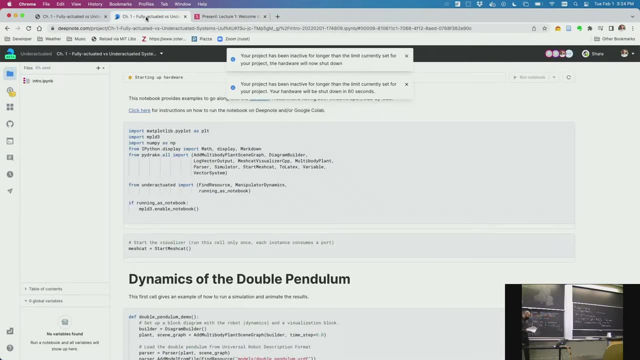 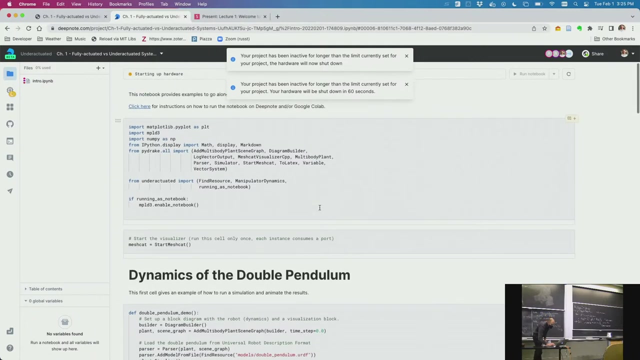 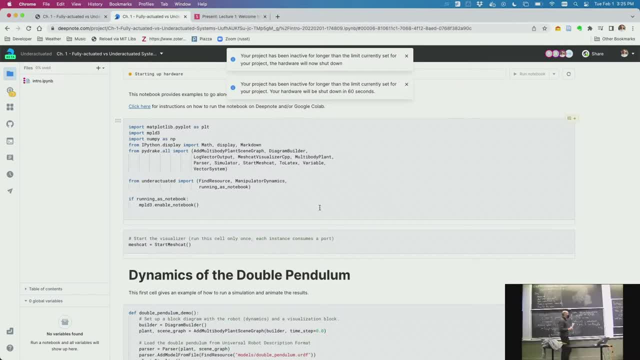 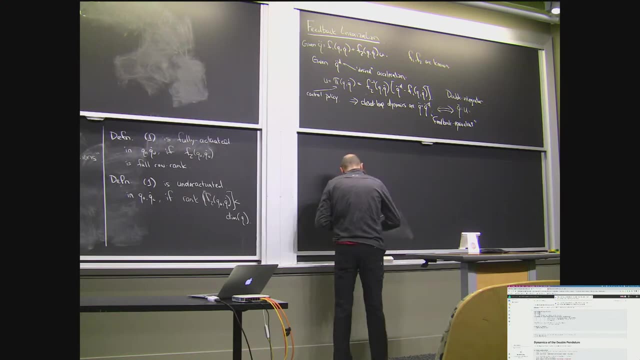 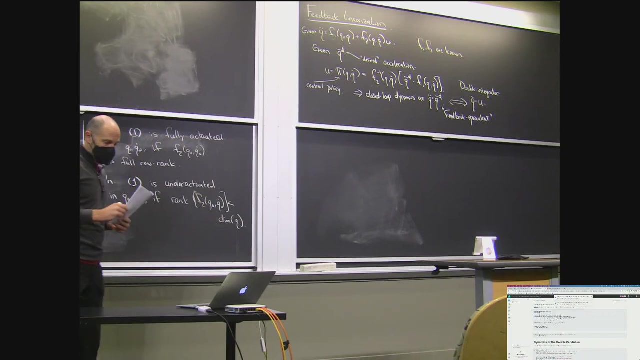 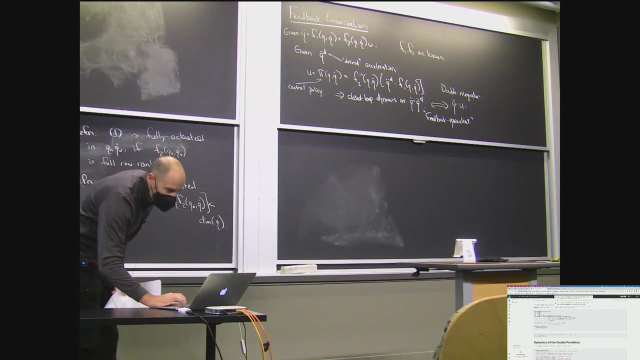 My claim is that robots that, basically, are canceling their dynamics are bad. Robots that aren't are good. I've got a demo that will load slowly when it plays. Let me think about how to take this home. OK, I'll just go from here. 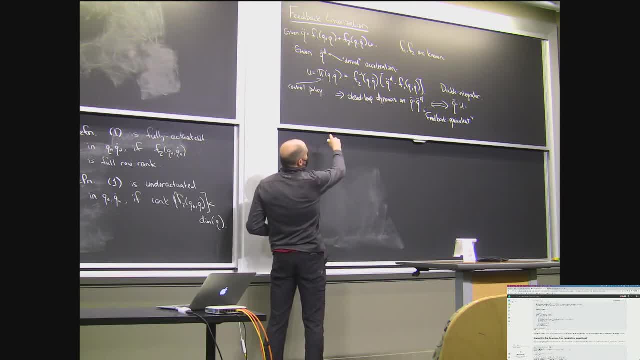 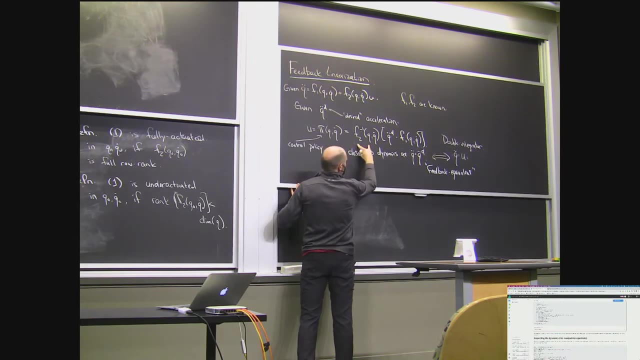 So do people understand? I guess people understand that basic definition. There are a handful of things that can complicate this. F being invertible is sort of the mathematical one that we've used, But there are other problems that can come into play. 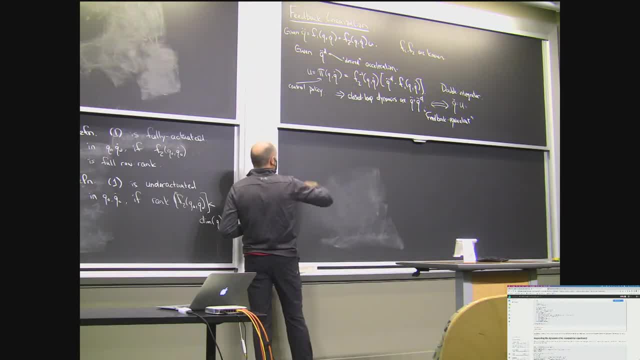 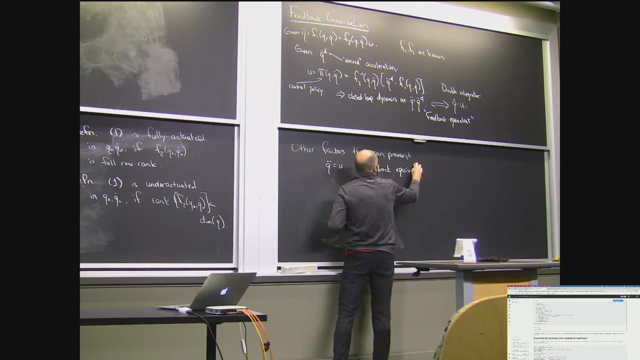 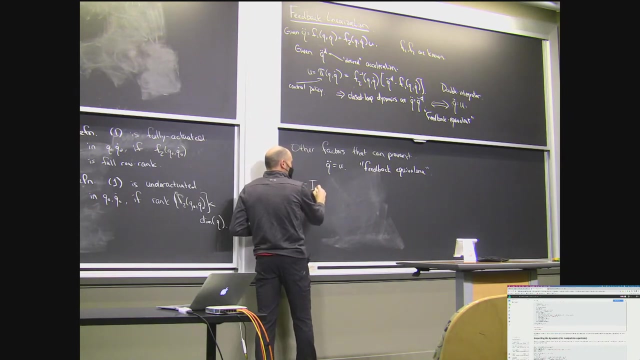 So Atlas has a lot of power, But still there are other factors that can prevent q double dot equal to u feedback equivalence. Those include, for instance, input limits. So if you have some limit in the amount of torque you can produce, 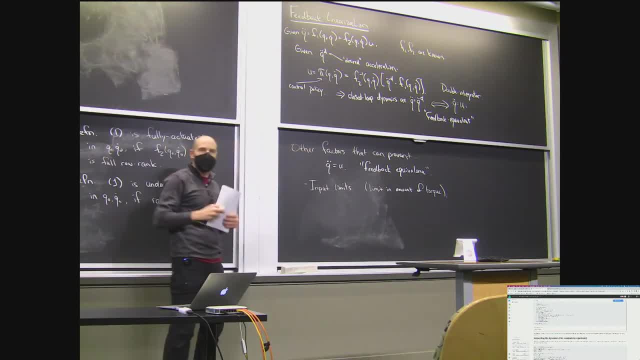 It used to be: we worried, We had a lot about that. We would constantly be up against our actuator limits. It's been interesting in a lot of the robots, In quadrotors for instance. quadrotors got really good when outrunner motors got powerful. 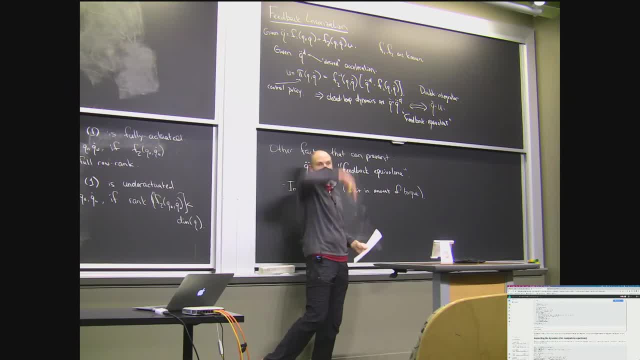 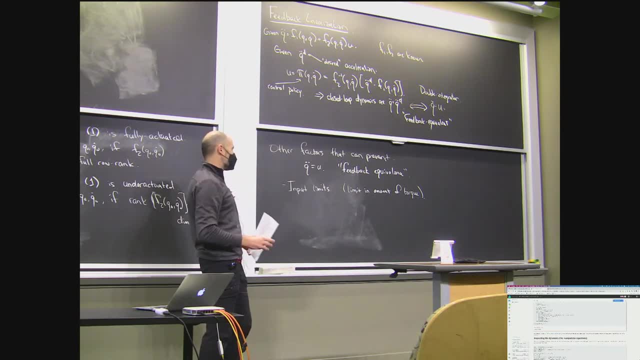 And we didn't have to worry so much about torque limits, And we have quadrotors that can produce multiples of their total mass in torque. Atlas got amazing, Spot got amazing. Spot got amazing when their torques got very large too. 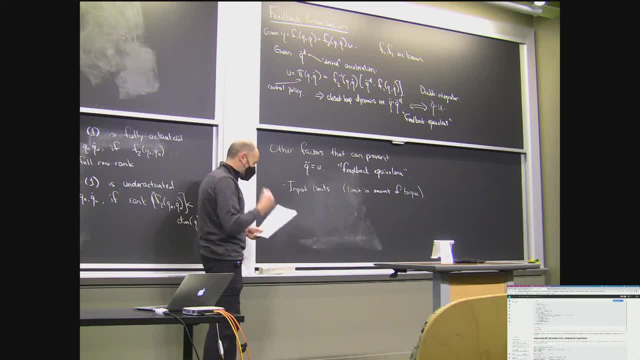 But if you do have input limits, power limits, that can be a big complexity. Sometimes you have state constraints that can get in the way. They could be joint limits, Collision avoidance. things can make things a lot harder. It means you can't just think about it as a linear system. 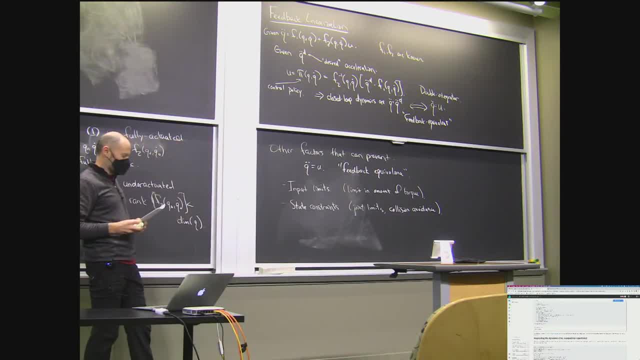 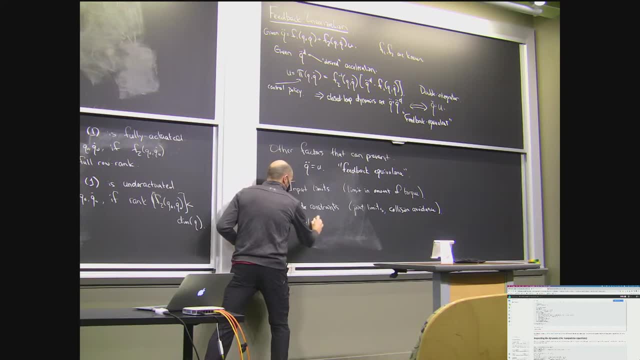 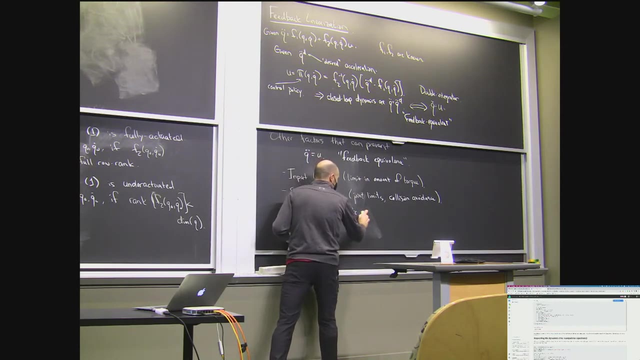 and assume things are going to go along. And then I think, other things that we mentioned on our list, model uncertainty, et cetera. OK, These all play in, But the fundamental concept of underactuated, which is, I think, 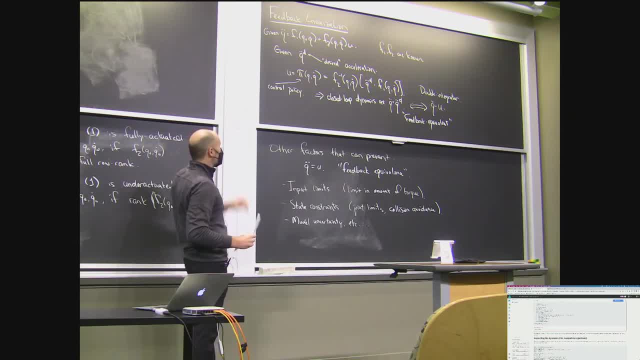 robotics. and this idea, this definition of underactuated and the slightly generalized version of the definition I give you in the text, is the question of whether I can, at an arbitrary instant in time, look at the state of my robot and command effectively. 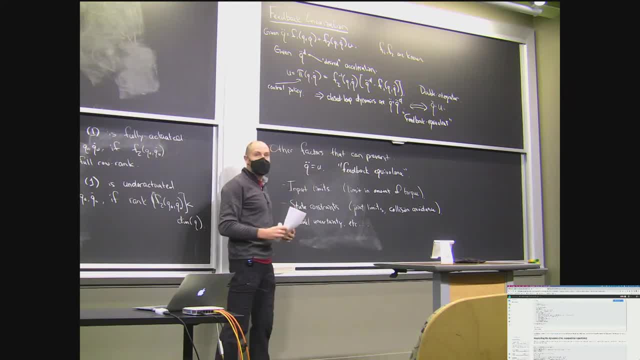 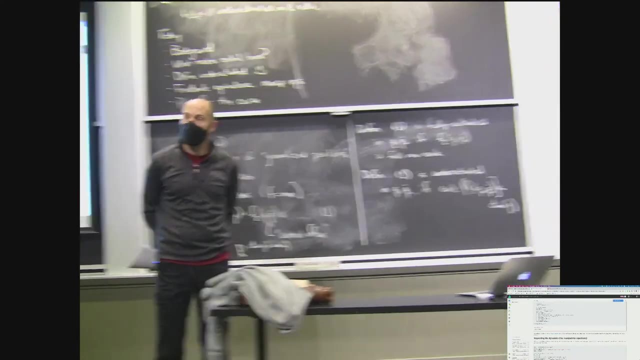 an arbitrary acceleration, If I can, then my claim is: the control gets easy again, And that's why robotic arms in factories are able to move incredibly well, But walking is a lot harder. Yes, So this is a robot. Does it feel like all the inputs are on the real number line? 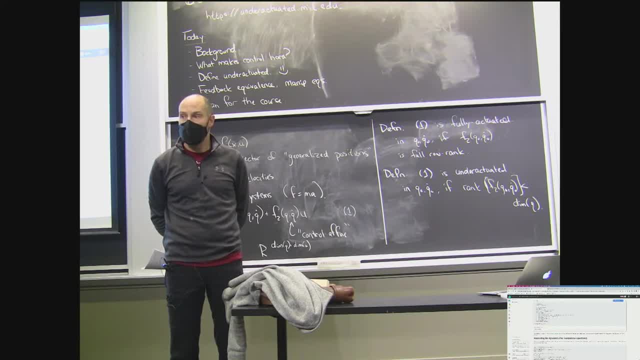 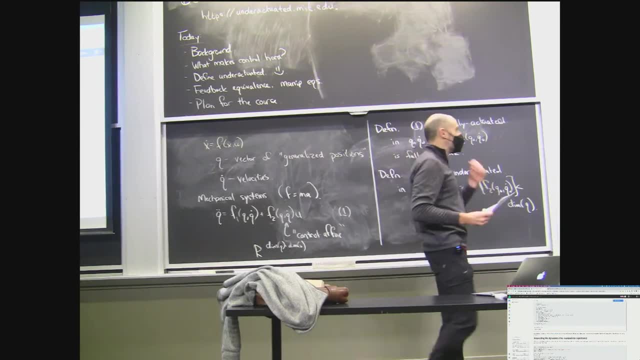 What about inputs that are maybe binary, so like a piston or something that has some discrete consequences? Yeah, that's awesome. So yeah, the question was what happens if I've been taking for granted that u is a real valued input, And what happens if you have discrete inputs? 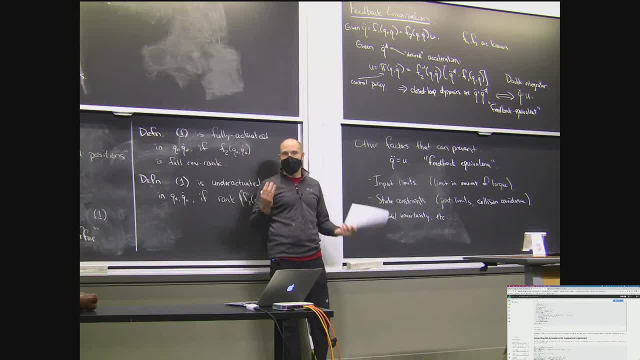 like a stepper motor or some other. you could imagine mechanical analogs. You can definitely treat that In some cases discrete states Or discrete inputs are easier, But actually in mechanics I think the structure is more beautiful if things are real valued. 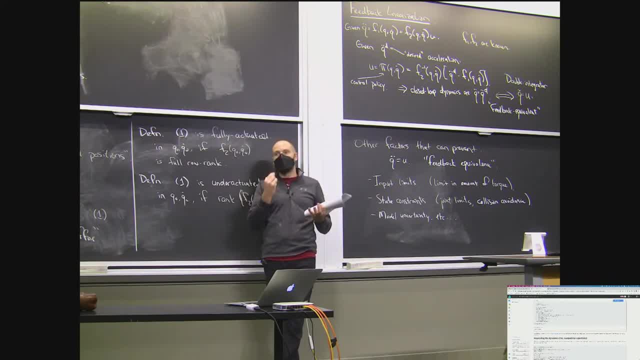 So we're going to spend most of our and most of our actuators are real valued. I think you'll see a lot of the math and the optimizations can grow in that direction, But we're going to go in and focus on the real value. 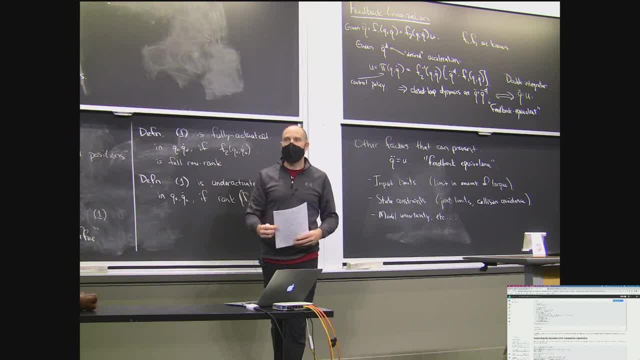 That's where the structure of the equations shines. At some point, if you have discrete numbers of u, then you kind of have to do a discrete search. There's no way to connect to see from one possible discrete action to another, Whereas if you have a continuous thing, 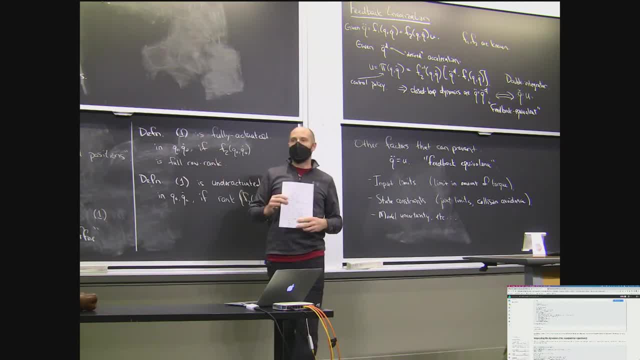 then you can write closed form solutions. You can write beautiful optimizations. Yeah, there was another question. When you write two double dot equals u, is that just a way of saying you can control acceleration to do whatever you want, Because right before you also have u equals the policy. 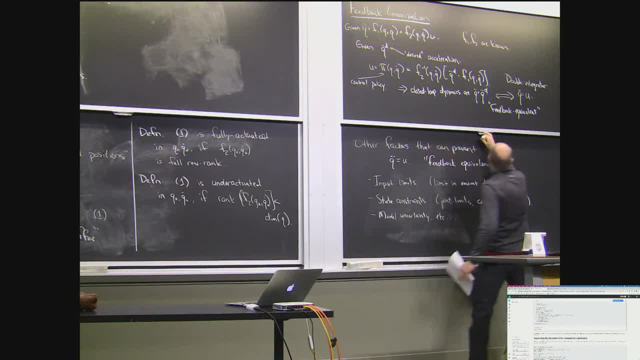 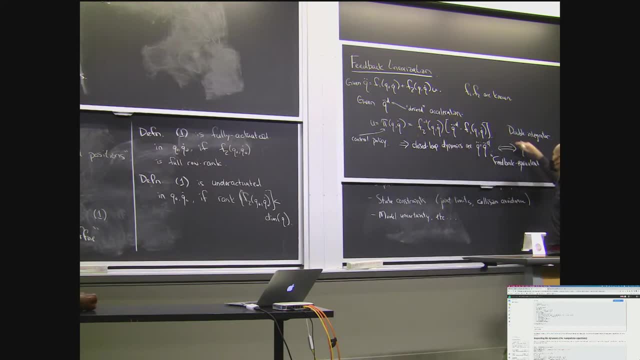 it's a bigger way. Good, So I want to. I'm sorry, I'm sorry, I almost called this v, just to keep that separate. So I'm just saying that you could think of it as a different system, System two here, which was like this: 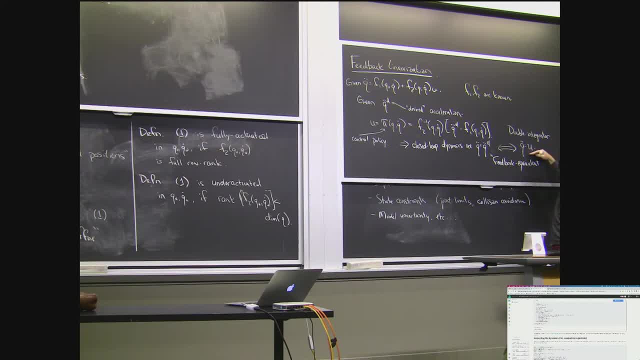 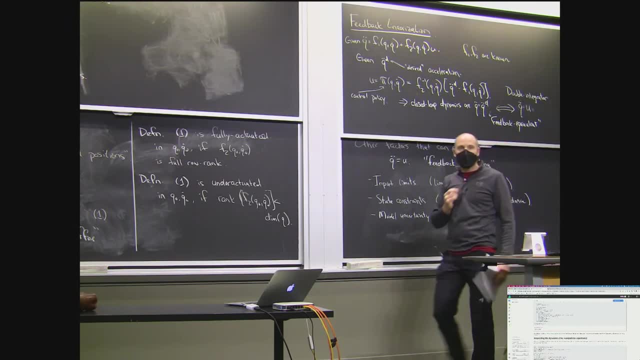 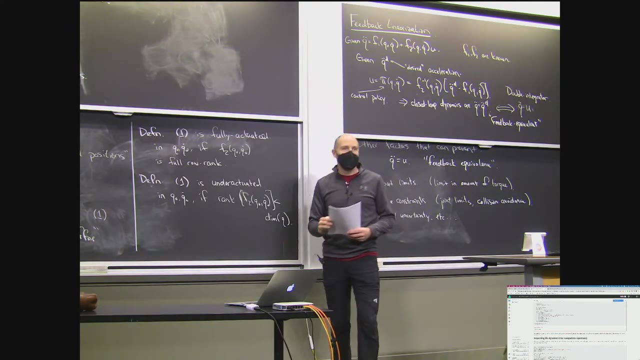 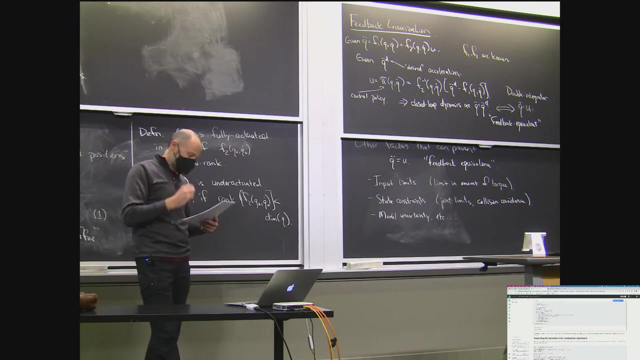 This is not the same u as that. I could think of it as a different virtual command input u. that's different. Yeah, That question was hopefully self-evident in the answer, But it was good OK. So let's think about how this plays out for robots. 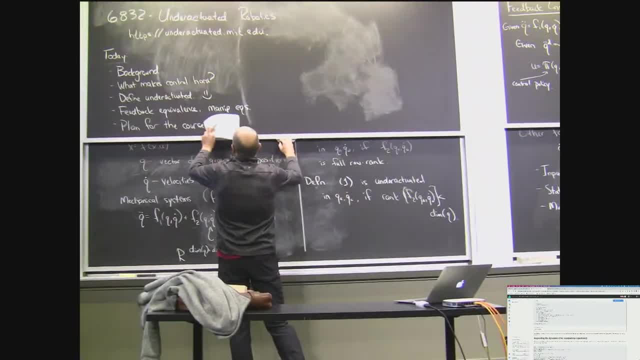 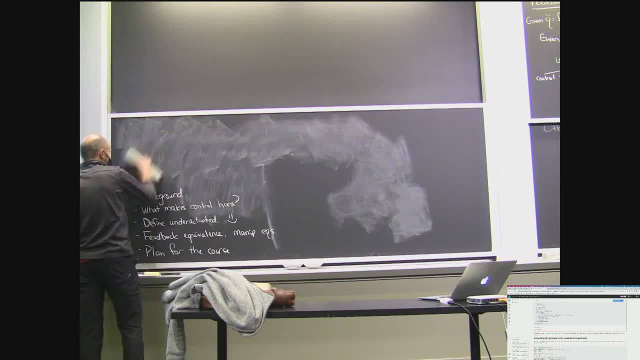 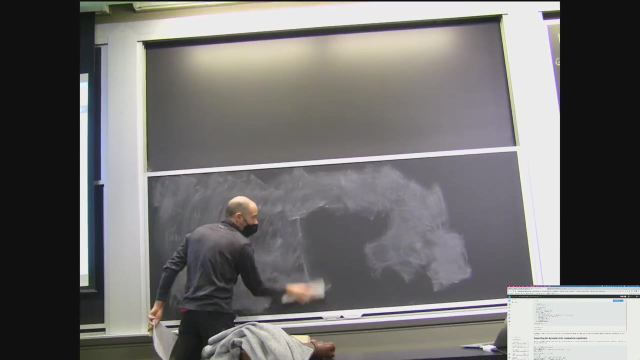 Let me show you the manipulator equations for a robot And I'll give you an example of it in just a second here. OK, So when I go and why do I choose real-valued u And why do I make all these control affine assumptions? 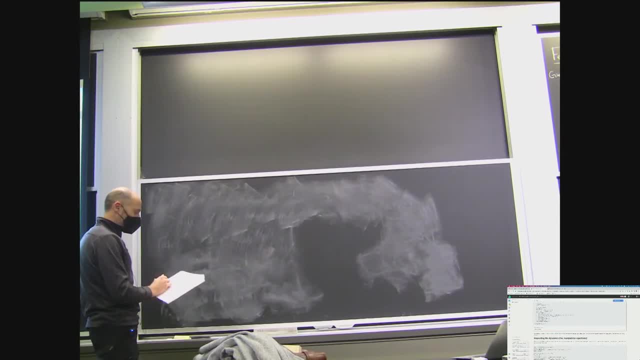 and everything like that. OK, OK, That comes from the equations of motion of our robots having a very specific form. OK, Now, what do you need to know to be successful in the class? You don't need to know how to derive equations of motion. 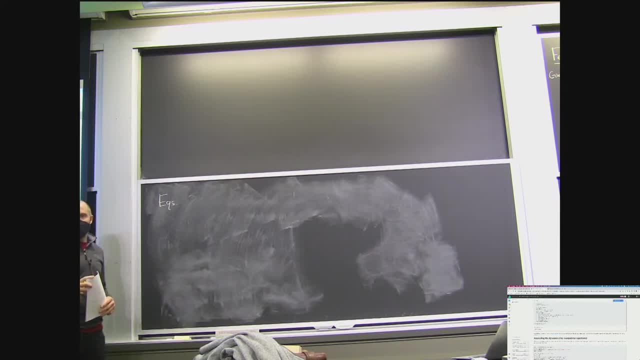 OK, You don't have to have a humanoid robot in your home. OK, I'm going to do a couple examples of this so you're familiar with it, And there's examples in the notes And there's software that will produce the equations. 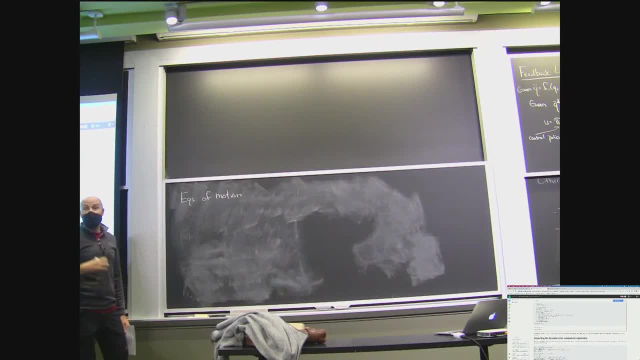 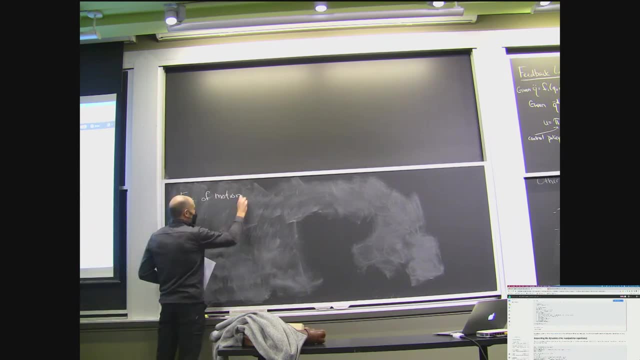 There's a lot of software out there that will produce the equations of motion for you these days, So you don't have to know that. But I want you to know the origin of it. I want you to know where these equations come from and appreciate the structure that emerges. 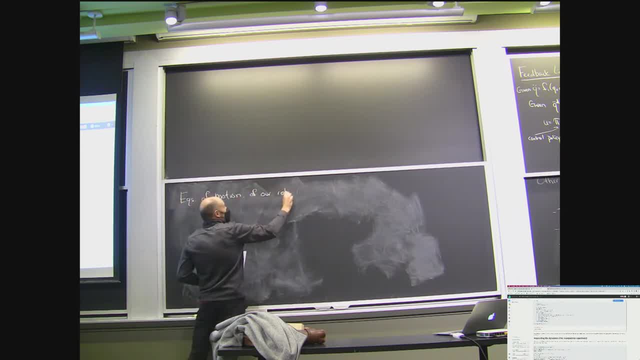 and sort of why it emerges. So the simplest way to do that is with kind of a simple pendulum or a double pendulum here. So let me make a two-link pendulum. I'm going to call this theta 1.. I'll call this relative angle theta 2.. 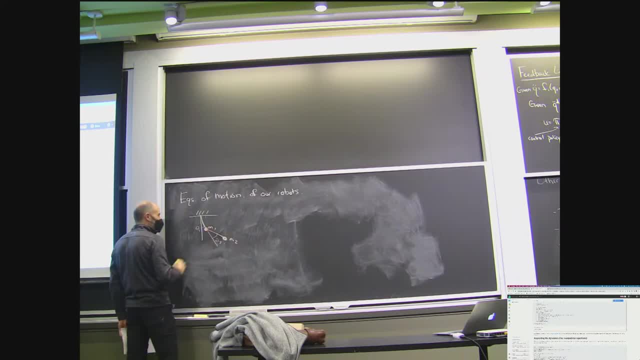 I'll call this mass 2, mass 1.. I've got some colored chalk here. I'll call this length 1 and length 2.. OK, Gravity pointing down. If you wanted to write a simulator to simulate that system, how do you start? 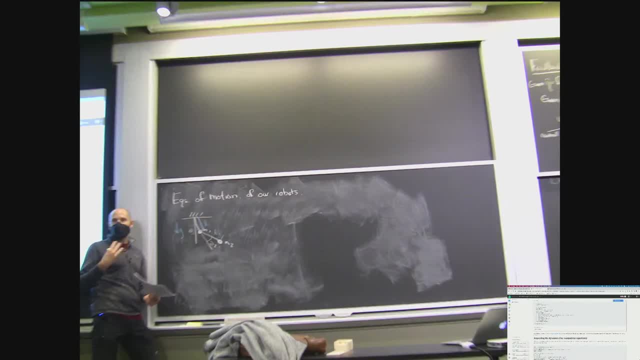 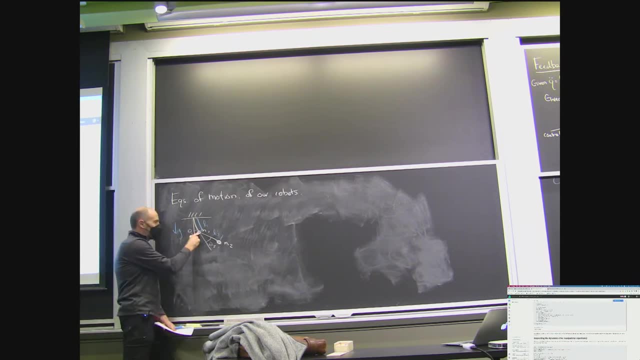 Many of you have done this in the past, But let me dust off the cobwebs if they're there. It's a simple recipe. I chose this. I drew it like this- because the simple version of this has just point masses at the end of each link. 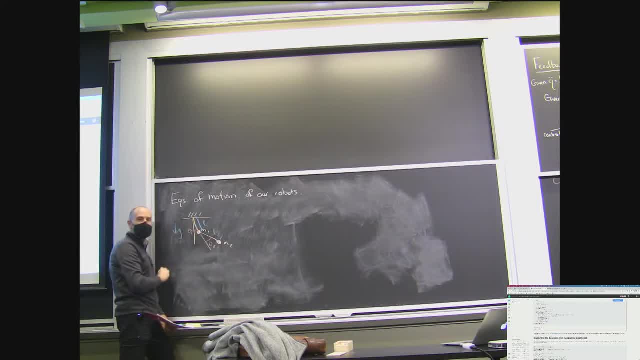 Of course there's a generalization of that, where you have mass along the extent of the link And you talk about moments of inertias and everything. But we can keep it super simple and still relevant. when you have point masses, OK, You need to write the total energy of the system. 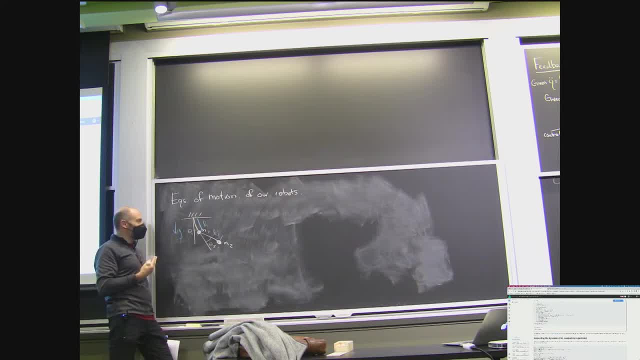 You need to write the potential energy of the system and the kinetic energy of the system. So the kinetic energy of the system is going to be 1 half mv squared plus 1 half mv squared. Potential energy is going to be mgh times. 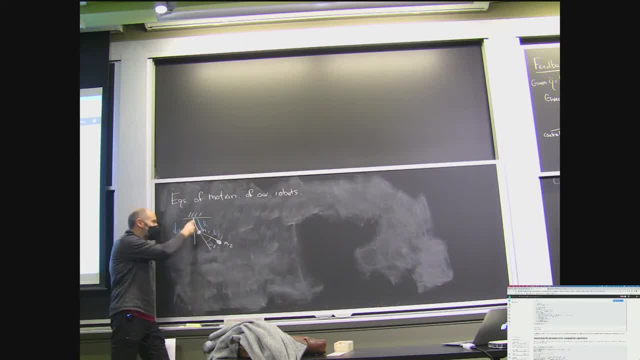 It's mgh plus mgh, right? So we need to figure out what the height of this is as a function of theta and theta 2.. And we need to figure out the velocity of that as a function of those variables and their derivatives. 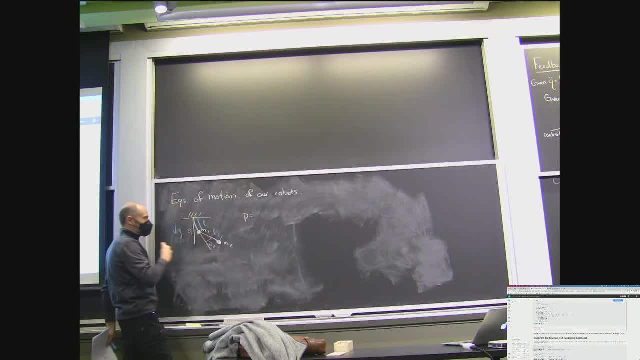 OK, And that's just kinematics And I'm not going to derive the whole thing, but I'll show you the basic form. So if this is length 1, this is theta, then my x position, This is the position of mass 1.. 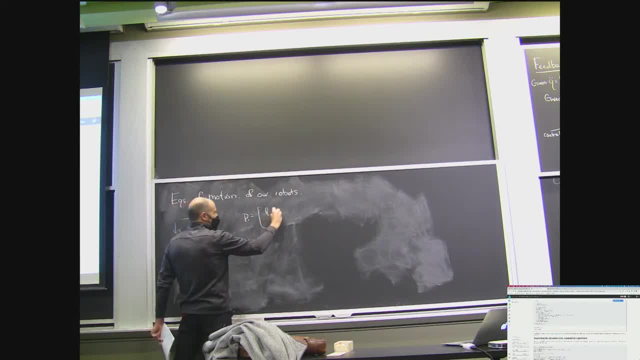 I'll call P1.. Would be L1 sine theta 1.. And then this would be minus L1 cosine theta 1.. You get a bunch of sines and cosines pretty fast. OK, P2 is just P1 plus L2 sine. 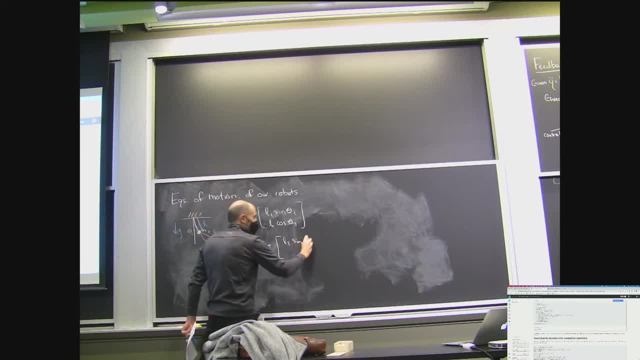 In the relative coordinates, you'll see that you get a theta 1 plus theta 2.. OK, OK, OK, That's enough to write your potential energy. It's just mass 1 times gravity, times this y value. That's the height. 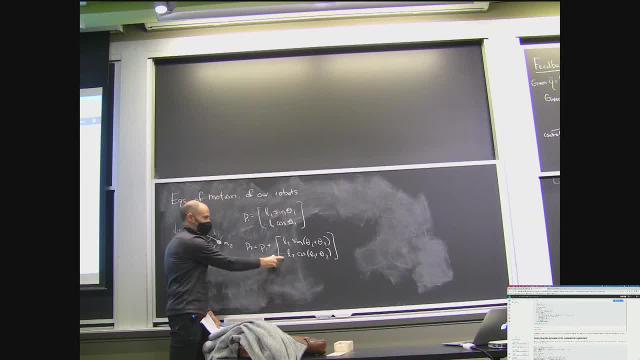 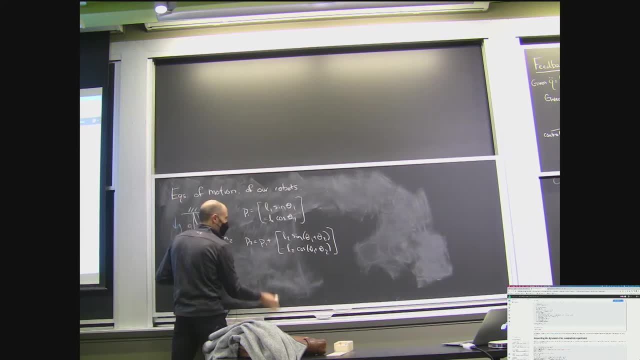 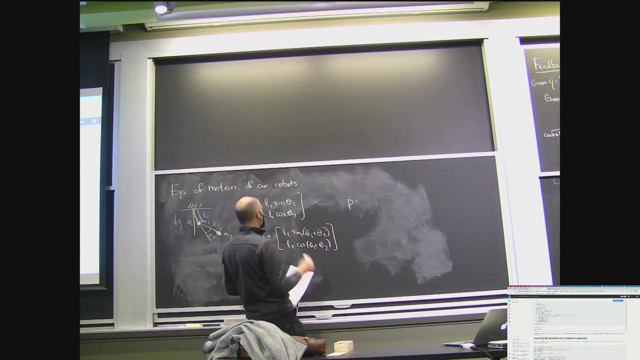 Plus the mass times, this of your second mass. That gives you your total potential. That gives you your total potential energy, The kinetic energy. you need the derivatives here. So you end up. you need the velocities of this Again. it's just going to be taking. 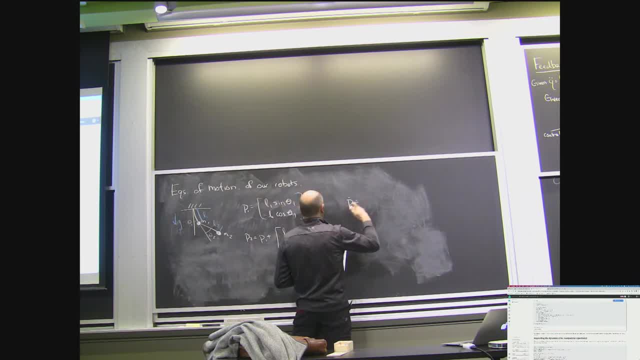 a gradient of a nonlinear function. here in vector form I'll get L1 theta dot sine theta 1. Right, And what I said, that wrong Cosine. theta Sine is cos right. And then L1 theta 1 dot. 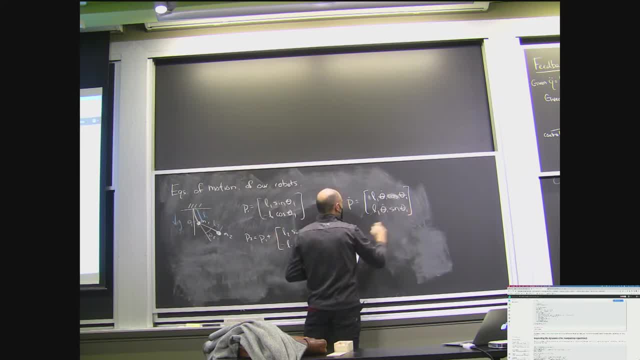 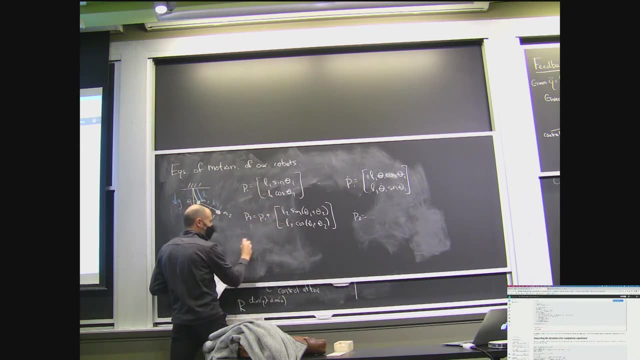 This was negative cosine theta, so just sine theta 1. I can do the same thing for P2 dot, but I won't. And then, if I've got this xy vector for the velocities, the vector form of the vector, OK. 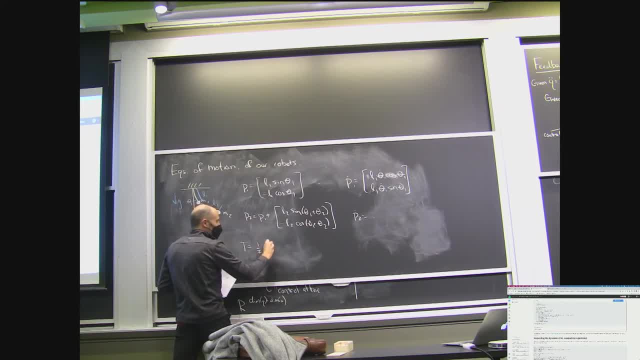 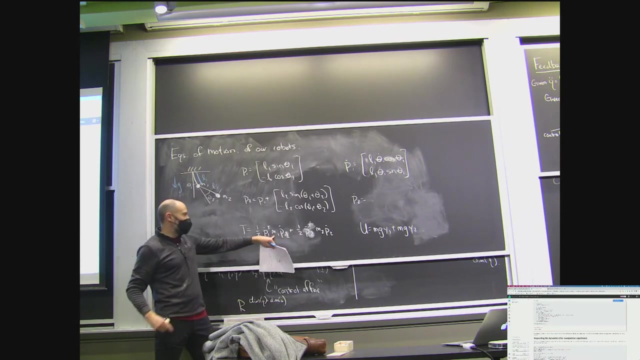 Total kinetic energy is just 1 half P dot 1. transpose times the mass, 1 P dot 1.. And u is just mg y1.. It looks a little funny to put my scalar mass in the middle of a dot product. It's not wrong, but I wanted to put it there. 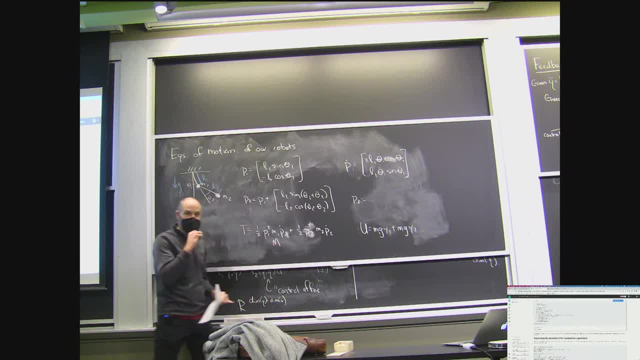 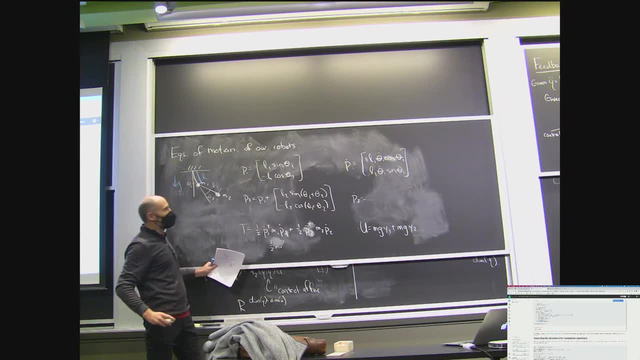 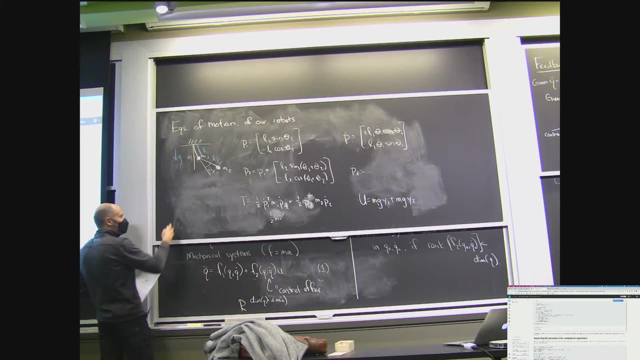 because there's going to be a generalization of that where that becomes a matrix mass. OK, But you can think of this as just 1 half mv squared. OK, It's just the. And then, If you guys know the Lagrangian, your Lagrangian mechanics. 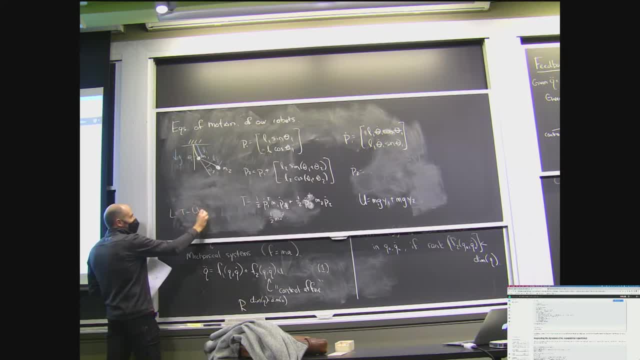 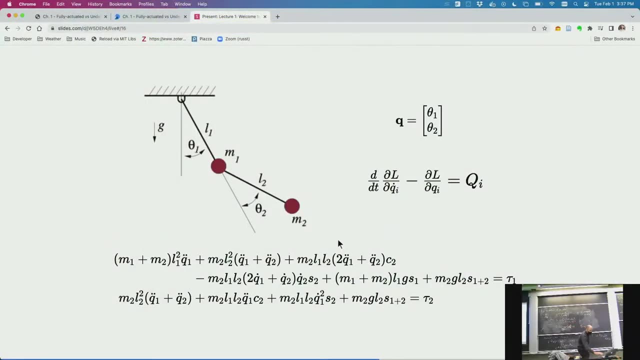 you plug this into your Lagrangian, you take some derivatives and you get your equations in motion. And if you turn the crank on that, you get this term that I have up on the screen here. OK, You turn the crank on that and you get some equations. 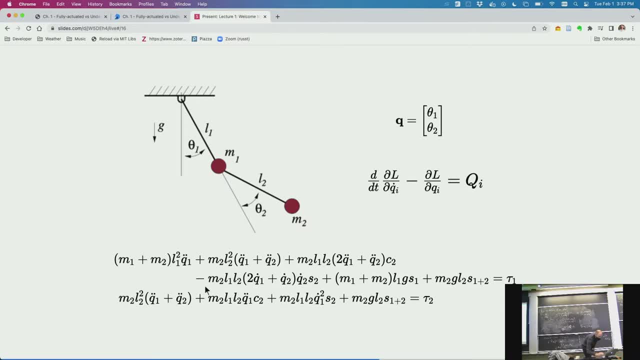 that look like this. OK, The exact form of it doesn't matter, but the structure of it matters greatly. Let me just make sure you see that I've substituted. I've used the shorthand c2 for cosine, theta 2 and sine and the like. 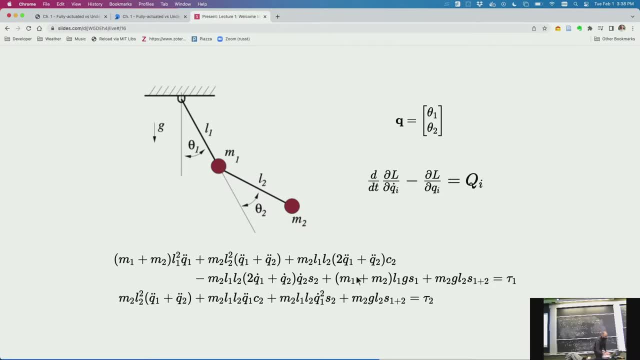 Sine: theta 1 plus theta 2.. So that's just shorthand. OK, Let's look at the structure of those equations. If you do this a bunch of times for a bunch of different robots, you'll see that there's always this very pronounced structure. 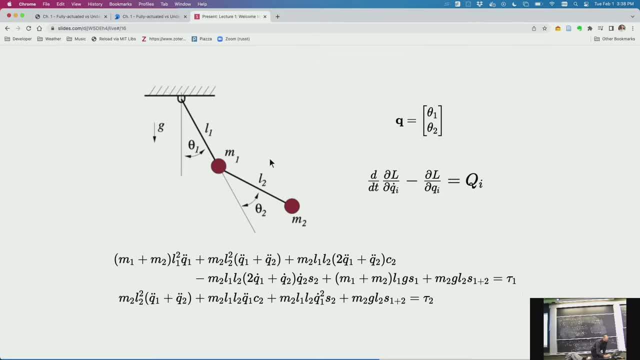 First of all, as I promised actually, if I were to put an extra torque here on the joints and plug that through the same equations, the torque always enters in this way, linearly, in these equations. OK, There's a q double dot on this side. 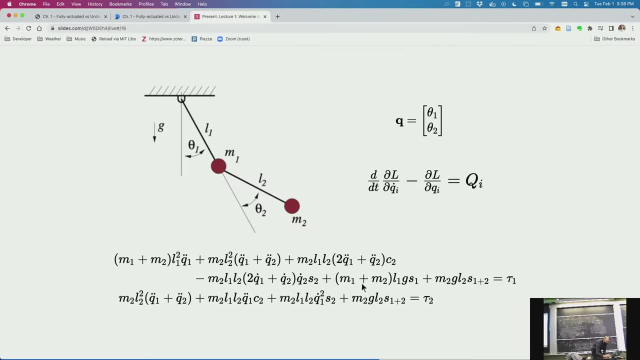 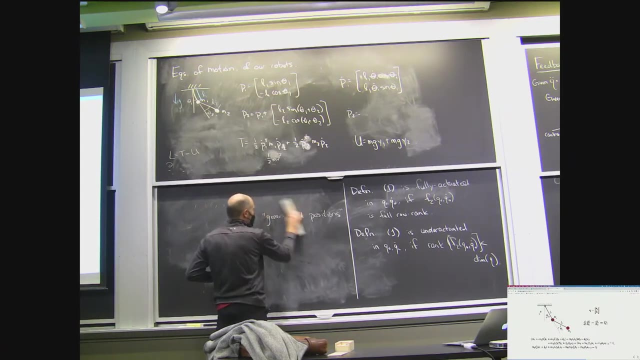 that has a big matrix on the front of it And it turns out. if you do this enough times, you'll see that there's this incredibly good general: general enough to describe our robots, but not so general that it doesn't have any structure. 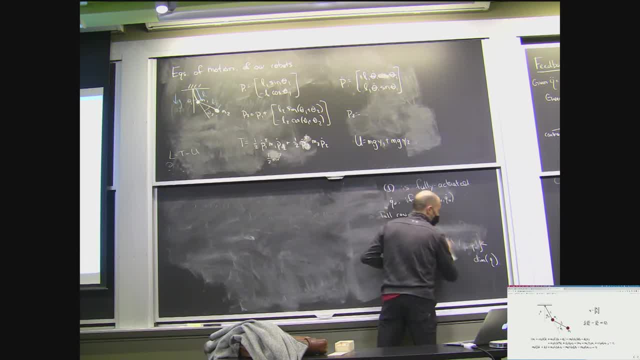 It's like a beautiful balance of you know describe the bunch, but still has structure where I can write all my robots, basically in this form where I have q double dot. Look at the q double dot times, some collection of terms which 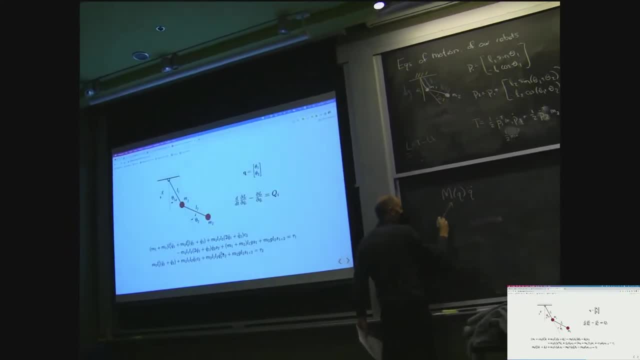 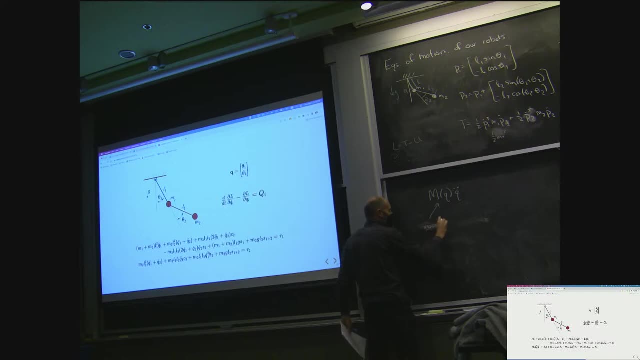 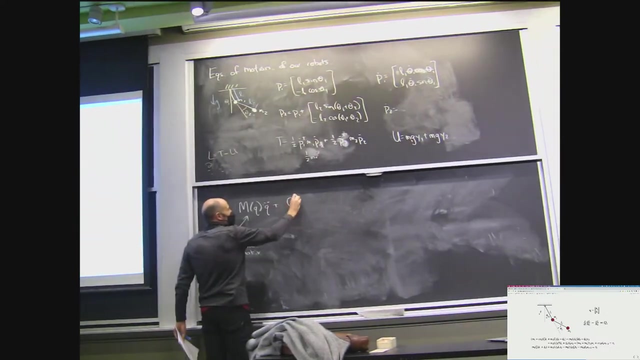 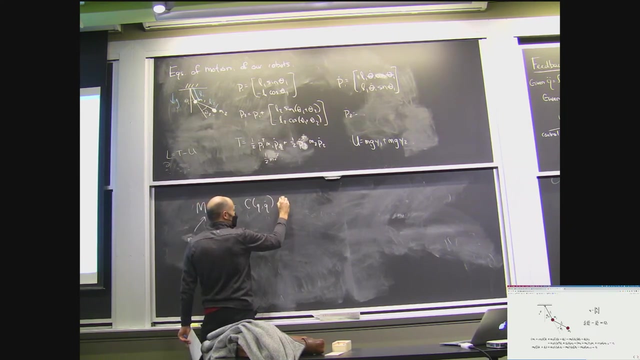 becomes a generalized mass matrix Or an inertial matrix, plus some collection of terms on the left-hand side. I'll leave it like that for the moment. We'll get more structure later. OK, We always have some gravity terms that come in. 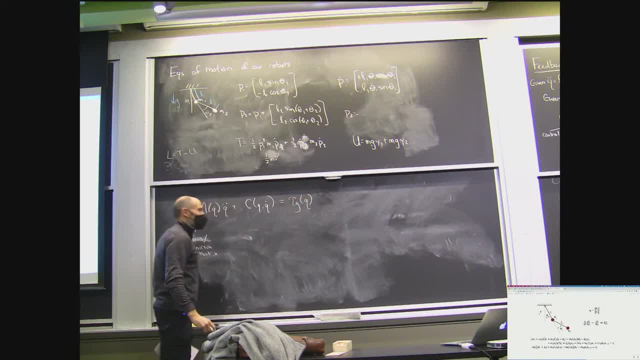 From the potential energy. They always just depend on q. You never have velocities in your gravity. So this is Coriolis terms, OK, And this is gravity terms. And then you have your control inputs- OK, And they come in looking like this: 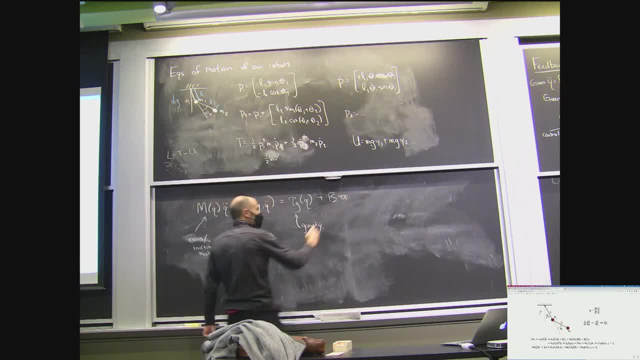 And you start from the very top, where this is almost always a constant actuation matrix And I could call these torque control inputs. Now if you have external forces or contact forces or other things coming in, you might have more terms coming off. 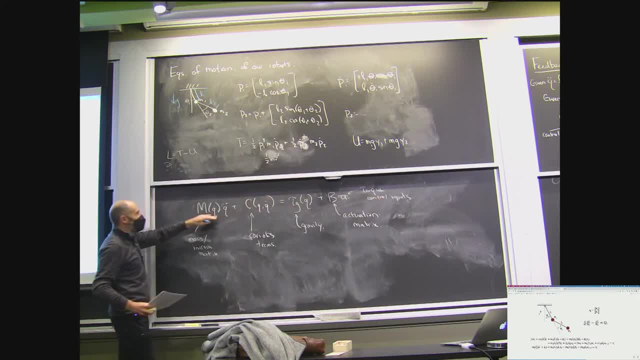 to the side. But this is the fundamental: f equals ma equation when you go through a Lagrangian derivation of the equations of motion and generalized coordinates And it's got even more structure than this, Like we could talk about the relationships between m and c. 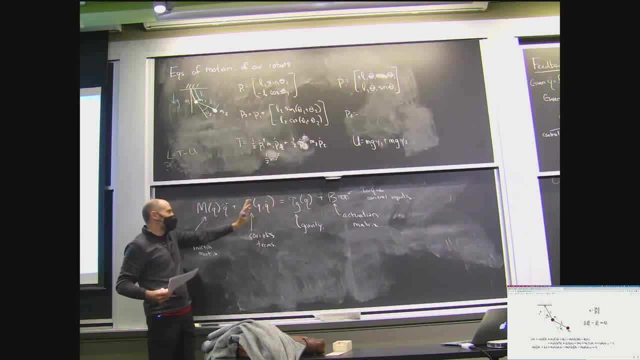 And c turns out to always be quadratic, and q dot, And there's all kinds of good things we know about these functions. The actuation matrix is interesting. OK, In the simple case, if I were to have an actuator both at the elbow and the shoulder. 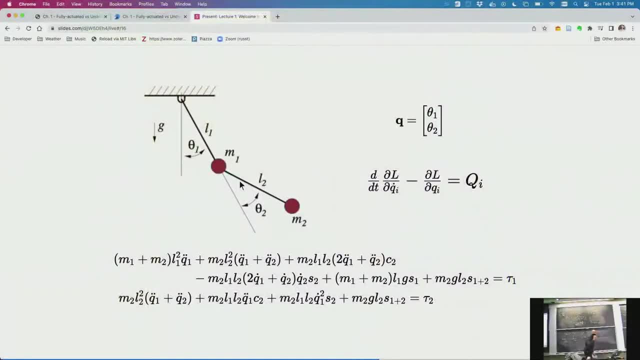 then the b would just be the identity matrix. That's the simple case. If I'm missing an actuator, then b might not be the full identity matrix. In fact, We'll think about systems, for instance, where b if I had only the actuator at the elbow. 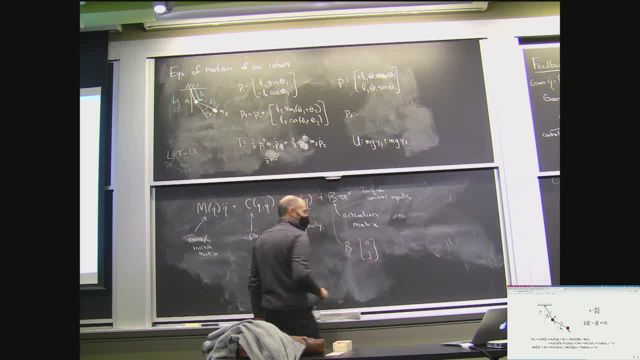 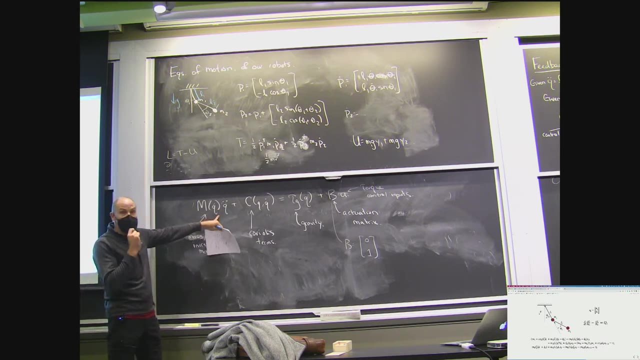 that's a famous system we'll talk about then. I would just have a b matrix that looks like this, that maps the elbow torque into the full coordinates. OK, How do we connect these equations, these beautiful manipulator equations that we'll use a lot throughout the class, with this basic definition? 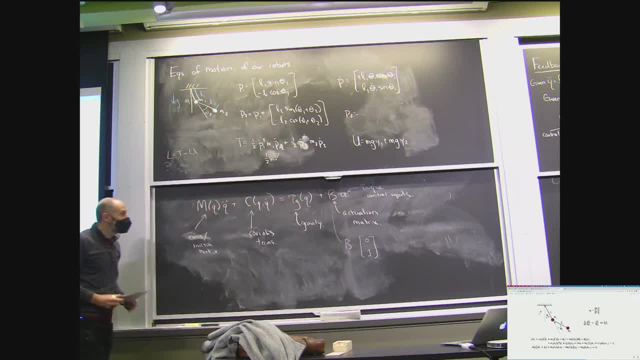 of underactuated and featureless. We'll talk about that in a little bit. But we'll talk about that in a little bit. But we'll talk about that in a little bit. And then we'll talk about the feedback equivalence. What are the conditions on this set of equations? 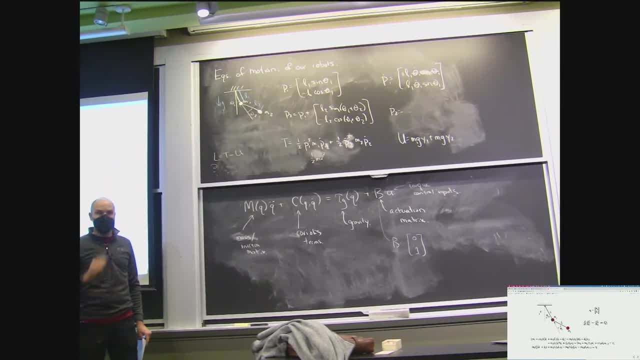 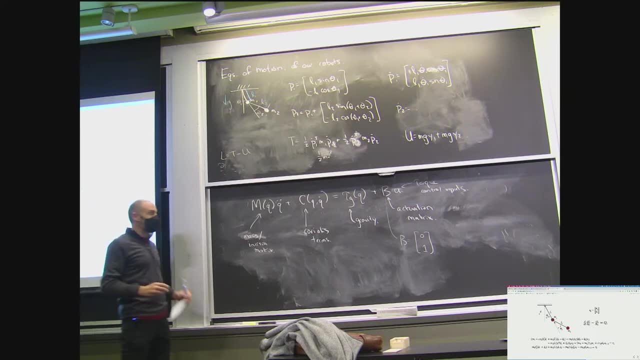 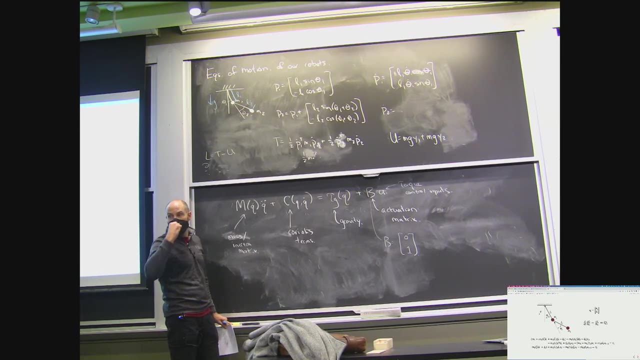 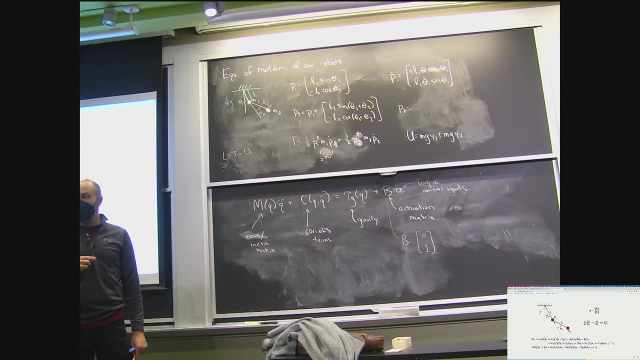 on my Lagrangian. OK, that would make a system fully actuated or underactuated. Yeah, Hold on one second. Can you just repeat the question? Yeah, You could just say. I think you could say the same thing about b, the actuation matrix. 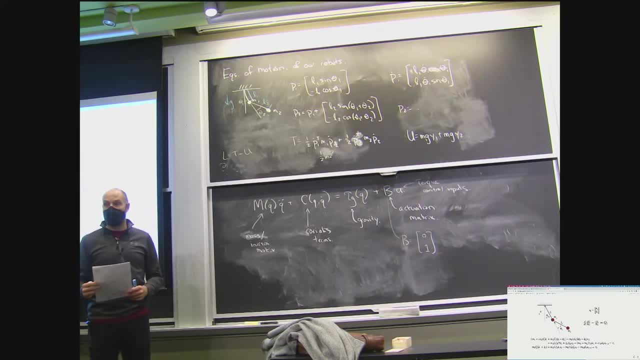 So if it's full row rank, then it would be fully actuated, I think OK. So the claim there was: if b is full row rank, then I'm going to be fully actuated, And that is absolutely correct. But there's a step of reasoning that you made there. 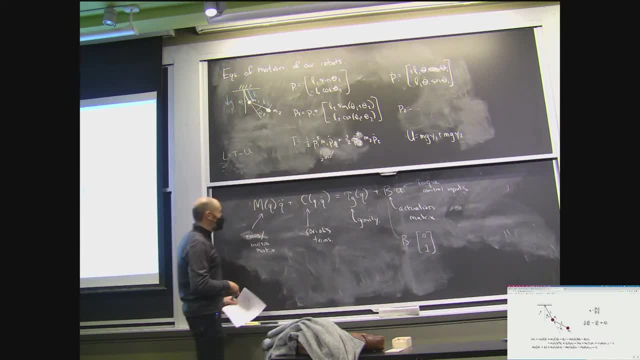 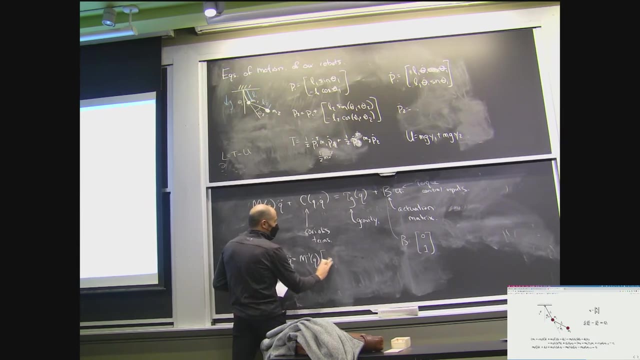 that is important for that to be true, which is that if I were to write this in the original form right that I used before, if I write it in this form, I have to take an m inverse on this other side: OK minus plus. 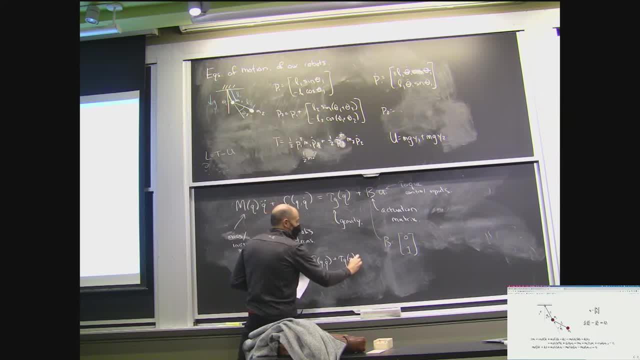 tau g, q plus b u. OK, In order to put it in the form we've already discussed: right, I have to take this mass matrix. I have to take this mass matrix inverse Every time you take an inverse in this class. 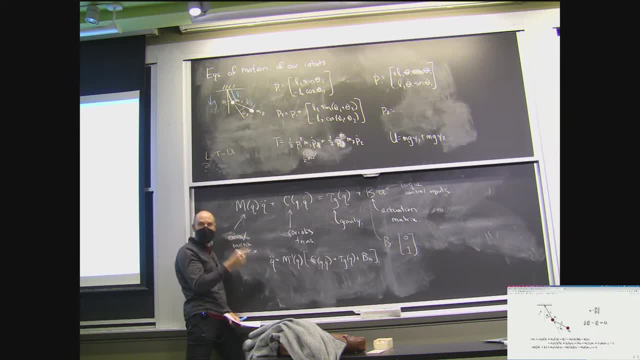 you should stop and think: am I allowed to take that inverse right? Does that always exist for all q's and for all robots in this case? OK, Luckily it does, And I will only at this point evoke your sort of physical intuition that mass is always positive. 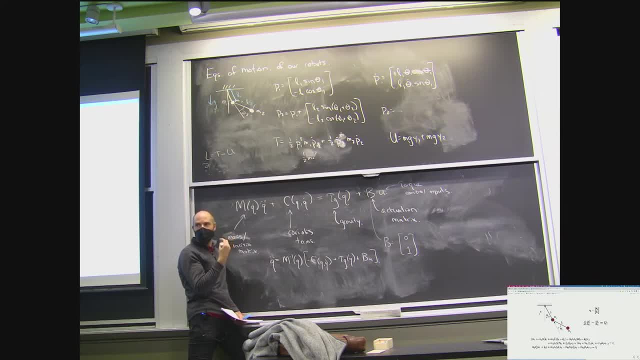 OK, This is a generalized mass matrix, but it does have nice invertibility properties In general. So every time you kick out the Lagrangian, you'll get some term here which is a generalized mass or inertial matrix, And mass is always positive. 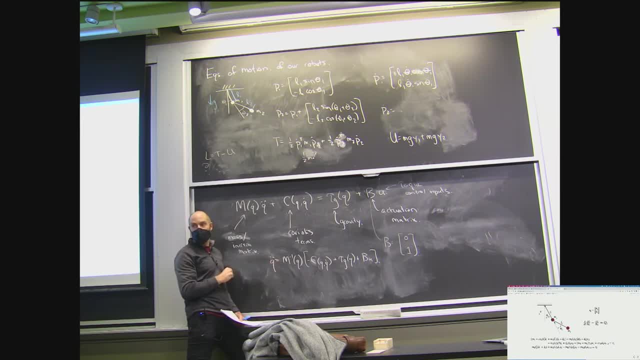 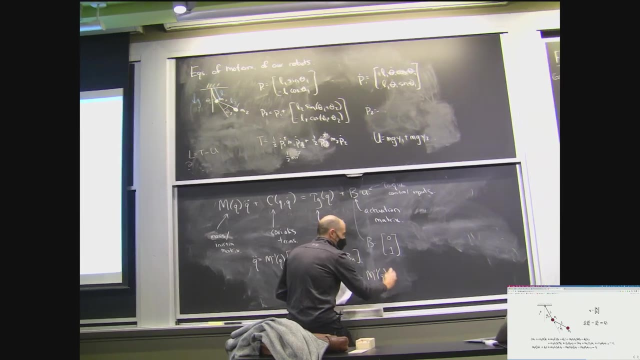 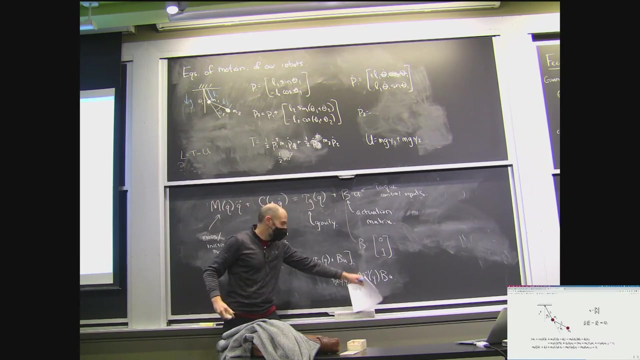 The matrix is always positive definite and you can take that inverse OK. So because of that, my f2 from my original equation right was the equivalent of f2 is m inverse q, b. OK, Because I know that m inverse is full row rank again. 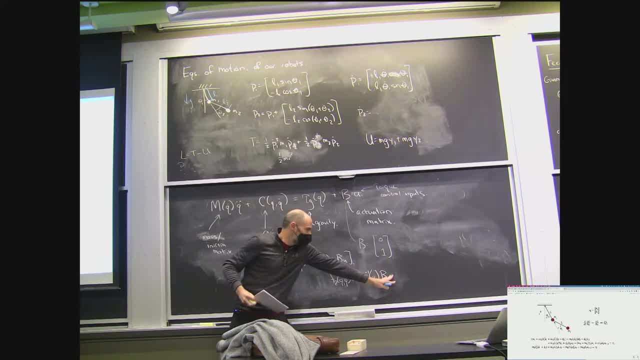 then the conditions of that whole thing being full row rank are exactly that: the matrix B has to be full row rank. So you're exactly right: If B is full row rank, then the system is fully actuated, And if it's not, it's underactuated. 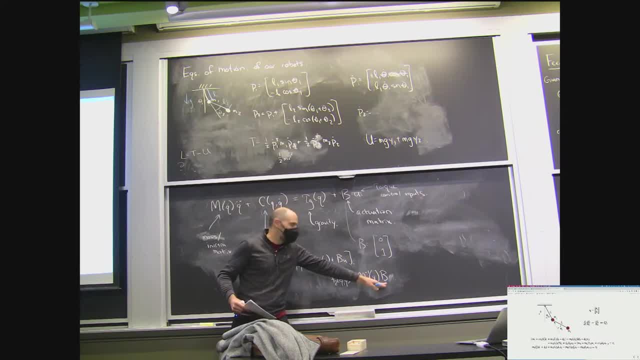 Now a walking robot turns out to not be full row rank because it takes. you know, it doesn't matter how many actuators you have. There's a Manoli Kellis. I don't know if anybody knows Manoli Kellis. 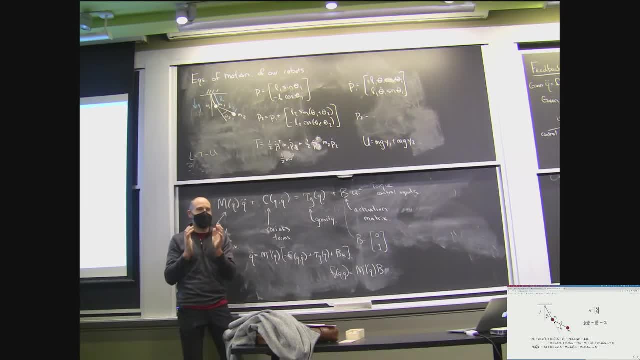 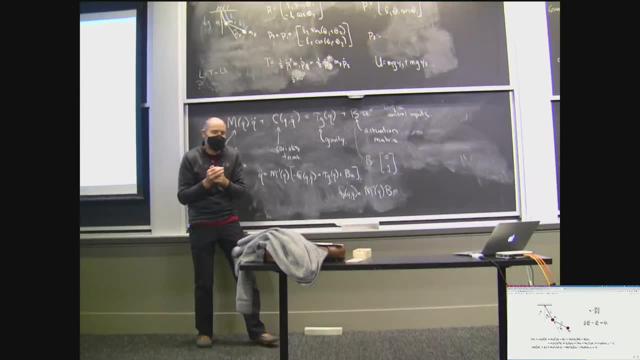 He's another professor in the department And he asked me one day in a faculty meeting. he says, Russ, if you had more research funding, would you work on fully actuated robots? You know, it doesn't matter how much research funding you have. 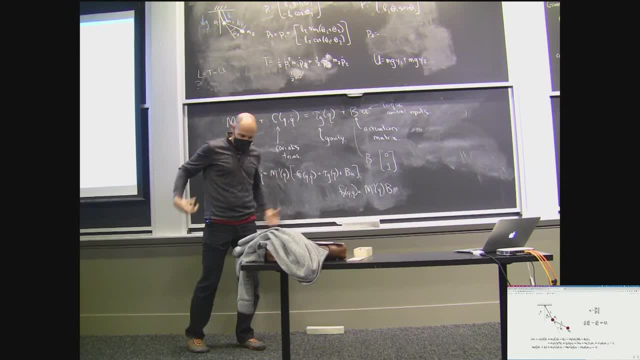 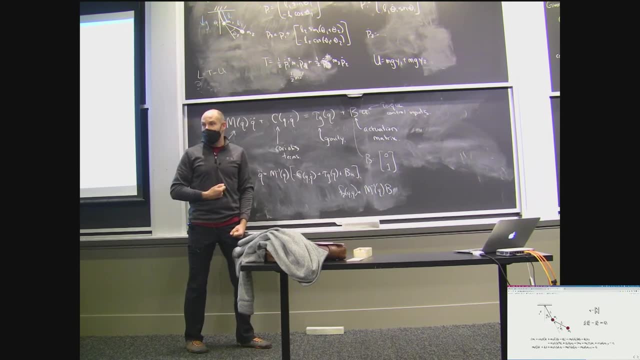 If you have a walking robot and you want it to move around, you can put as many links you know- motors as you want on your robot, But there's still some degrees of freedom. let's say your center of mass that is not directly actuated. 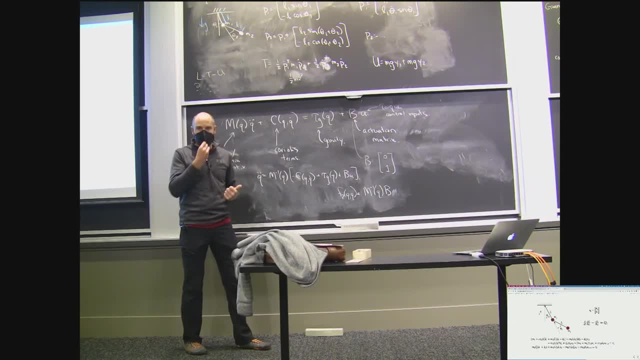 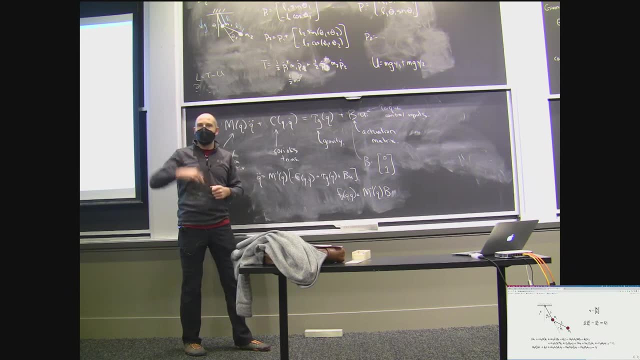 and you can't control it. So Atlas, no matter how powerful it is, cannot fall down through the sky faster than gravity. There's no control when it's jumping through the air that would allow it to accelerate itself towards the ground faster than gravity, unless it had a jet pack, which 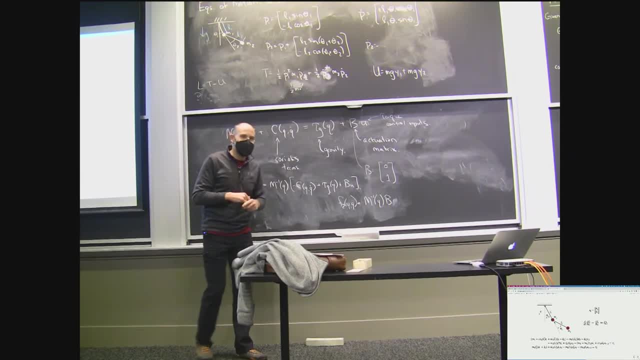 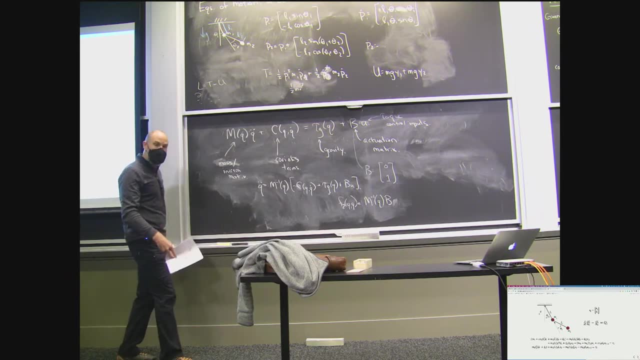 maybe next year it will, Who knows right, OK, So walking is fundamentally under-actuated, Unless you're in this regime. if you were to assume your foot was bolted to the ground and model your robot as being able to apply arbitrary forces, 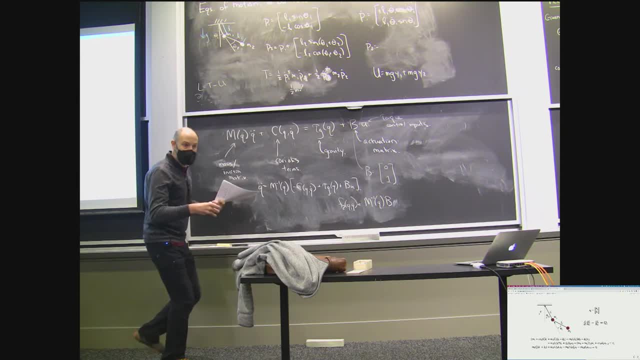 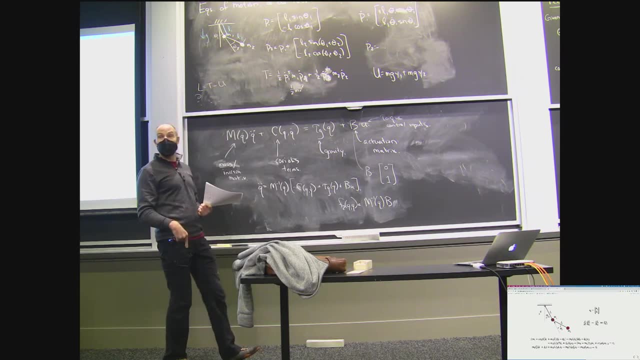 as if your foot was attached to the ground. then you can think of yourself as fully actuated. And that's what the early walking robots did. They roughly stayed in a regime where the assumption was good that the foot could be bolted to the ground. 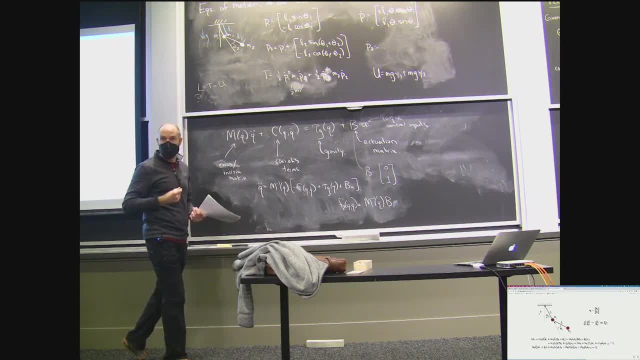 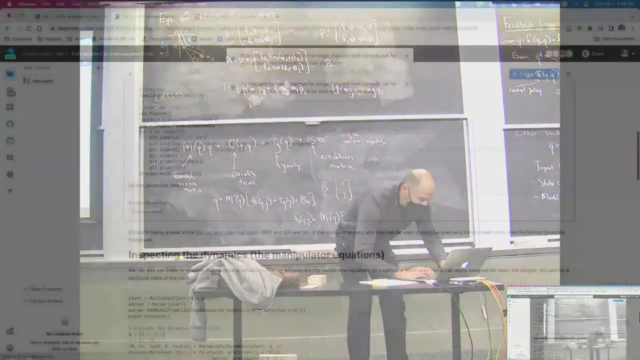 and then used all the tools from fully actuated robotics, And it's only a matter of time. It's only as we've developed this machinery for thinking about longer-term dynamics, using optimization as a tool, can we do more. OK, let's see if my demo is ready to go here. 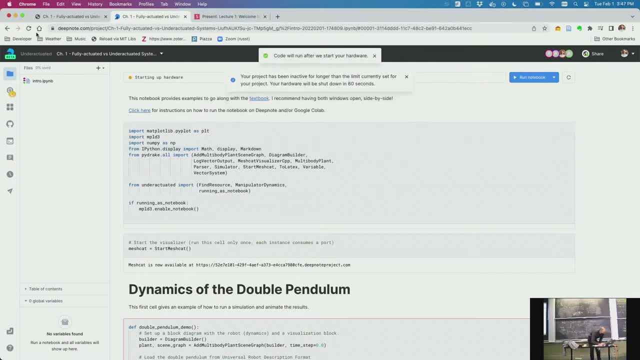 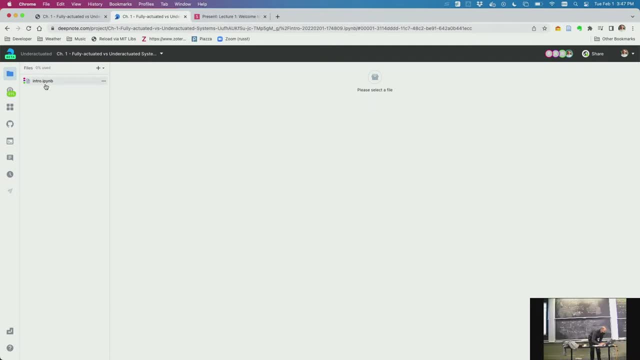 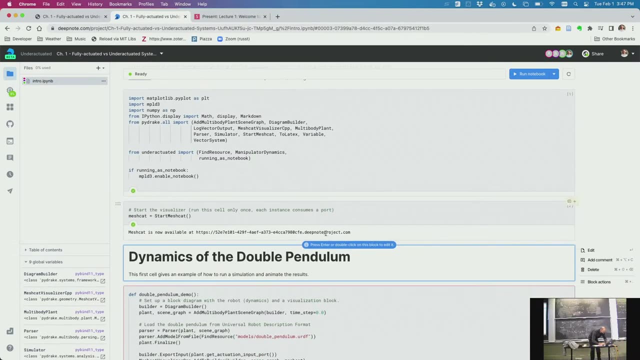 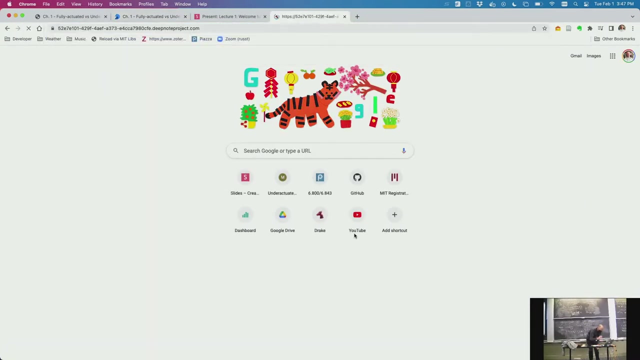 Did it really shut down again? Not my day. It says ready, Let's see. All right, This is. some of you who took manipulation, for instance, have seen this before. This is the setup we'll use for class. I've switched everything to Deep Note here. 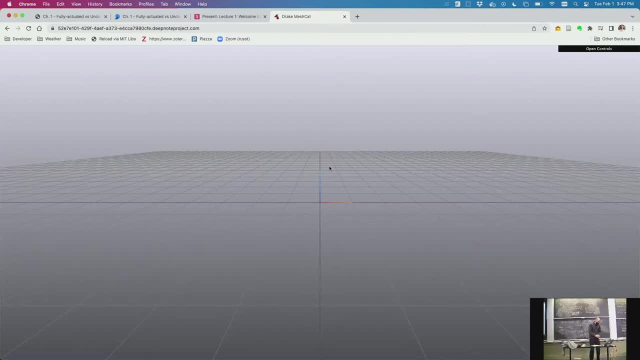 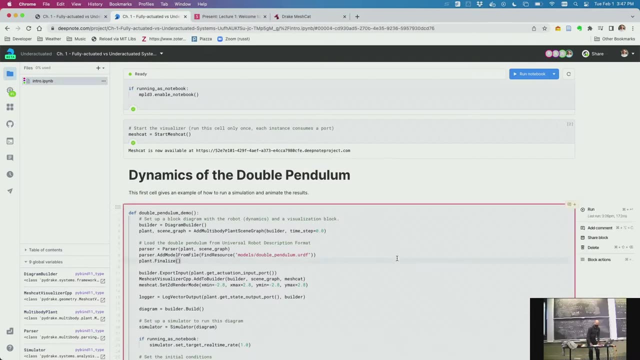 OK, we have the online visualizer. that will work in your browser And you shouldn't have to install anything. OK, let me show you a quick demo that tries to make this point. So I'll write the equations of motion of the double pendulum. 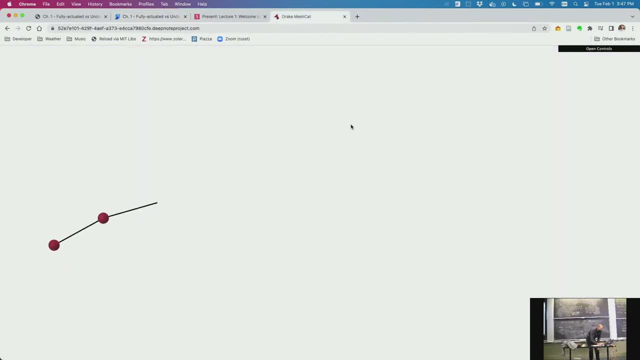 And the first thing in this cell is just to simulate it. It'll just simulate the double pendulum. That's a 3D renderer that's not being put to good use in this particular simple example, But you can see it's got lighting on the point masses. 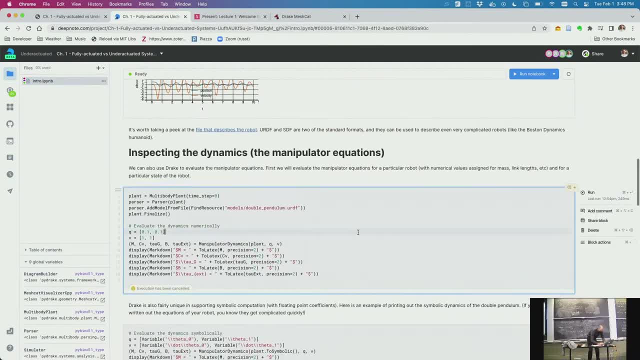 OK, and the software for the class. it's called Drake. It's actually a very. it was built for this kind of reasoning, So it has a symbolic engine underneath it, So you can not only simulate things, but you can also. 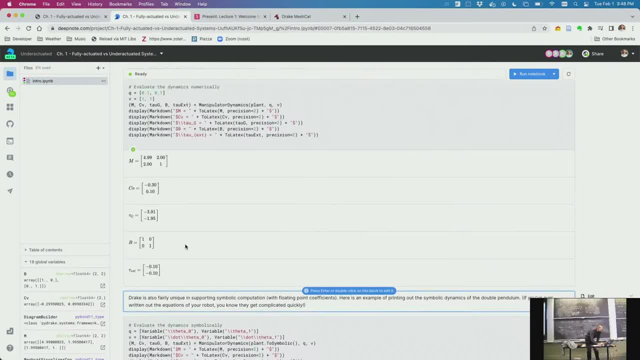 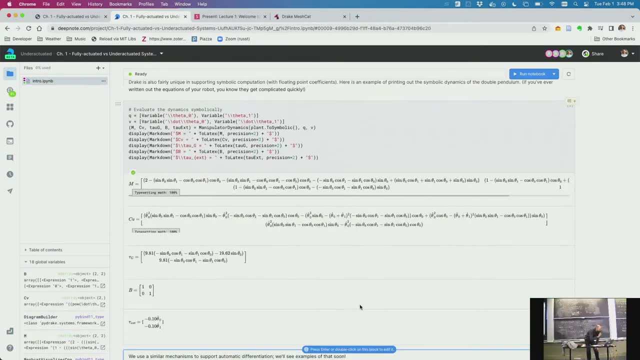 you can also just ask for the equations of motion. It'll produce them numerically, It'll produce them symbolically. So you don't have to do any Lagrangians yourself. You can just say: load up a double pendulum, And if you want to make your own robot, 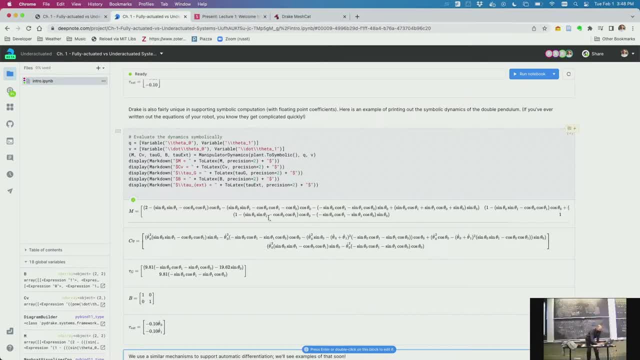 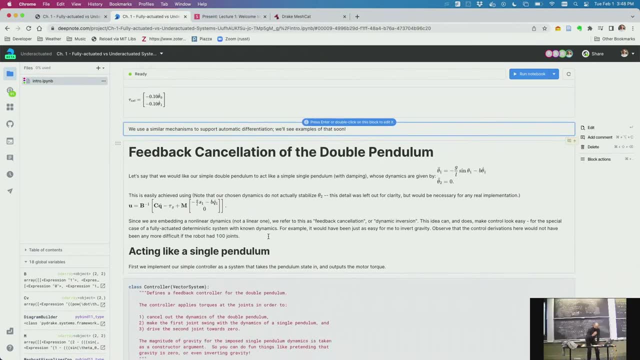 you can say: you can produce one of the standard robot formats And it'll produce all of the equations of motion for you. Now here's a simple example. I want to do So. my claim is that if your system is fully actuated, 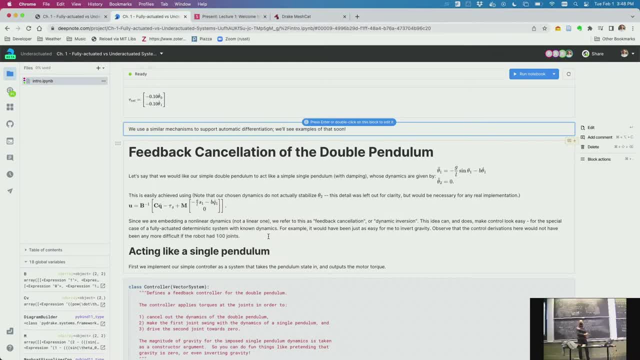 so if I put an actuator in both links, then I can make that robot do anything I want. It's not even like a fun control problem anymore, right, So to make that point, I can make this system. I can erase the dynamics of the simple pendulum. 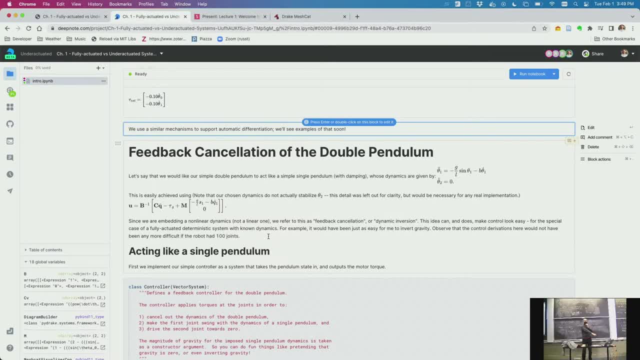 and replace it with the dynamics of a one-dimensional pendulum, I'll make the robot pretend it's a different robot. OK, So I just made a version of this that was actually a simple one. It's acting like a simple single pendulum. 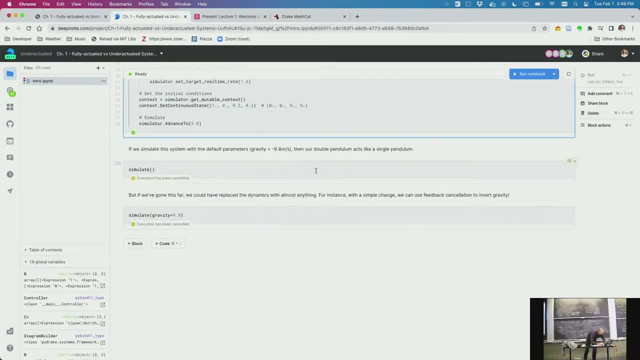 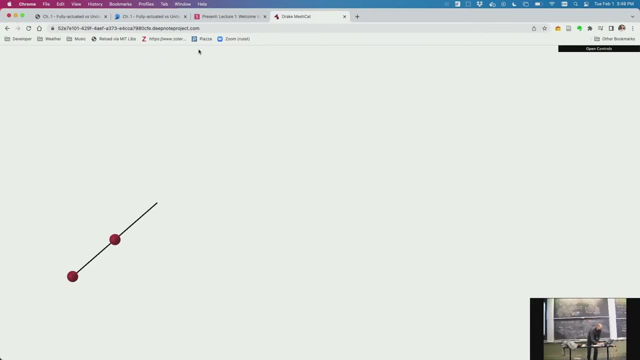 And I have to simulate it. OK, yeah, So there it goes As far as the. this is the same dynamics of the robot, but a different controller that is subtracting out the terms I know exist in the dynamics and replacing them with this sort of feedback cancellation. 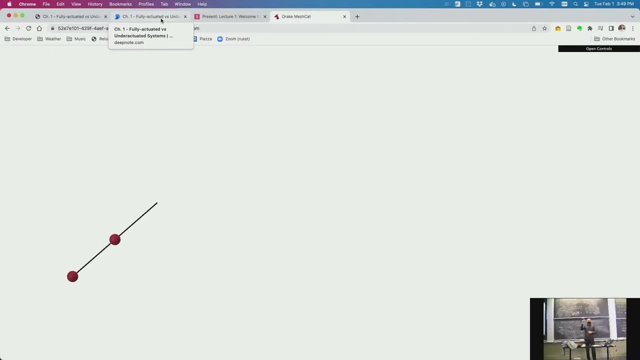 and just writing in the dynamics of a pendulum instead, so that when I simulate the whole thing through it, it's as if I had a single pendulum. OK, And it doesn't even matter, like I could make it do any. 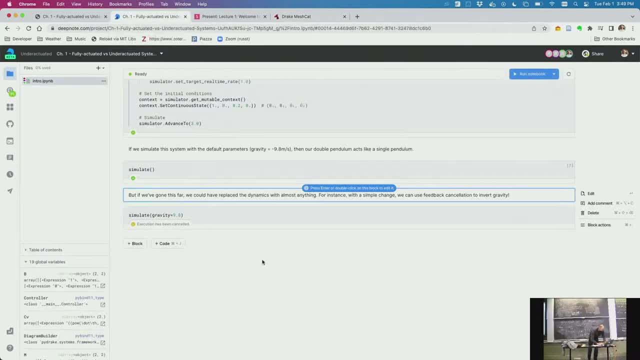 I could say: gravity is upside down. So that's what my second thing is here, right? So let's just say: I want to do exactly the same thing, but pretend I'm. you know, the gravity is upside down. It's an identical set of equations, right? 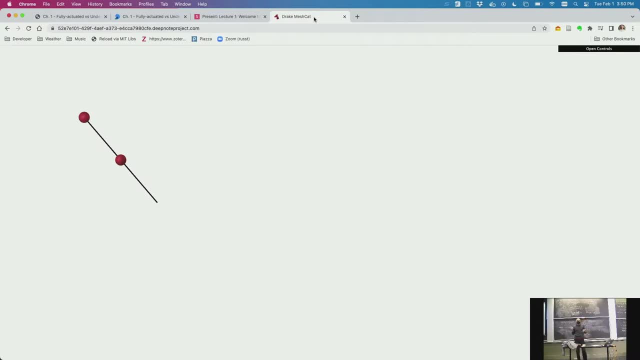 And it produces interesting torques that makes the system act as if it's upside down. OK, And if you're a robot that's bolted to the ground, has a full rank B matrix and has arbitrary control authority, then you can do that. 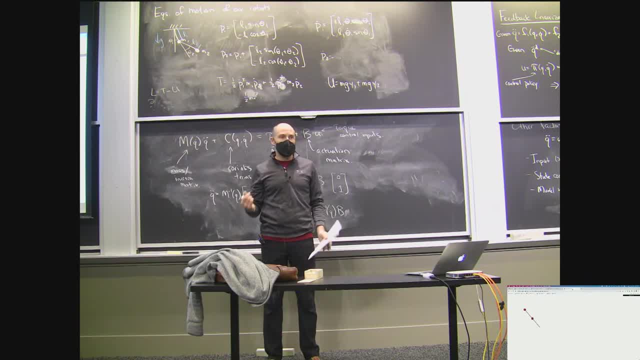 And you can, and the problem of control is not significant. OK, But when B you know this criteria is the simplest thing to point to, to say: control just got hard. You now you can't just erase your equations of motion. 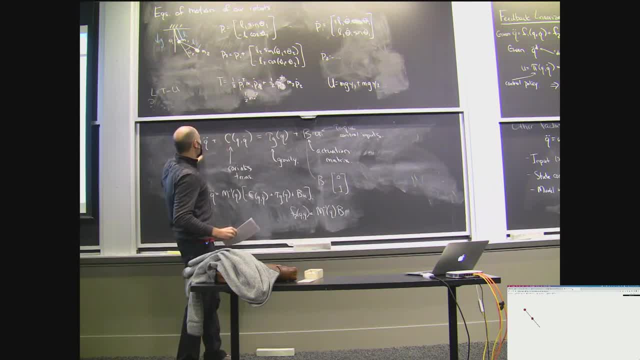 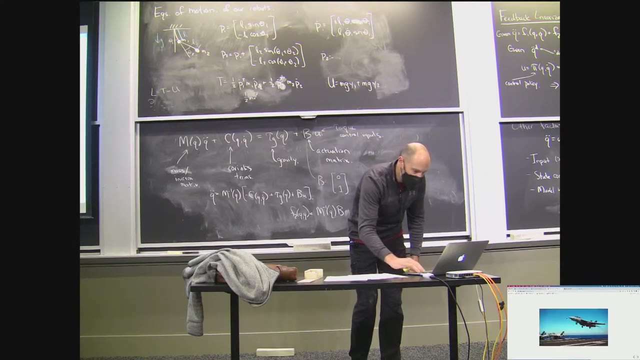 You have to go, you have to dig in, You have to understand what's going on Again, you have to understand what's happening here. You have to make long-term control decisions in order to do excellent control. OK, It's true. let me just, you know, say it's true for quadrotors too. 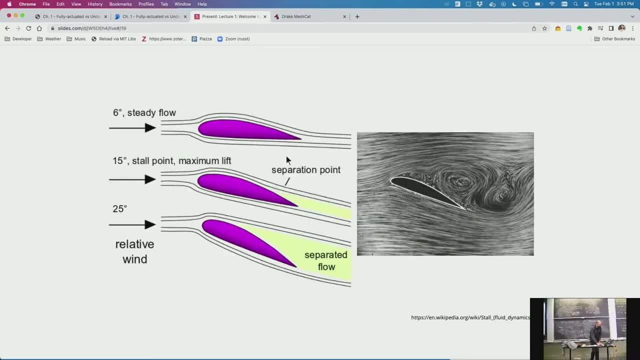 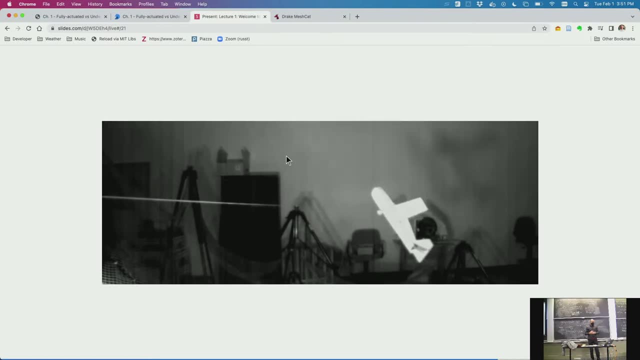 I'll give you a longer version of this later. but we have, like, airplanes landing on perches and stuff like this. You know some early work we did of trying to do, you know, very aggressive maneuvers with flying robots, you know. 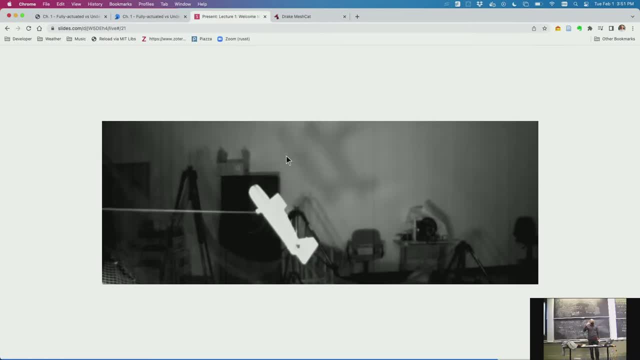 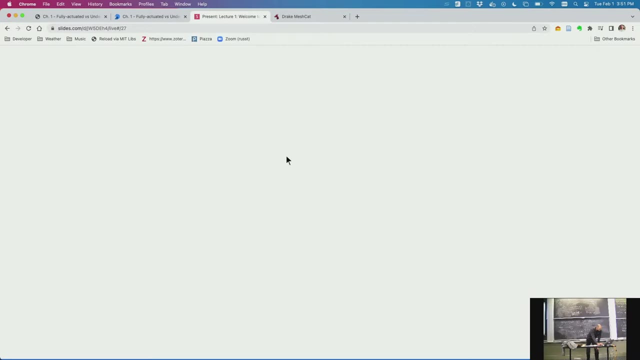 weren't possible until we started thinking about had stronger optimization tools to power through the nonlinear dynamics of post-stall aerodynamics. But now we can make airplanes land on a perch. We can do all kinds of fun stuff, Oh, all kinds of fun videos that I was going to show. 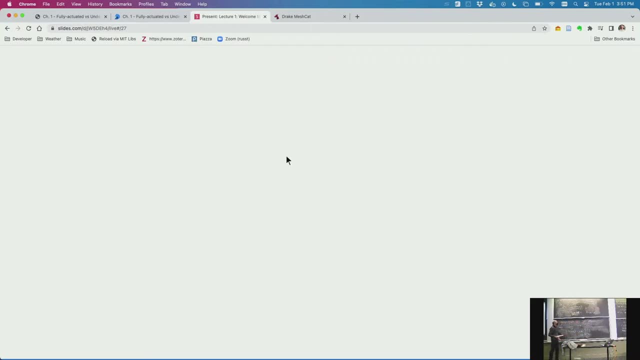 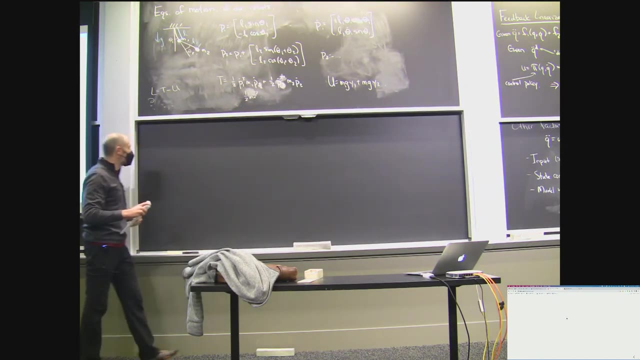 All right, So let me tell you roughly what the plan is for the course. We're going to talk about nonlinear dynamics. right, We're going to start off. We're going to make sure people understand the basic tools of nonlinear dynamics, of stability, of basins of attraction. 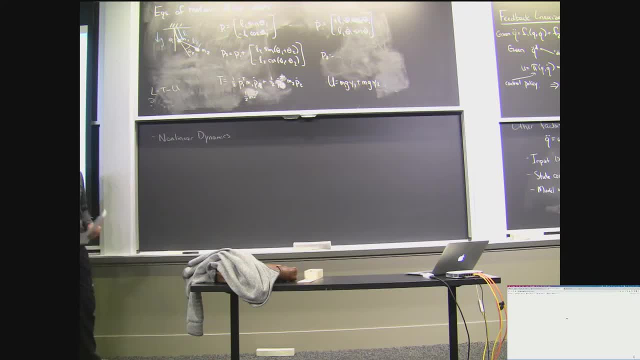 of you know, of Poincaré maps, all these kind of things. OK, We're going to talk a lot about optimization and optimal control. We'll talk about both control theory approaches to that and machine learning approaches. OK, And yeah, I think the whole thing should hopefully come up. 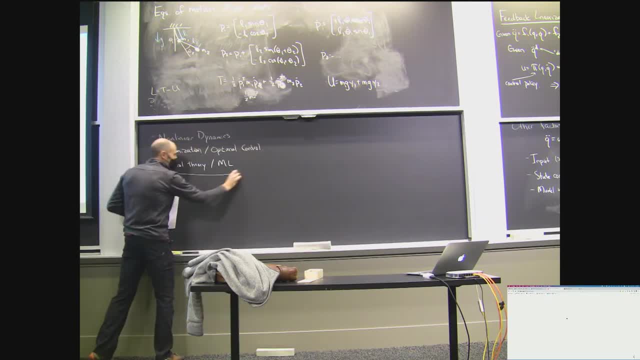 and blend nicely together. The way that I like to structure it is by doing sort of really simple things, Rigorous, thinking about simple model systems, OK, And we'll also give you sort of a big toolbox for your complicated robots, OK. So, double pendulum, we'll have very simple versions. 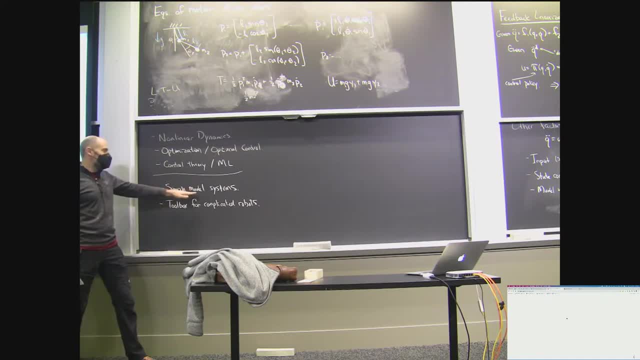 of walking robots. We can, like, write the equations down, We can understand them, We can understand what an optimal controller would look like for them. OK, And that's what's going to teach us the fundamentals. OK, And give us you know, just even understand what we're going. 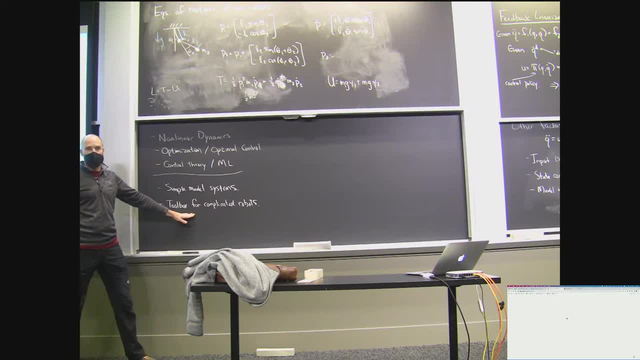 to see, And then we're going to try to give you algorithms that are going to work for the big, complicated systems too, like Atlas doing a backflip. OK, So I organized the class, sort of starting off with, you know, very simple models. 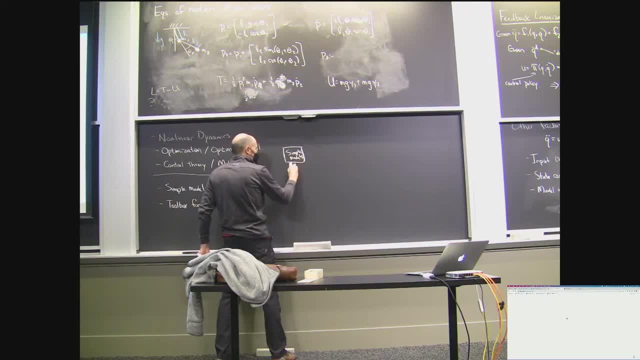 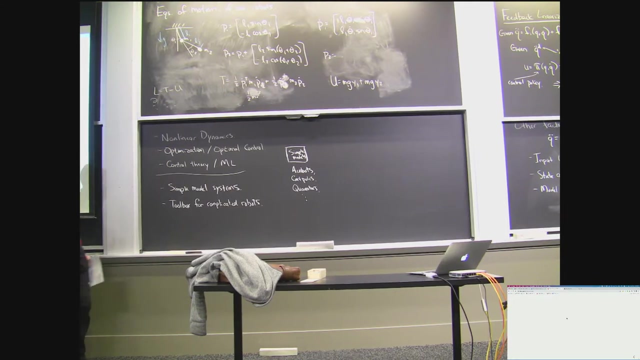 OK, We get like acrobats, cart poles, the basic quadrotor models, et cetera, And given that set of models, there's already just a huge set of powerful tools from optimal control, from optimization, from machine learning that we can throw at that set of models. 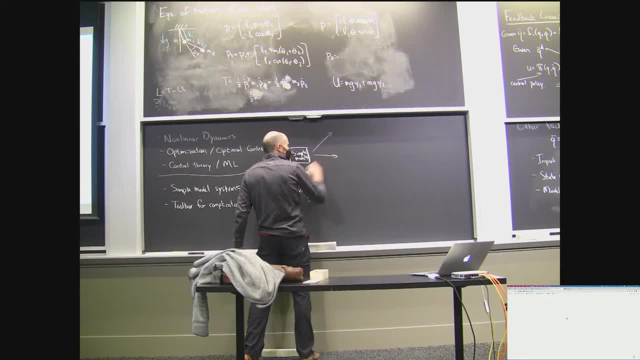 And then we're going to start making things harder in interesting ways. OK, So when the environments get really complicated, so you might have to do more complicated motion planning alongside these. You have to work in a very cluttered environment but still be very dynamic. 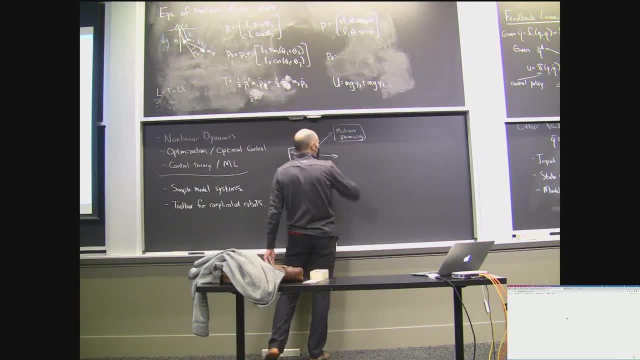 There's a whole bunch of interesting algorithmic challenges that that brings up. We're going to do walking robots. OK, These are my simple models of walking robots. that goes like this: Introduce limit cycles, Think about long-term periodic stability And control through contact. 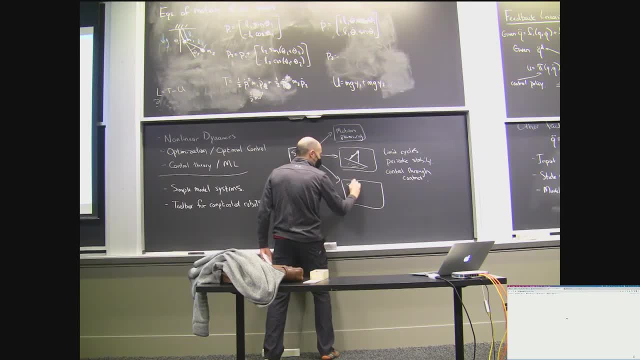 And then we're going to talk about stochastic systems, And we'll talk about stochastic and robust optimal control And I'll sprinkle in some system identification ideas, some model-free control ideas throughout. OK, But roughly, we're going to start simple. 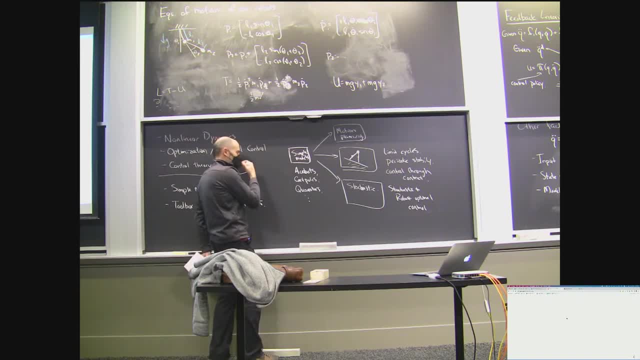 We're going to form a foundation. We're going to understand optimizing and non-optimizing controls for these simple systems and how to analyze them rigorously, And then we're going to blow out in a couple different directions to try to build our toolbox for really complicated systems.